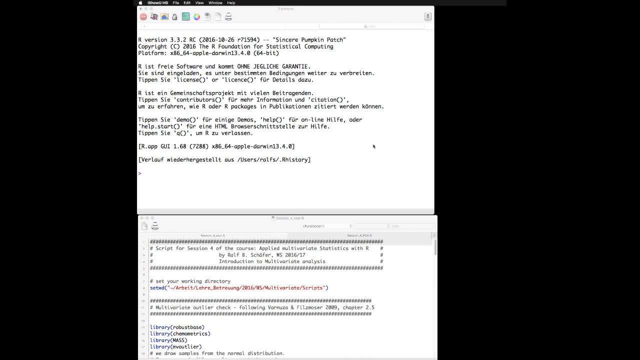 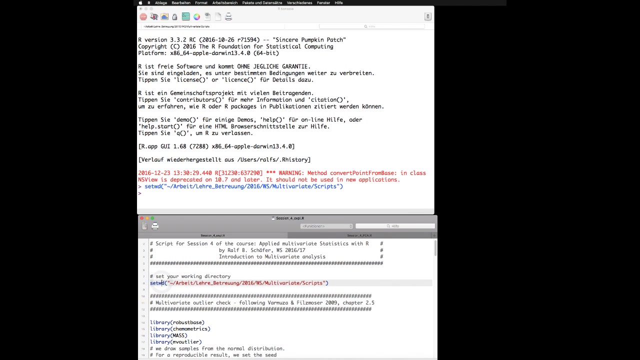 Welcome to the practical part of the multivariate analysis. This part. we deal with two scripts. The first script describes a couple of general analysis methods for multivariate case, like multivariate outlier checking, and the second script describes the principal component analysis. So you have the session four script explained, dot R, and a session four script for PCA. We start with the session four script for explanation of general diagnosis and analysis. First, as you know, you set your working directory. I can quickly jump over that. You're used to that now- And then we load a couple of libraries that we will need for multivariate. 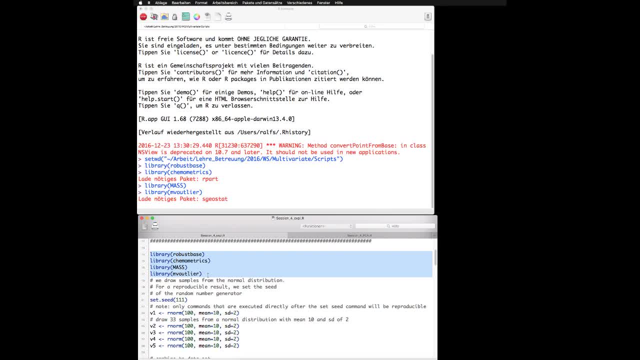 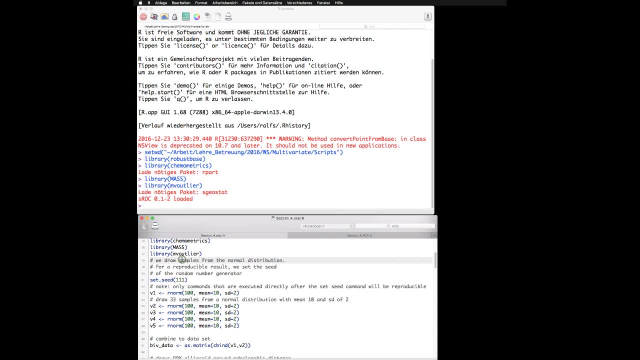 analysis. But we first do as what you have seen on the slides: We draw samples from the normal distribution, We set the seed. That means that the random samples that are taken here, So the function R norm, samples 100 values with a mean of 10 and a standard deviation of two from the normal distribution. And we do this five times. 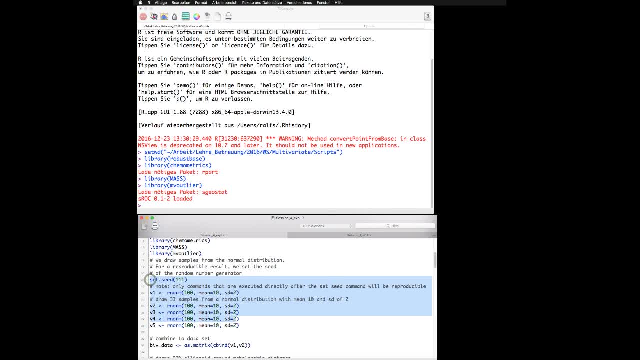 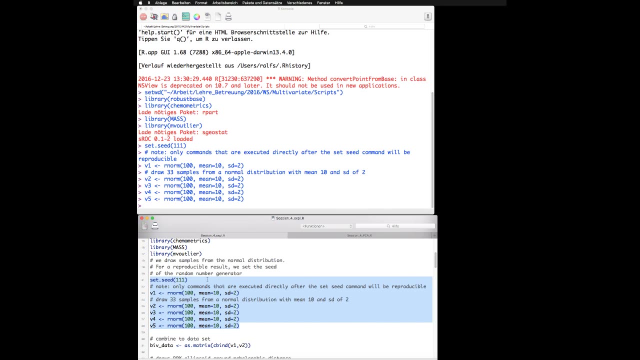 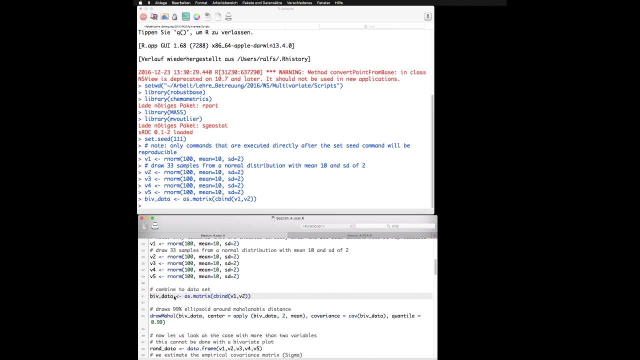 So we create five random variables and to execute this report in a reproducible manner, so that everybody who executes this function obtains the same result of the random number generator, We use the set seed function. Then we combine these different variables into one data set And what you've seen on the slides- 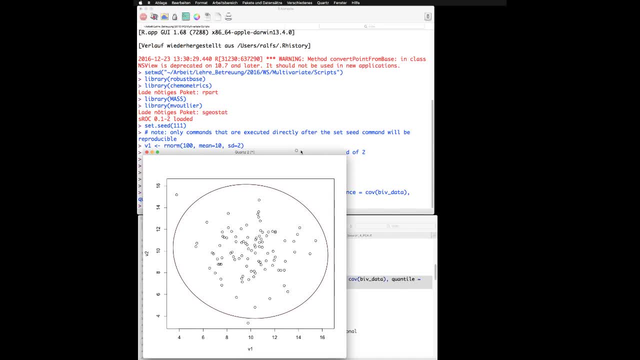 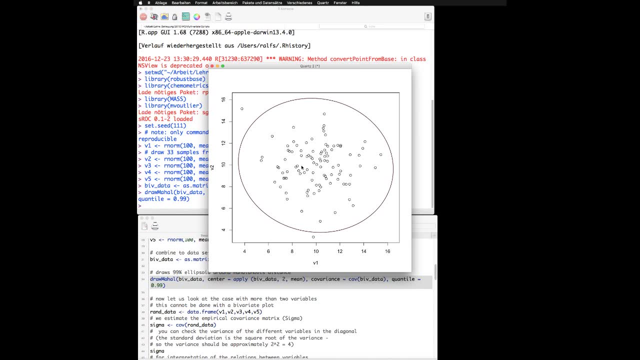 We draw the ellipsoid around the malanobis distance. So you see, here these are the different data points that we have for just two variables that we have created, And one of the points would lie outside of the malanobis distance. In fact, two points: The point here below and this point here. 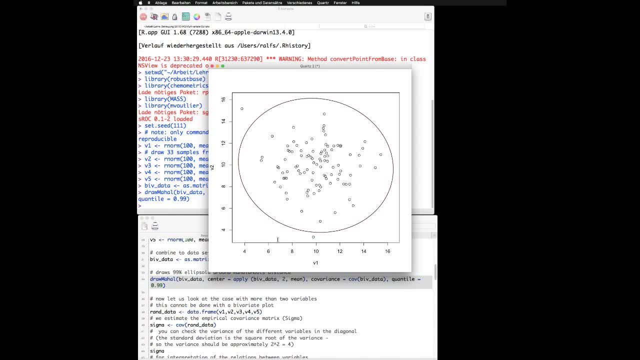 And we've discussed in the lecture already that the malanobis distance was more as drawn here- is more suitable to detect outliers, joined outliers, than any other individual variable. outlier checking method: Okay, for two variables, that straightforward, But we want to look for. 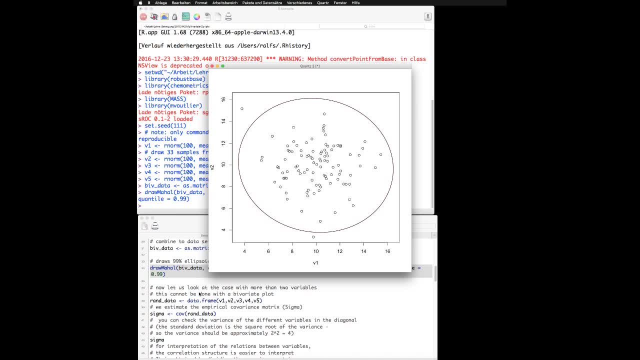 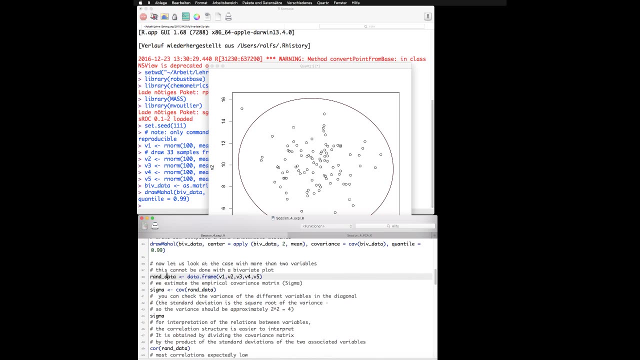 outliers that are related to the full data set, which is five variables here. so we can't plot these five variables in five dimensions. What we do now is we draw samples from the random normal distribution. To do this, first we create a data frame with random data and use this to estimate the empirical 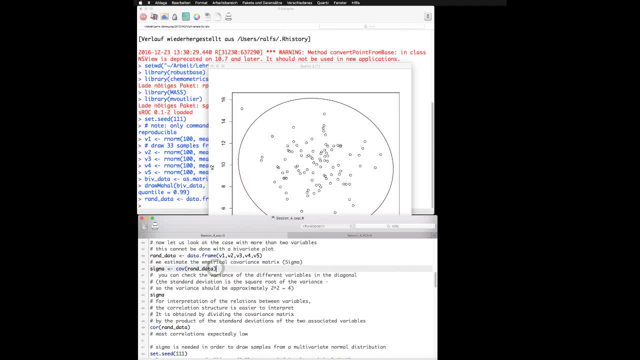 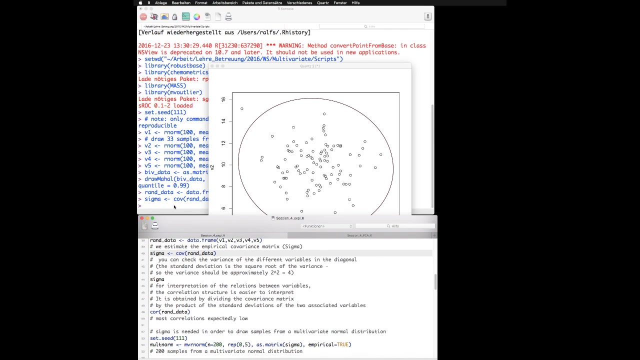 covariance matrix we have encountered. If we discuss the covariance matrix on the slides, that's basically the matrix that provides the co-variation between two variables and in the diagonal, the variance of the individual variables. Let's call sigma and we can check that the variance. 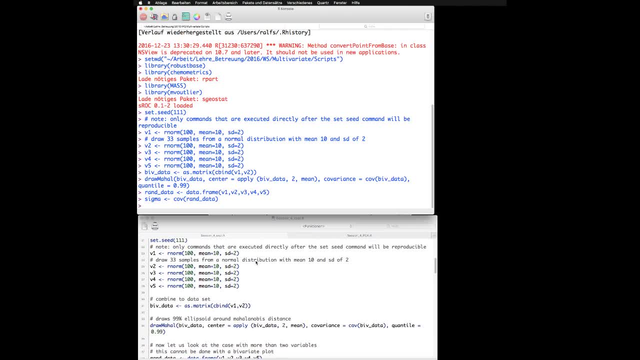 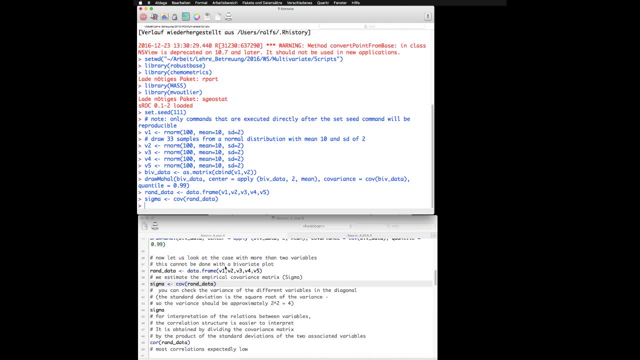 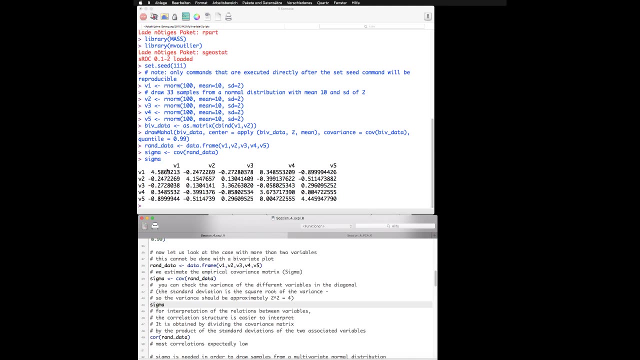 of the variable is equal to the variance of the variable. When you think back that we created here variables that have a standard deviation of 2, so we should have a variance of approximately 4.. If you look at these variables we see in the diagonal, we have approximately variance. 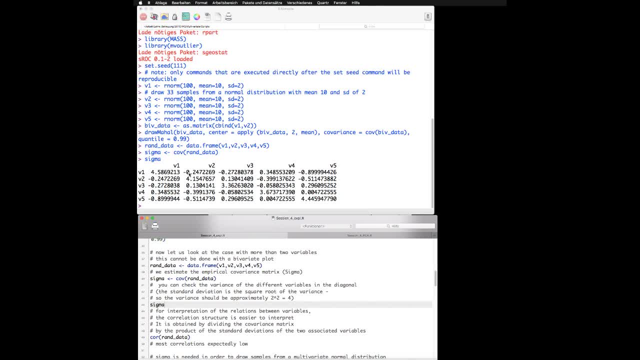 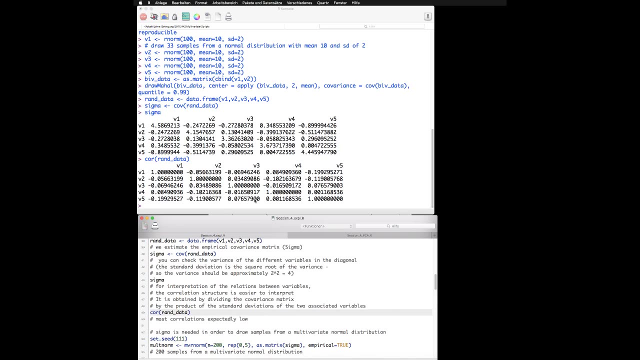 of 4.. Of course these are random variables, so that doesn't match exactly the value of 4.. Then we can calculate the correlations. We see that most correlations of these random variables are relatively low, and that's to be expected, because these are just. 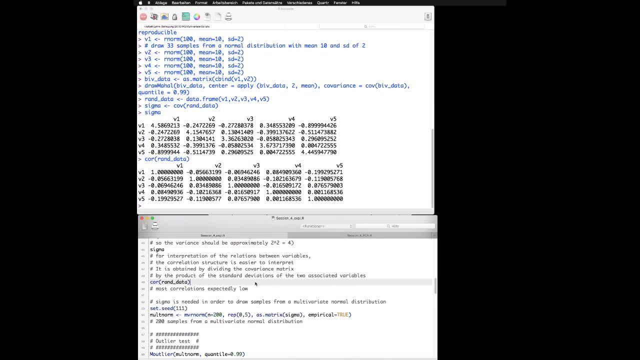 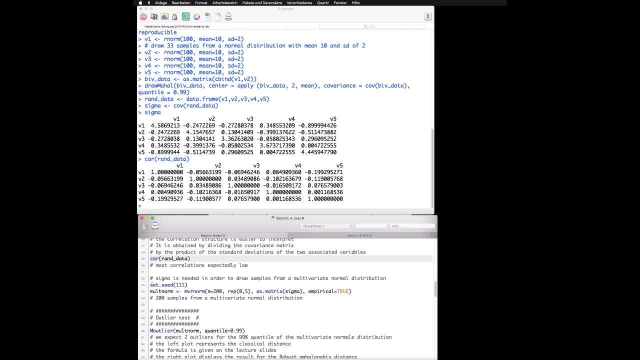 random variables that have been created. What we do now is we take, we draw a sample from the multivariate normal distribution using the function mv, our norm. That means it's the multivariate random normal distribution from which samples are taken. We take here 200 samples and we have, we have. we mean that we, that we 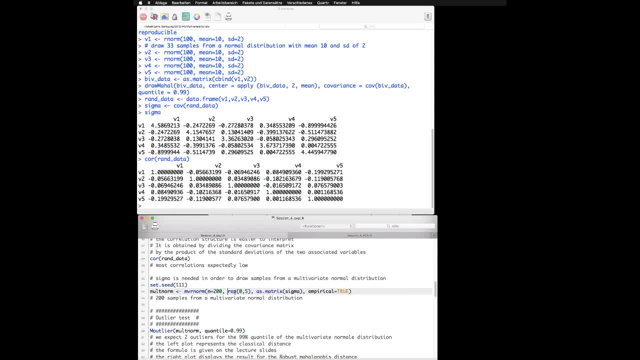 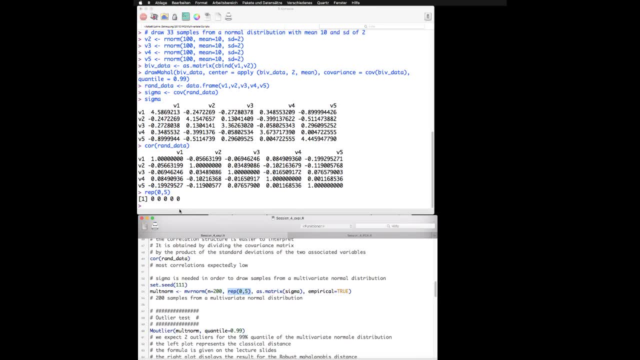 use here is: if you execute this, it's a mean vector, apparently. so let's see what happens. Since we have five dimensions, the overall mean is, in any dimension is 0.. We need to provide a covariance matrix to inform the function what correlation structure the data has, and we do this by providing the sigma. 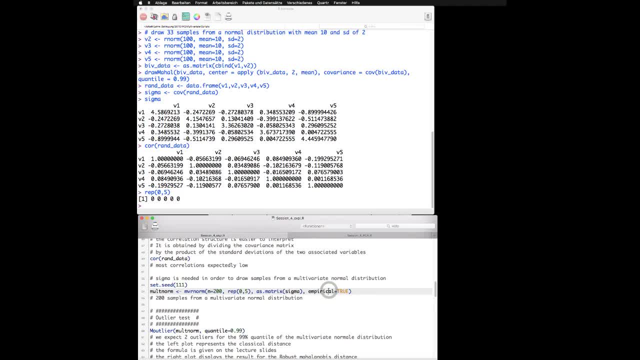 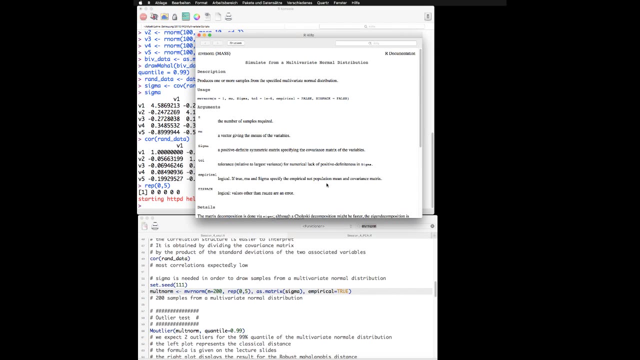 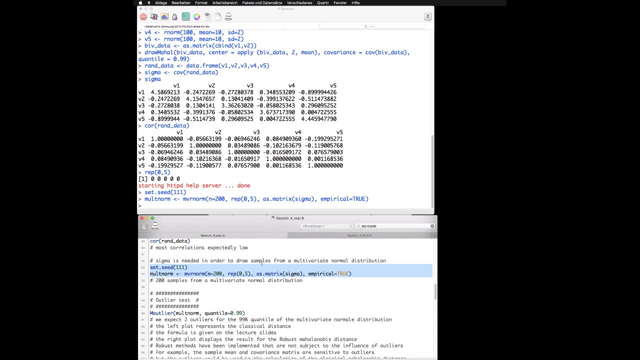 that we just created And empirical equals true, As always. you find that all information on the functions and the help files and you can see that empirical equals true is. that is the empirical covariance matrix. See a couple of more couple, more information here. Okay, so we draw the sample. 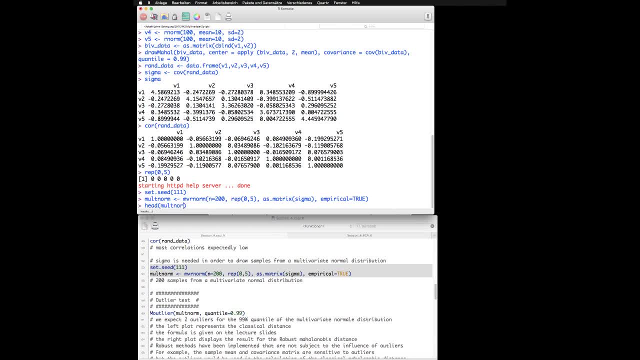 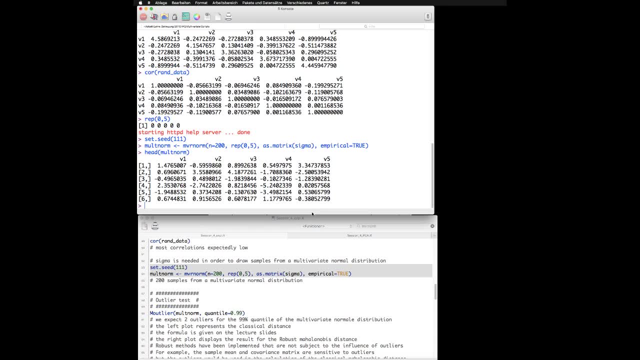 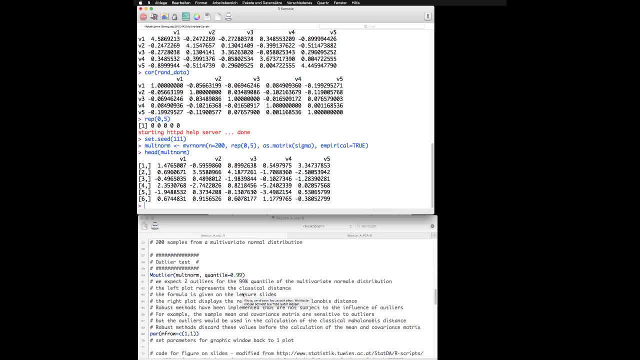 We have obtained now is a five variable data set with 200 rows. These are the individual samples that we just drew from the normal distribution, from the multivariate normal distribution. So to conduct an outlier test, now we can use the function moutlier, where we provide our multivariate object and define a 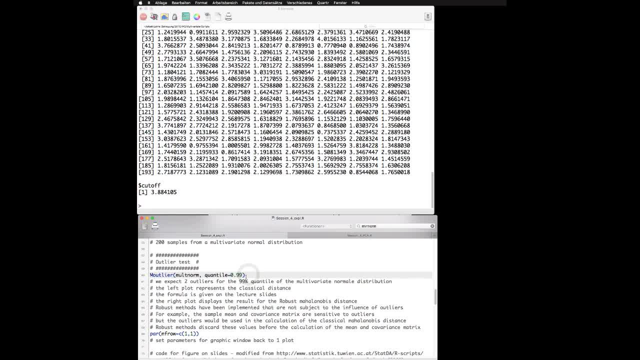 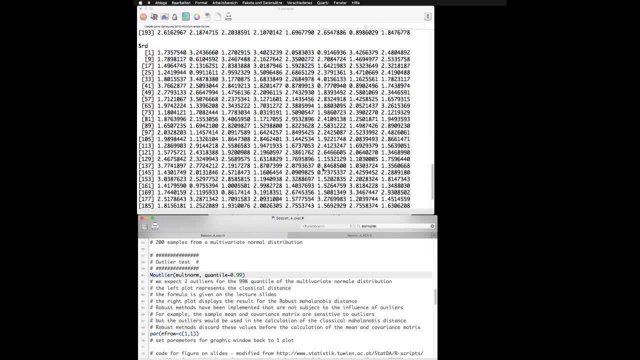 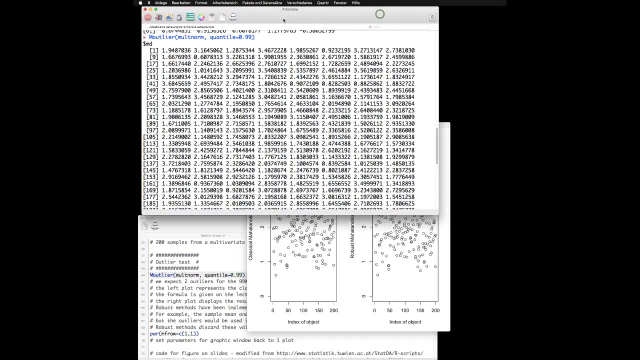 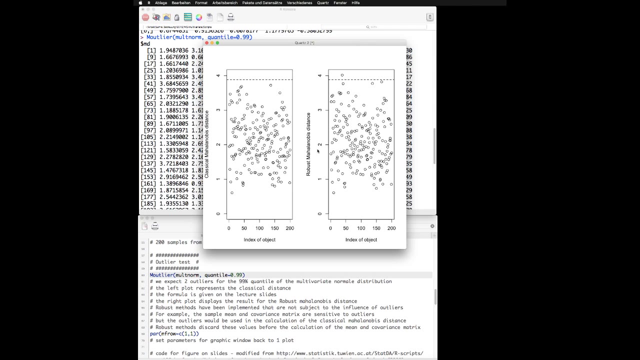 quantile For this outlier. we will use our multivariate object and define a quantile For this outlier checking, and you can see the individual values from this function that we obtained. The plot has disappeared here. We see here the classical malnourished distance that is calculating here a robust, malnourished. 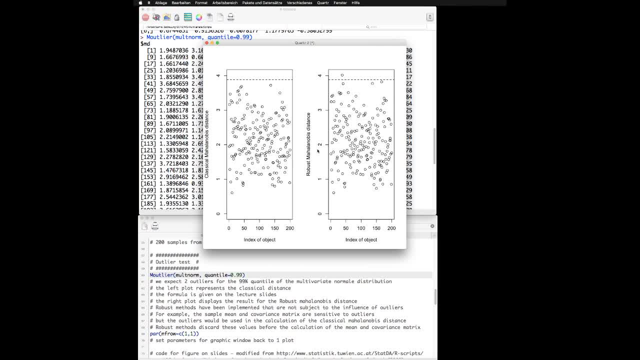 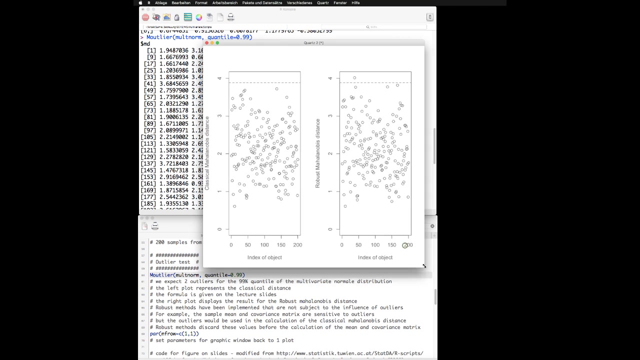 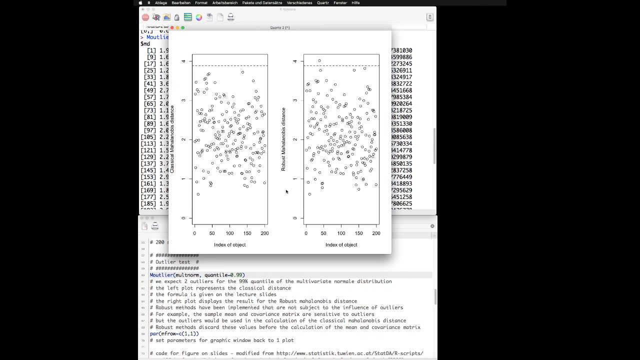 distance. Robust, malnourished distance means that not all not so. the outliers are basically not included in calculation of the modern novice distance because they would otherwise increase the distance itself or influence the distance itself to the sort of mean vector when you calculate this. so in 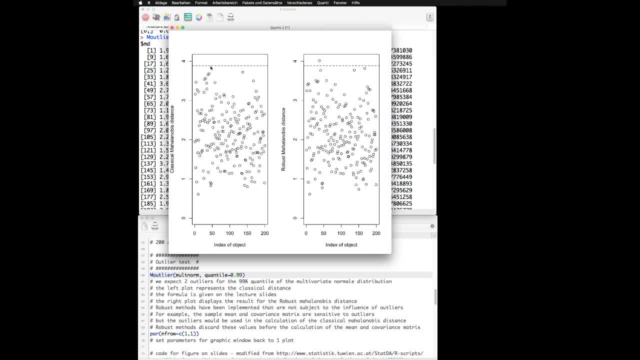 case of quantile here we have, we can define what we define as outliers. so could be 95% quantile or 99% quantile. in the case of the 99% quantile which we have defined here, we'll expect approximately two outliers. so we see. 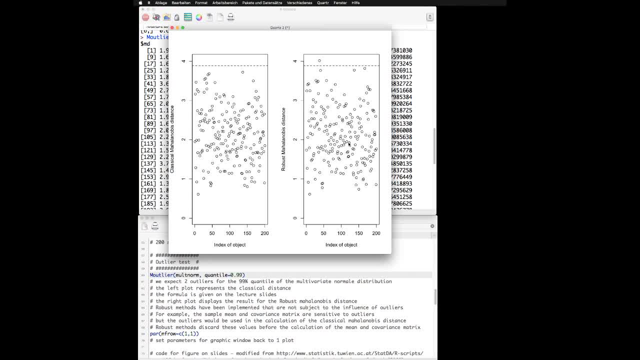 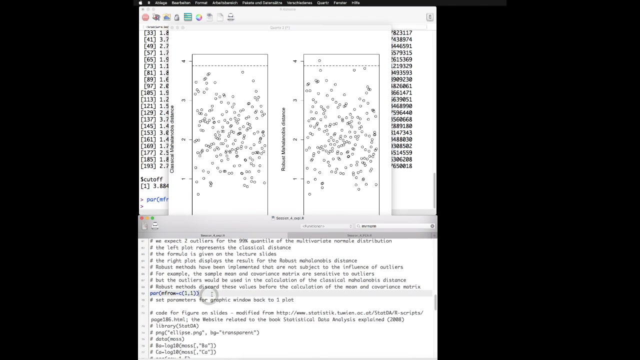 that we only have one outlier based on the robust my novice distance and it's actually relatively close to this threshold, given the threshold that we provide for the 99% quantile. so now we set back the parameters for the graphical window to having just one window. you have some. 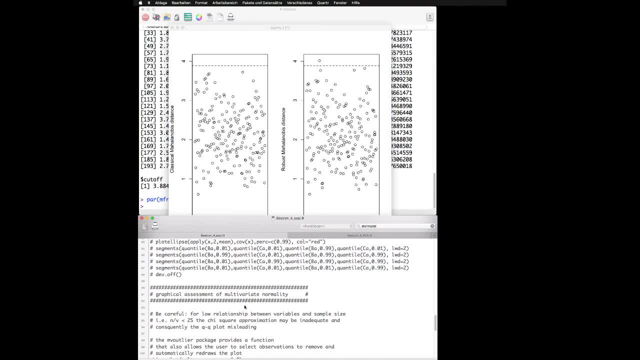 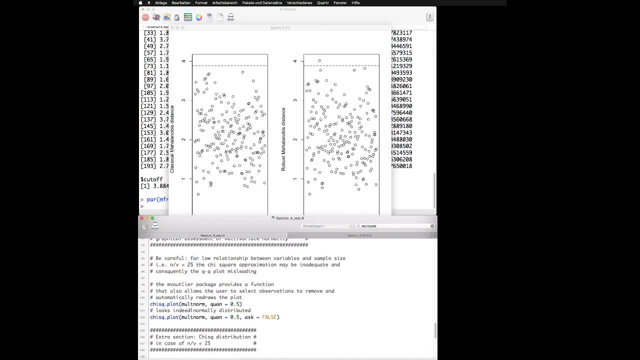 code to access to to reproduce this slides and we continue with the graphical assessment of multivariate normality. you have some code to access to to reproduce this slides and we continue with the graphical assessment of multivariate normality. you have some code to access to to reproduce this slides and we continue with the graphical assessment of multivariate normality. 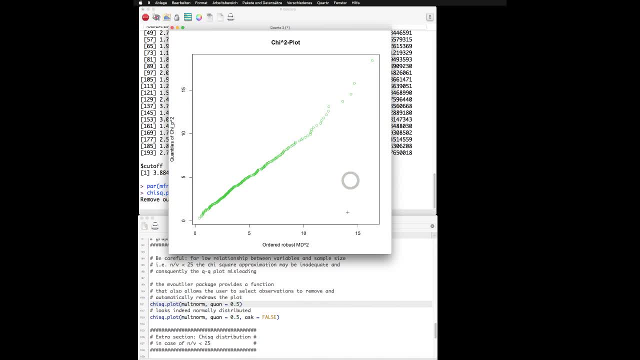 we do this and this is the plot that we obtain for the G square, G square distance. and you see that, not surprisingly, the data are fairly well, normally distributed, multivariate, normally distributed, so the quantiles and the orders- robust, my novice distances- match each other's quite well. 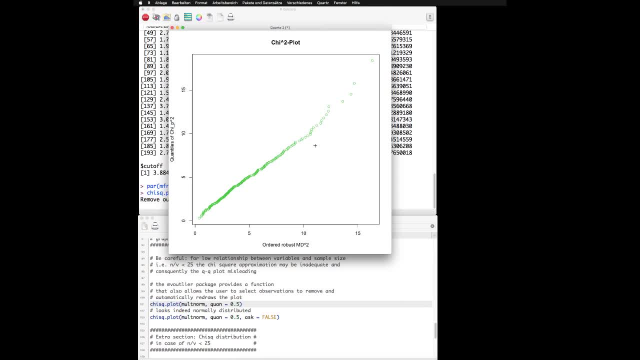 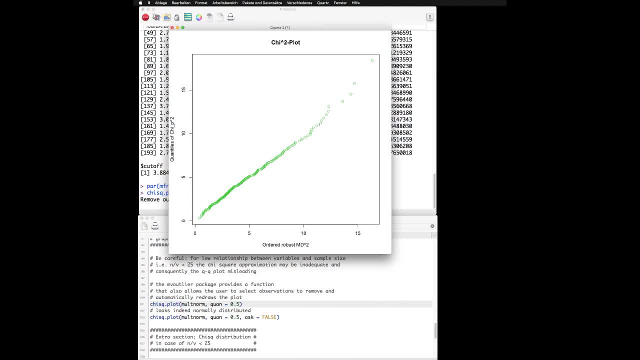 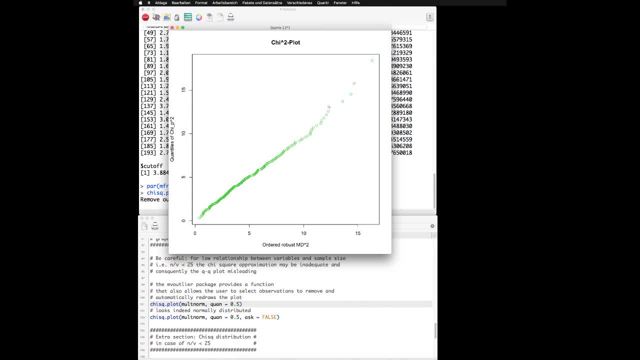 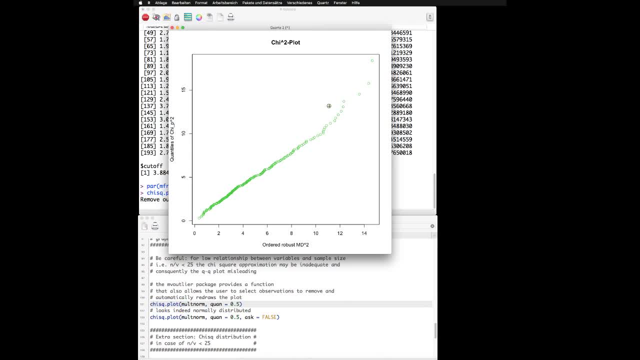 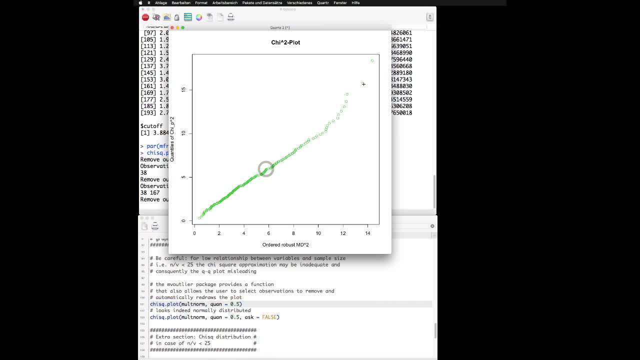 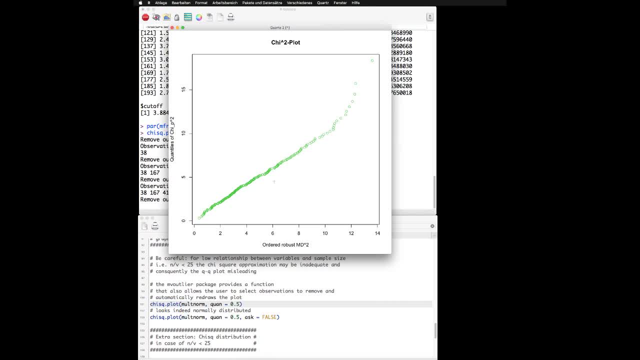 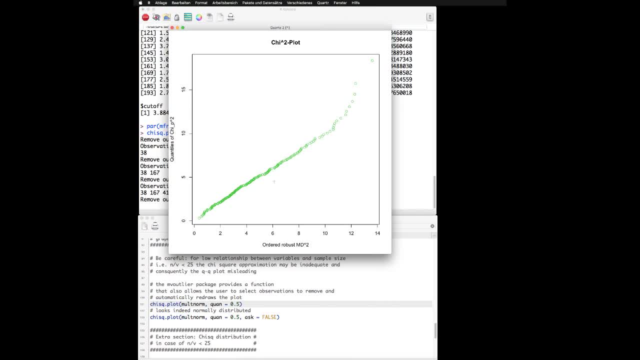 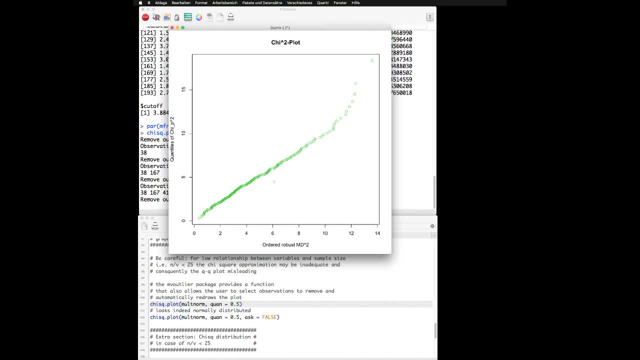 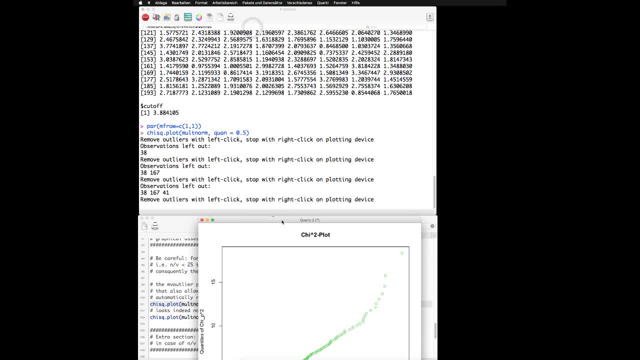 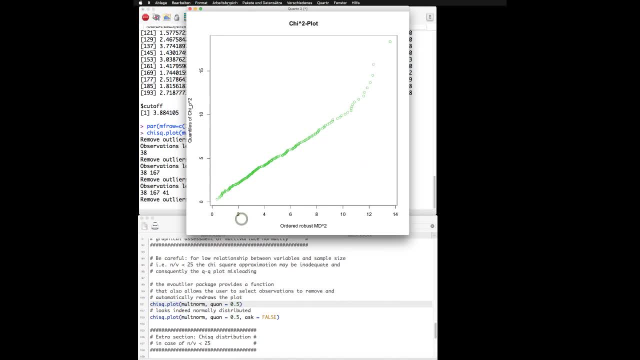 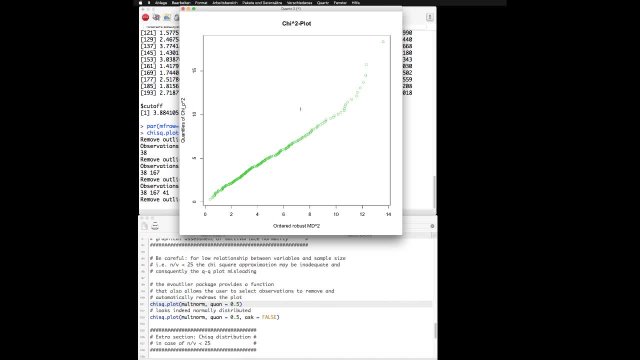 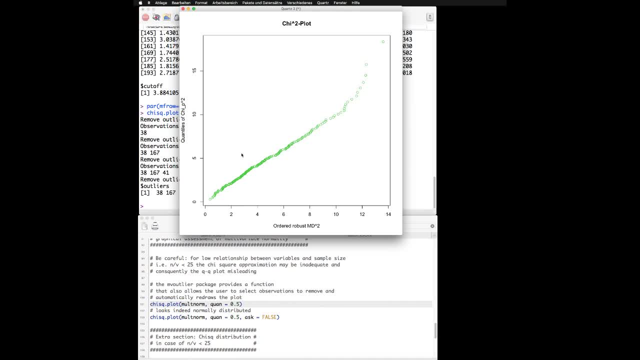 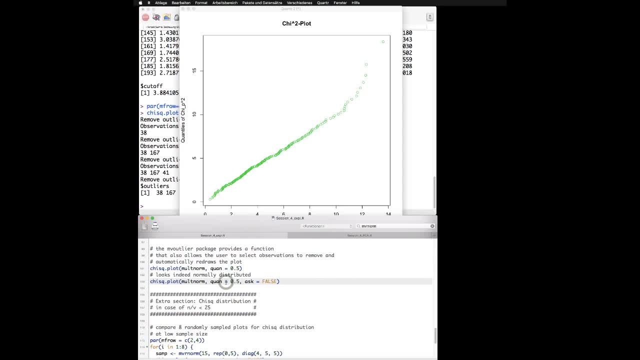 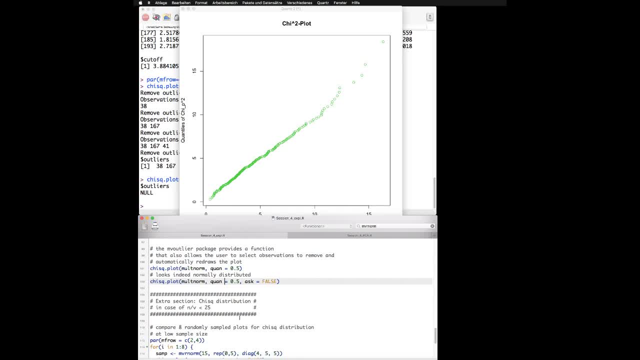 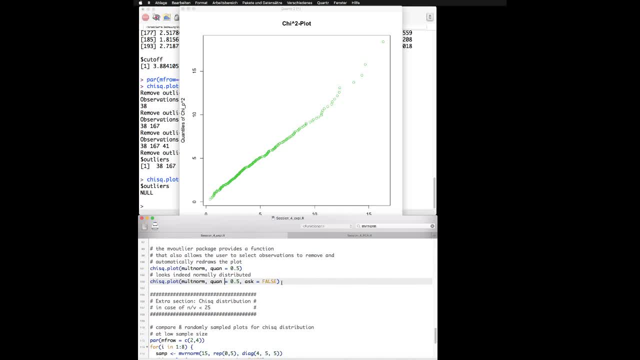 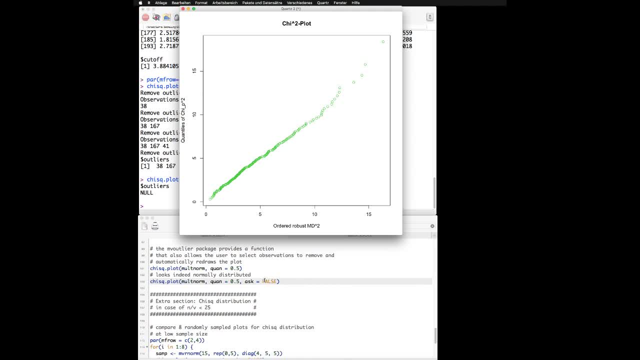 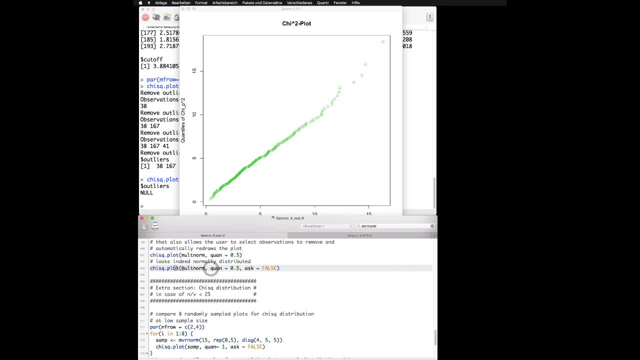 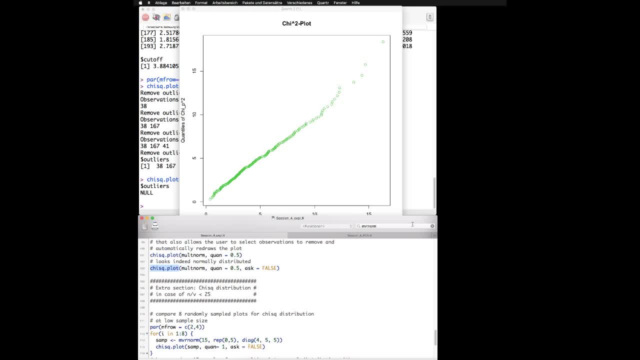 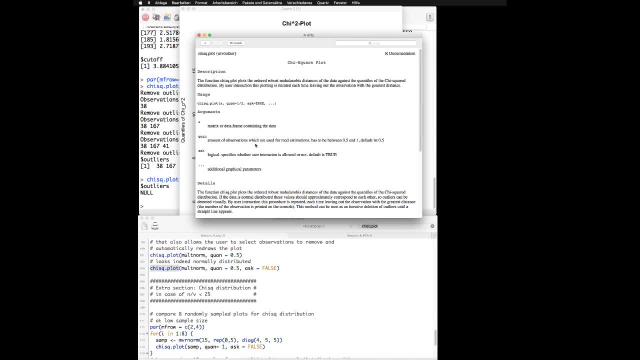 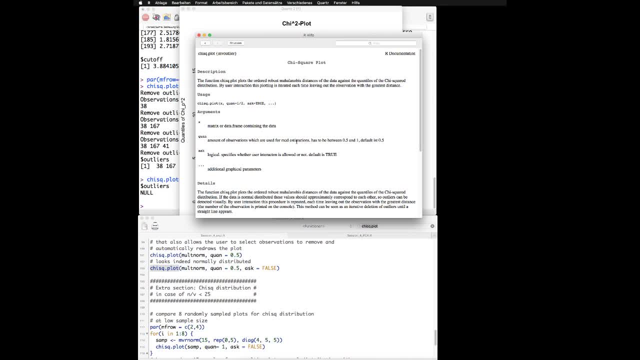 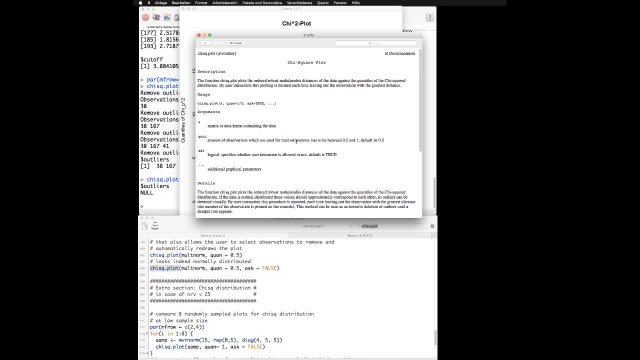 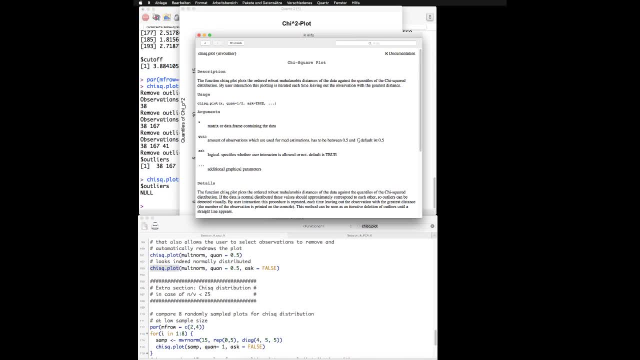 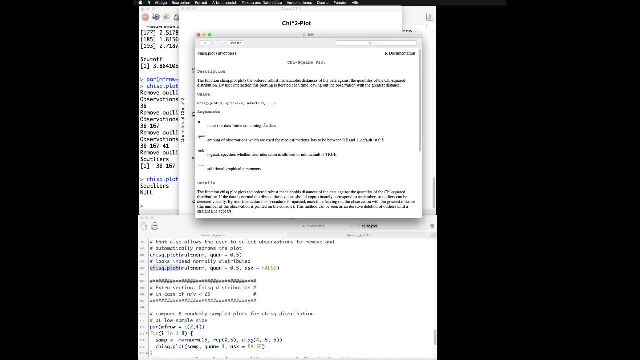 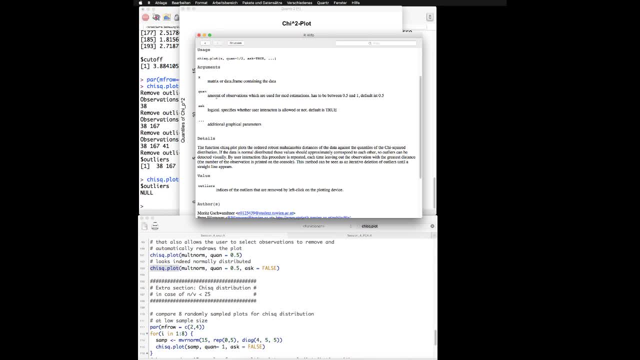 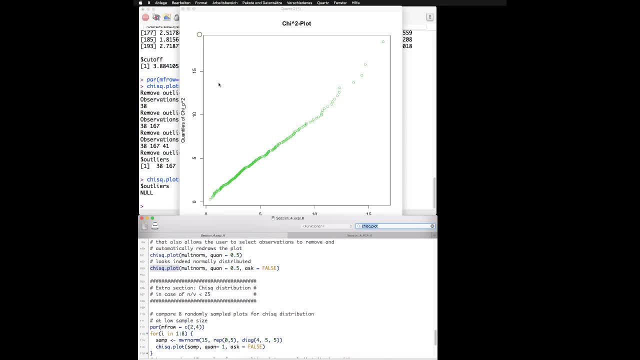 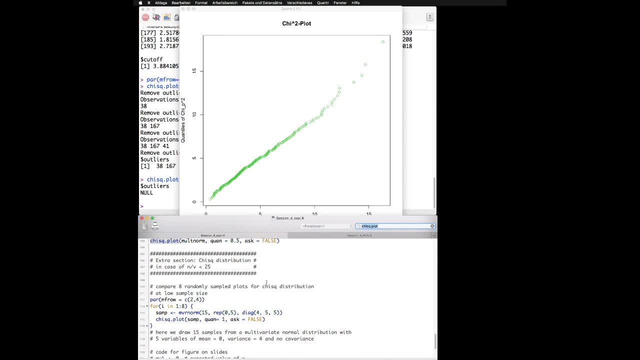 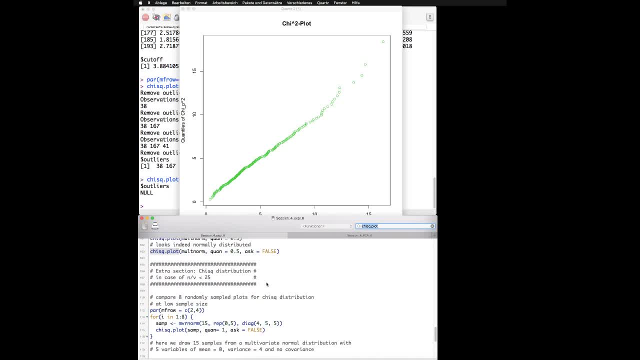 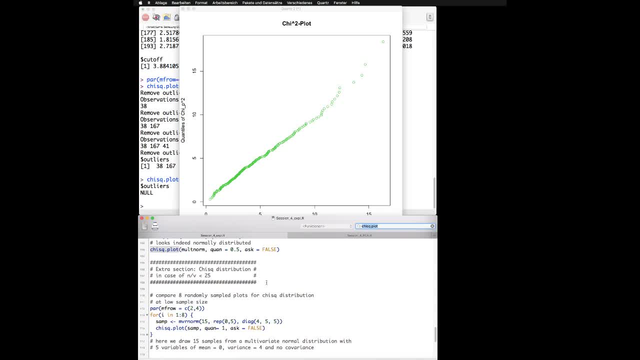 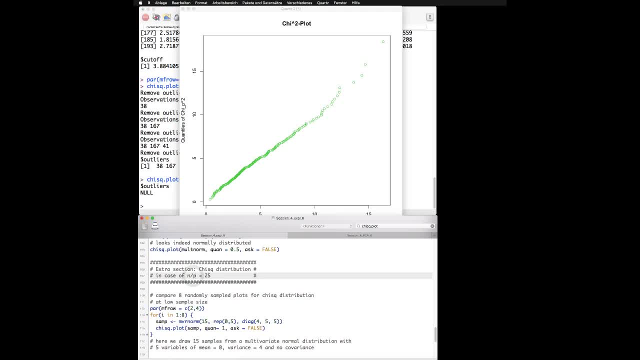 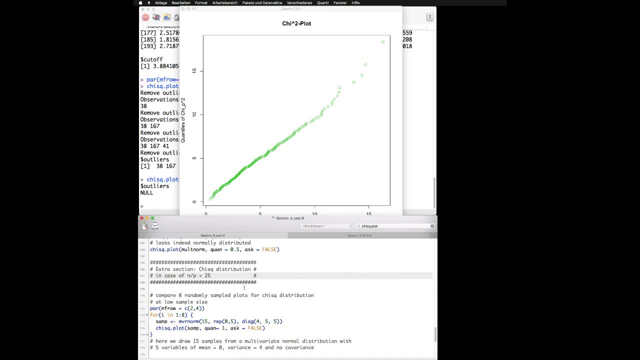 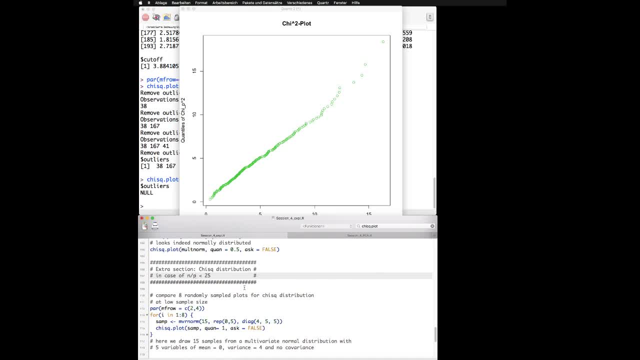 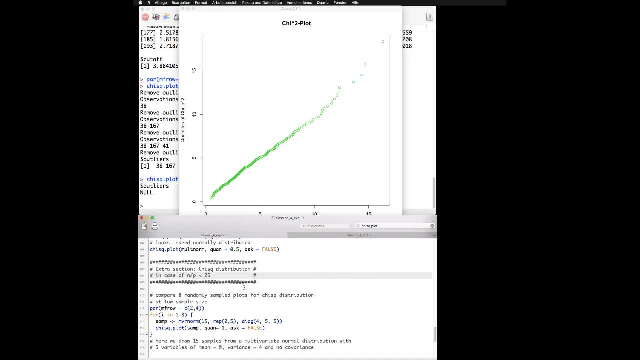 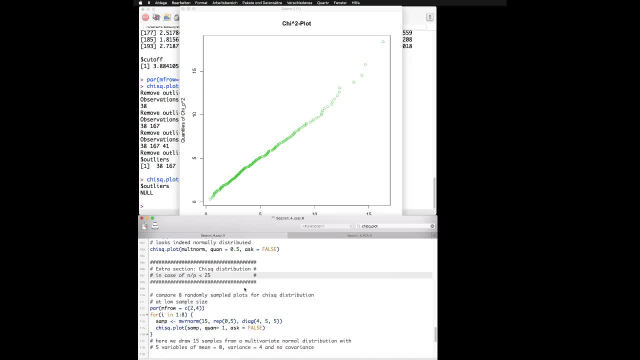 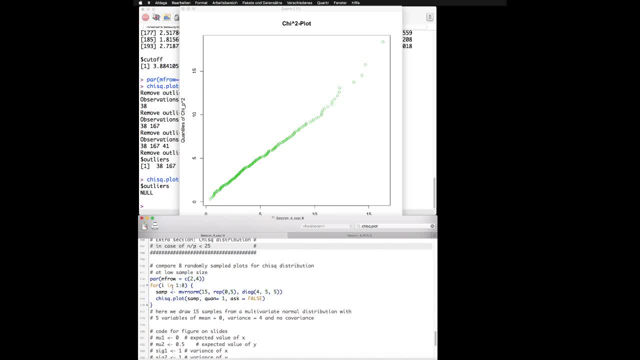 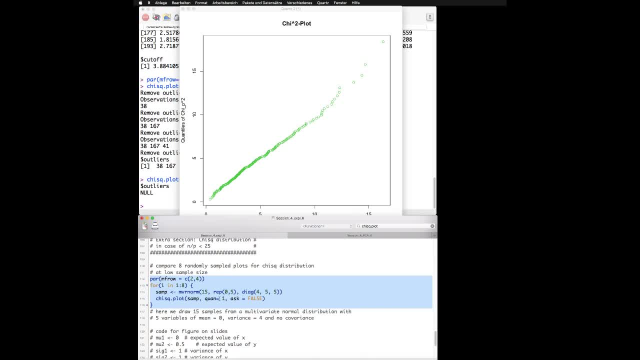 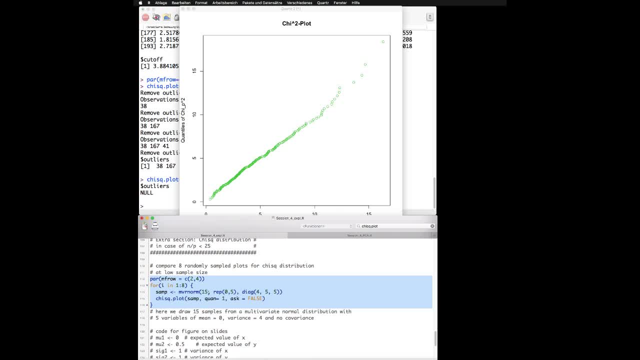 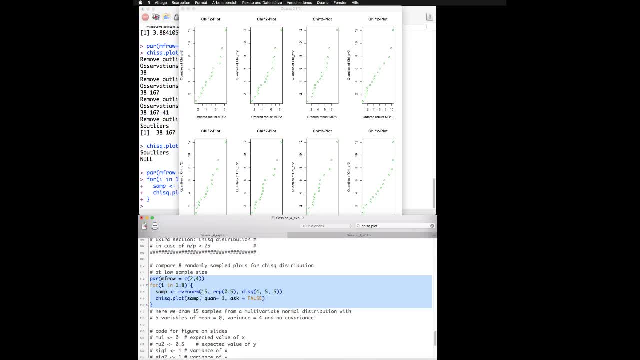 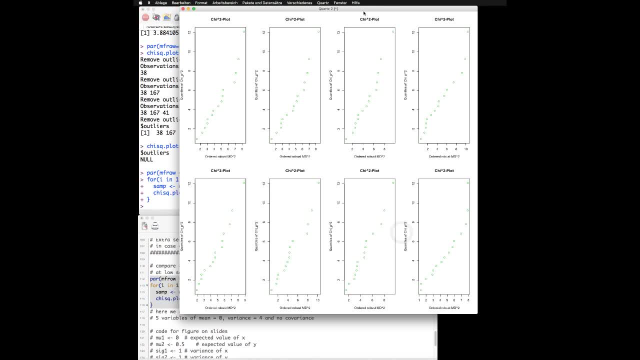 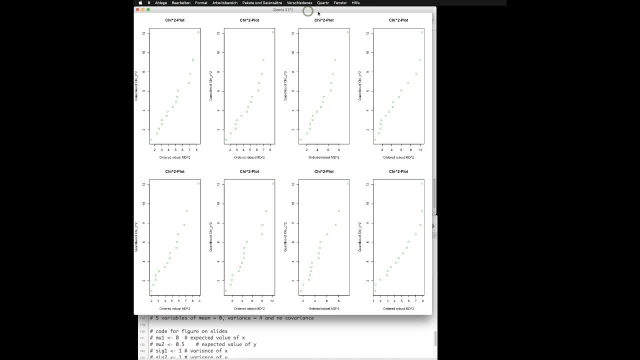 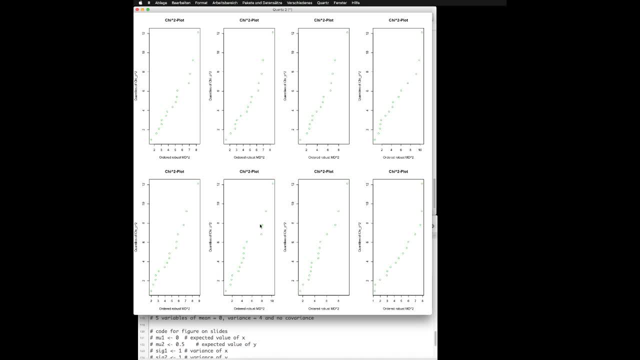 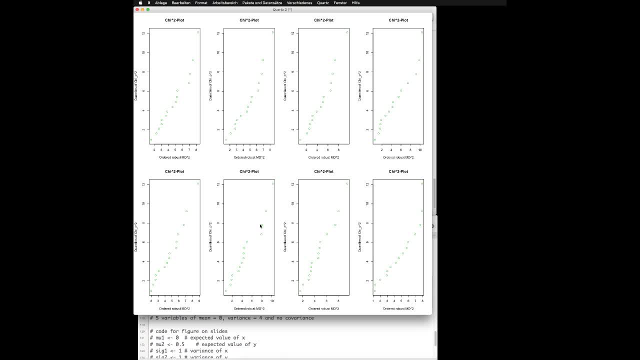 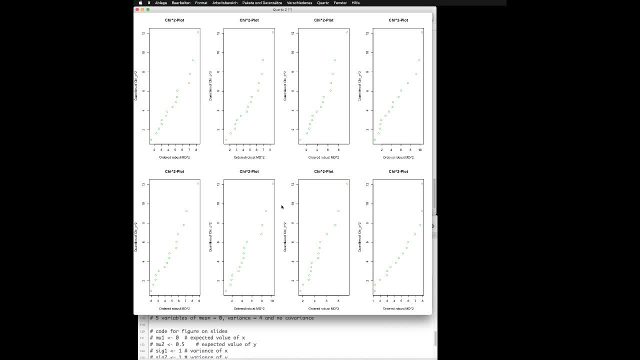 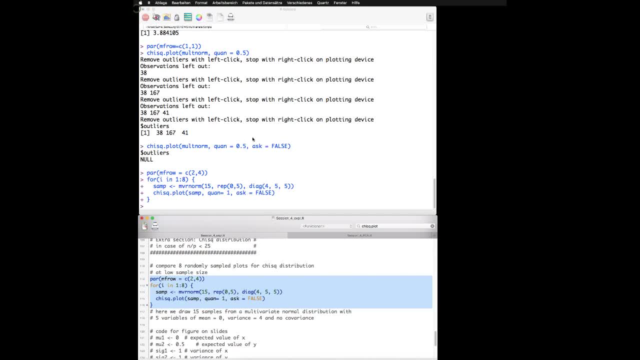 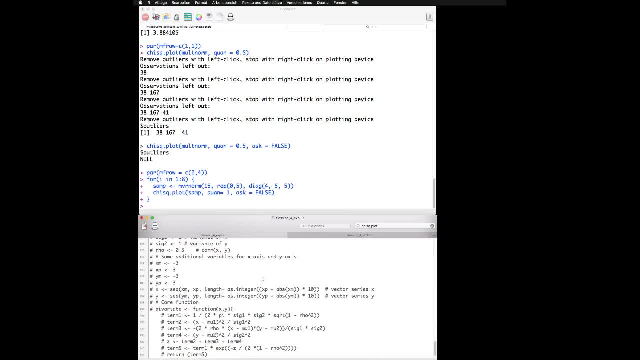 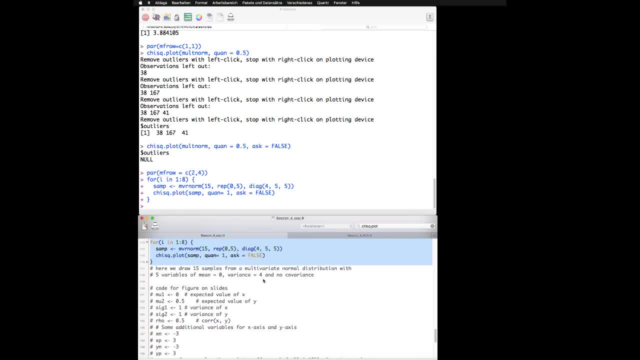 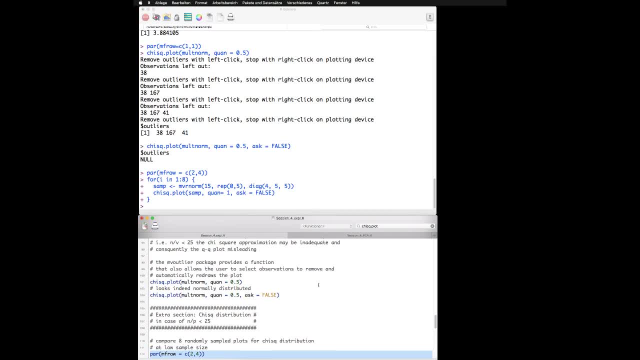 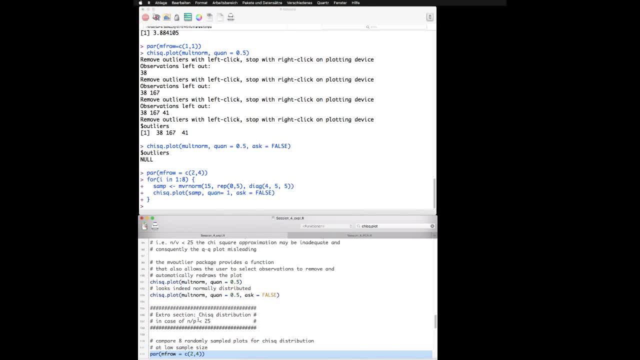 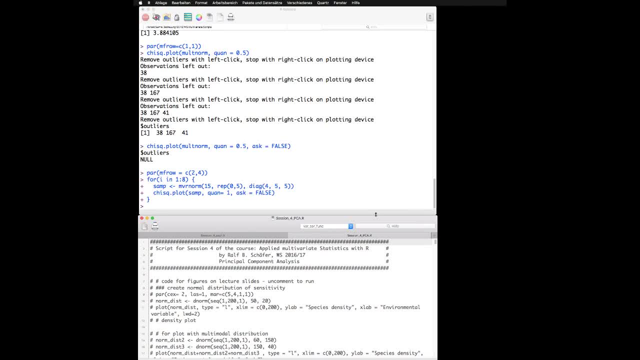 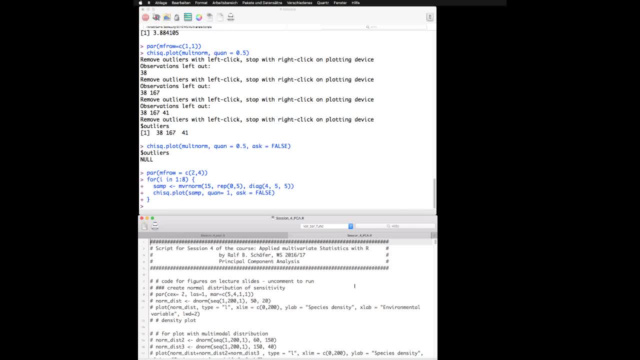 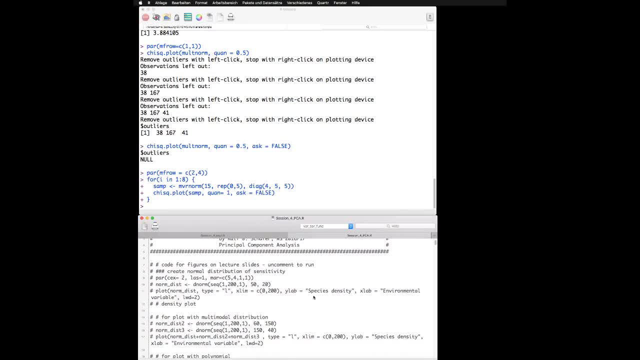 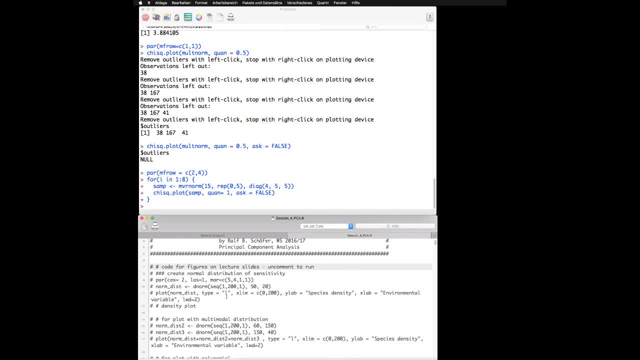 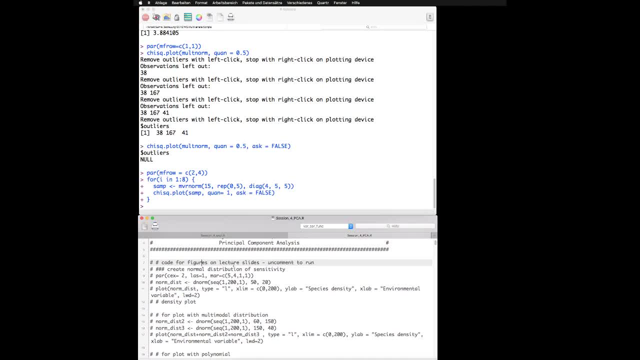 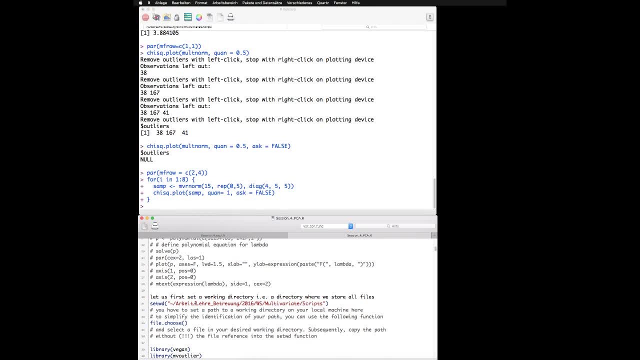 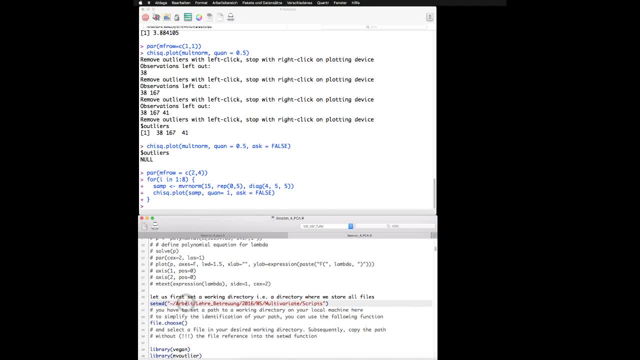 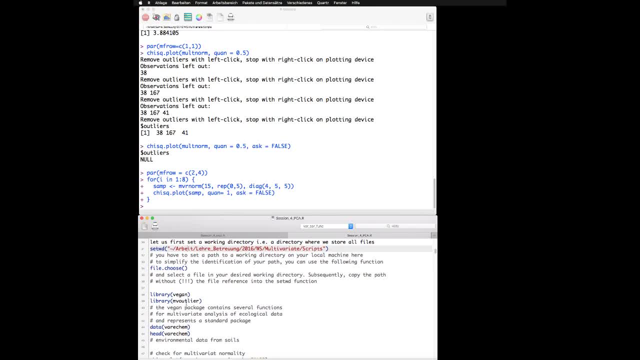 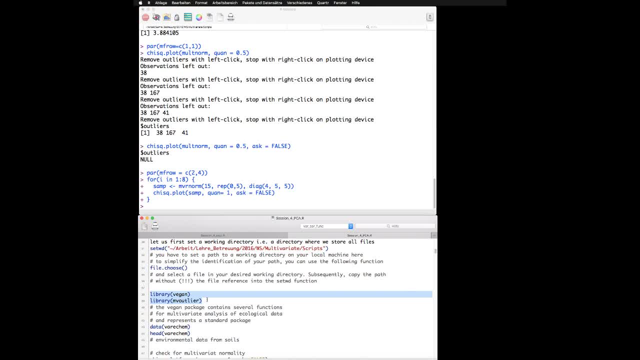 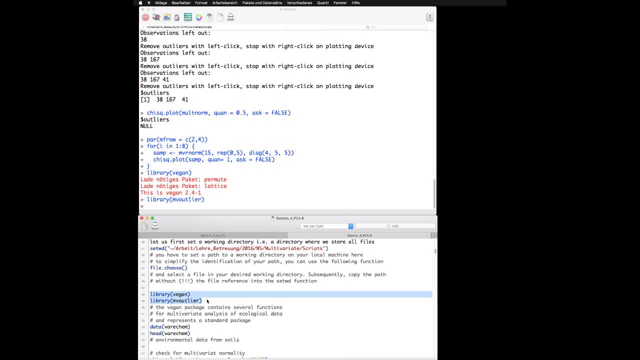 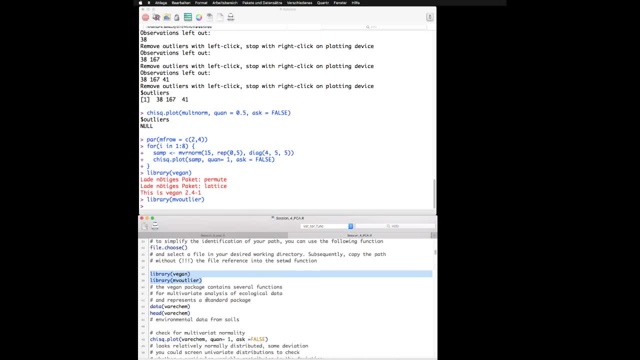 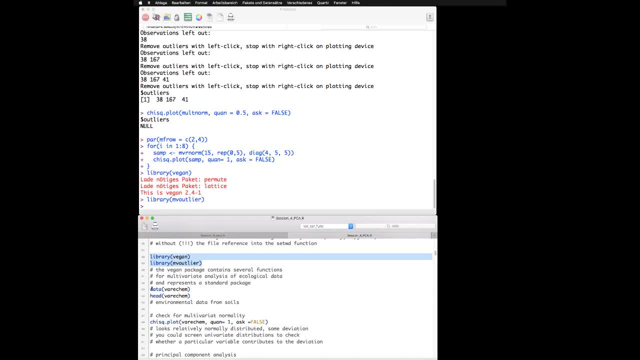 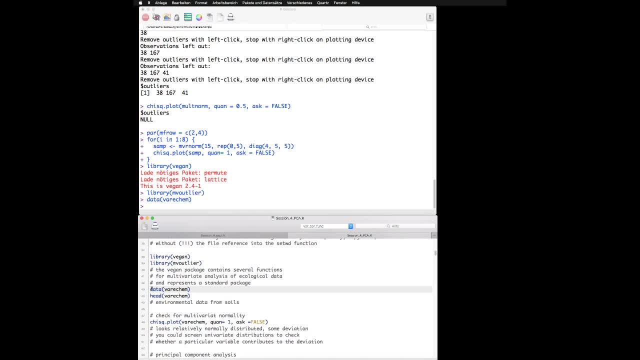 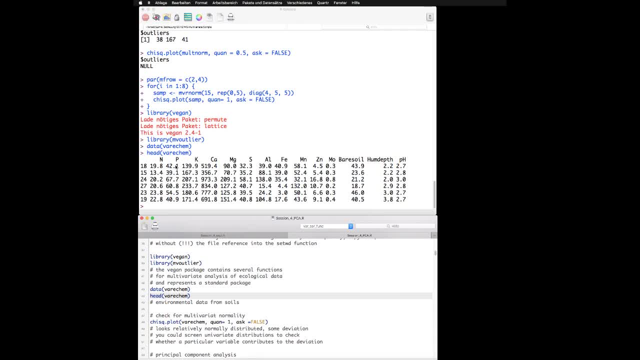 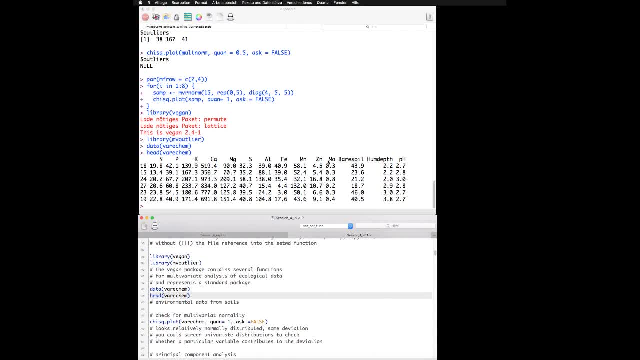 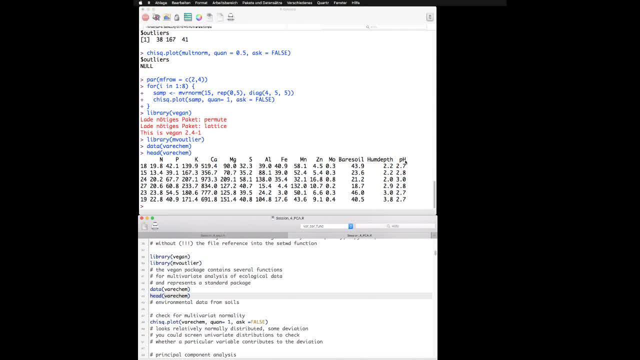 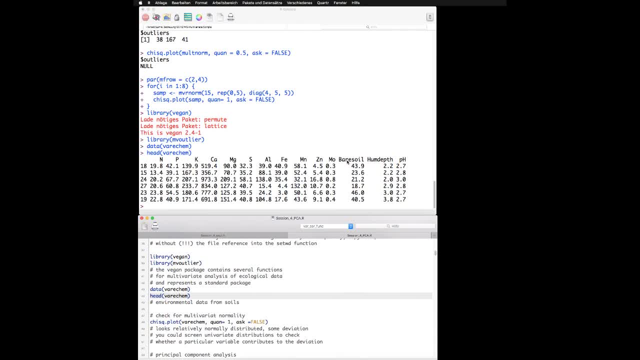 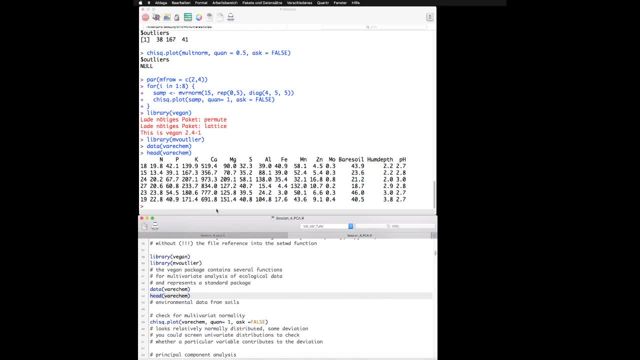 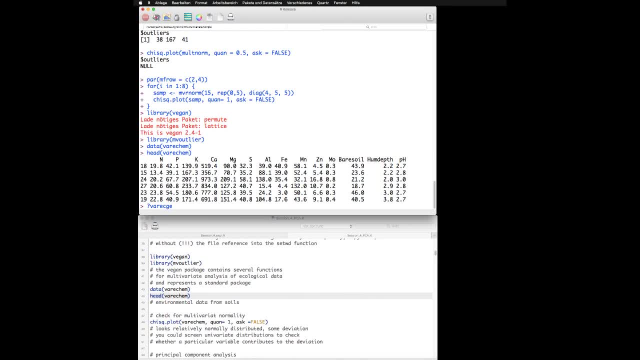 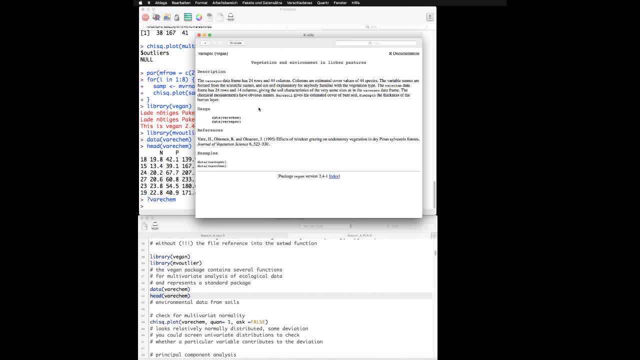 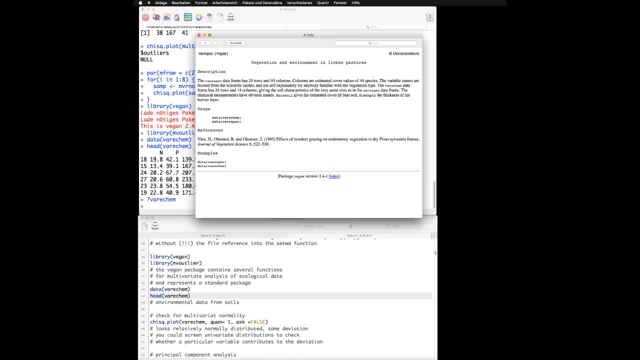 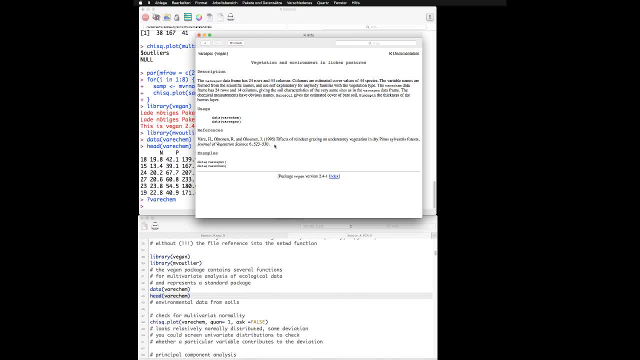 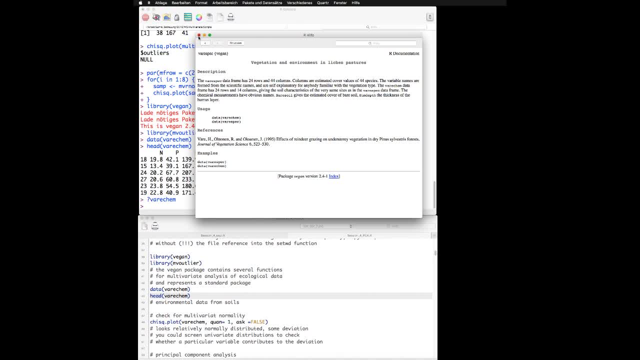 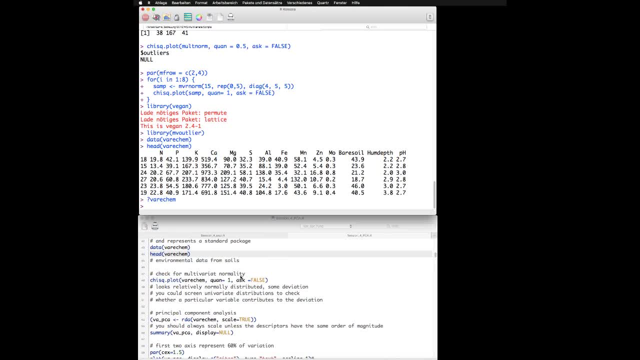 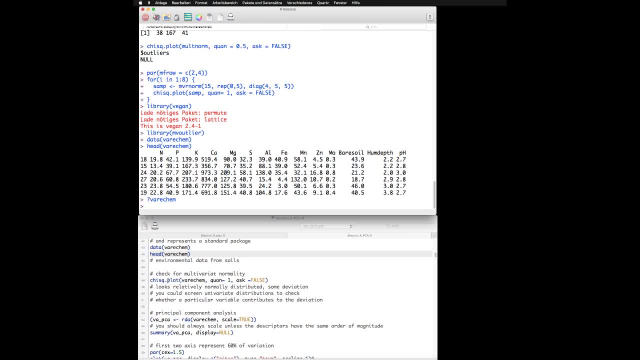 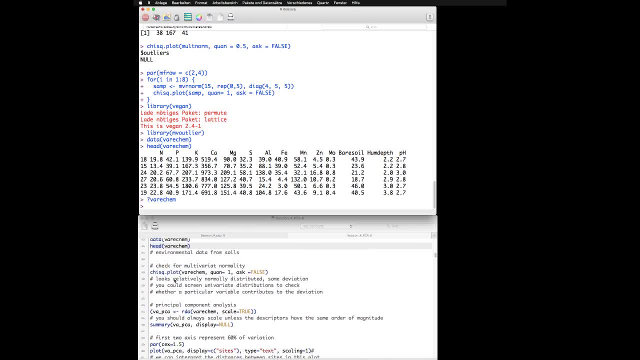 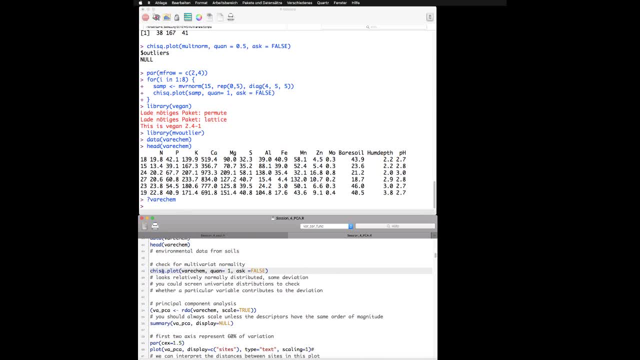 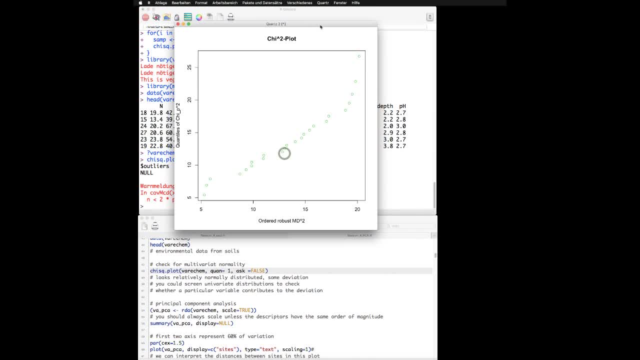 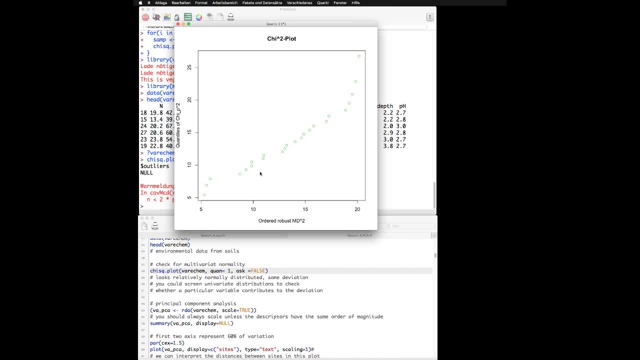 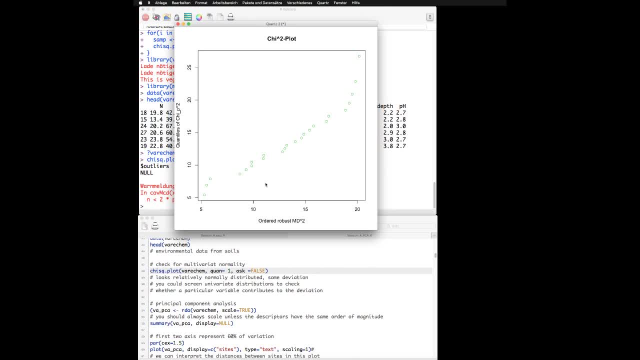 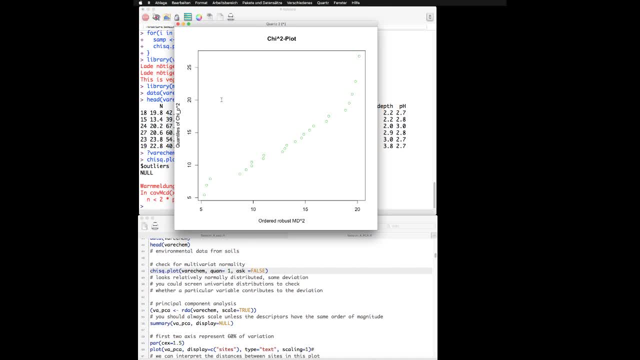 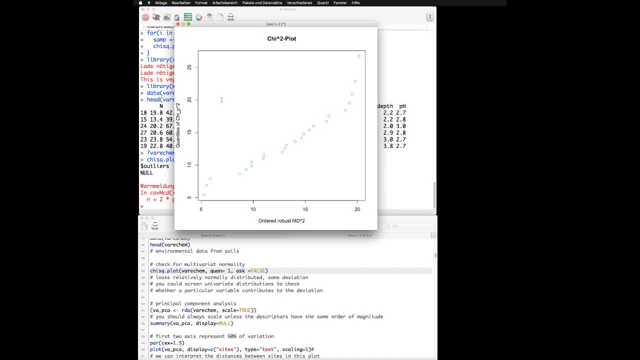 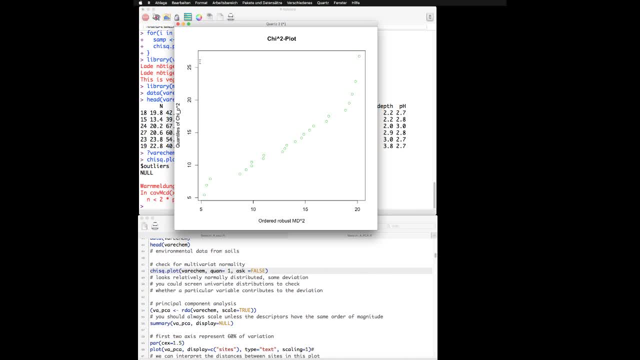 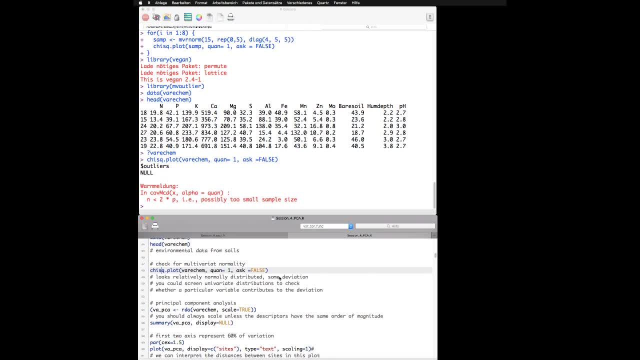 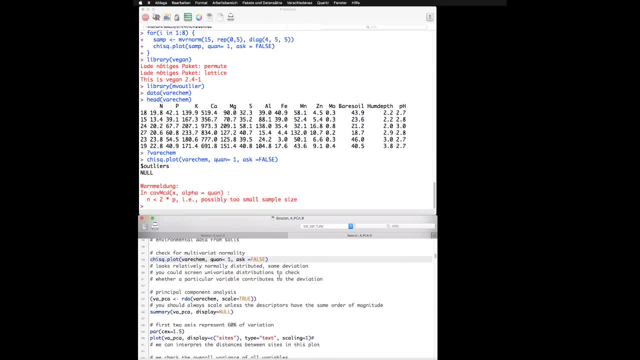 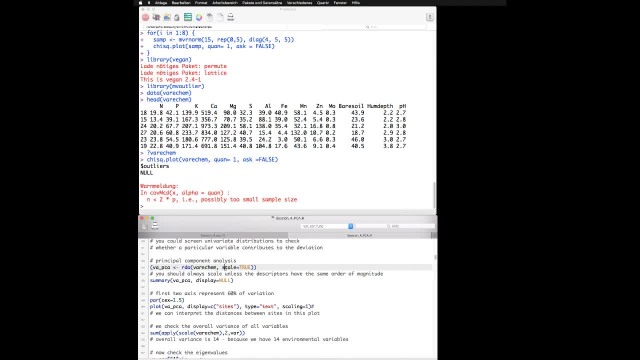 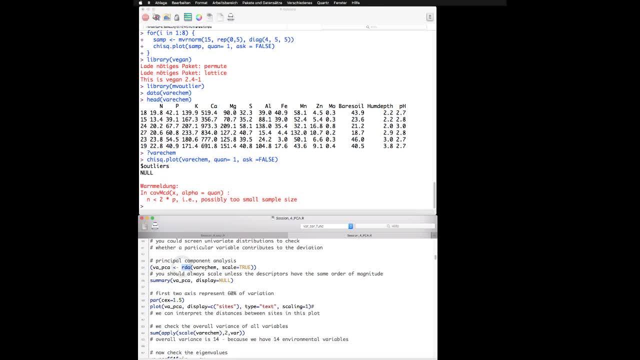 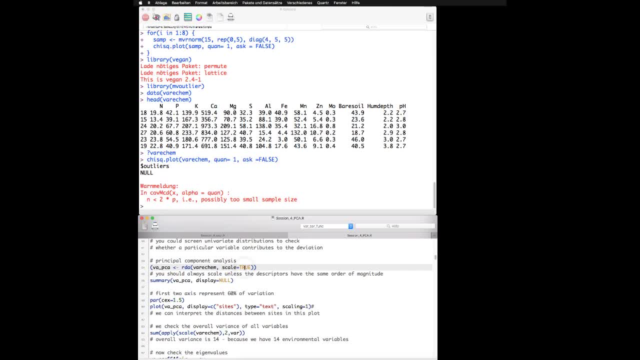 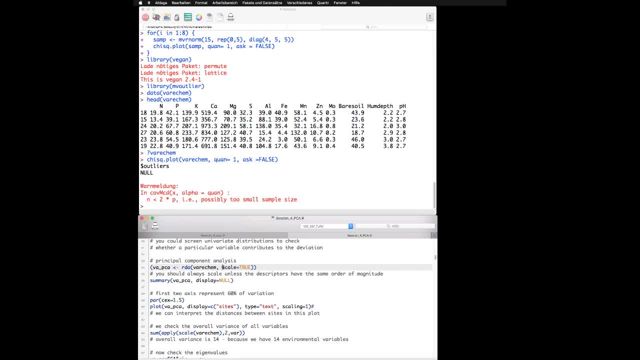 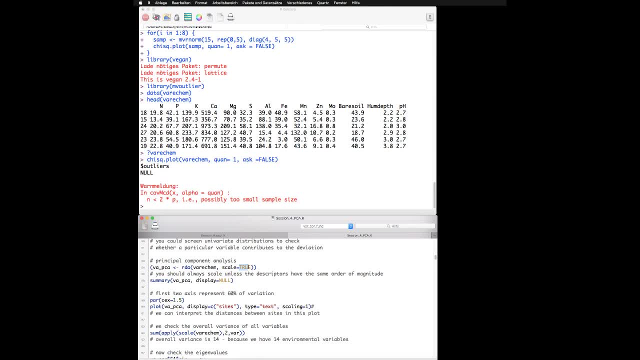 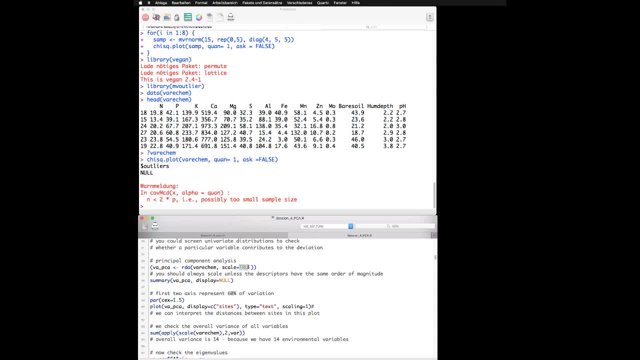 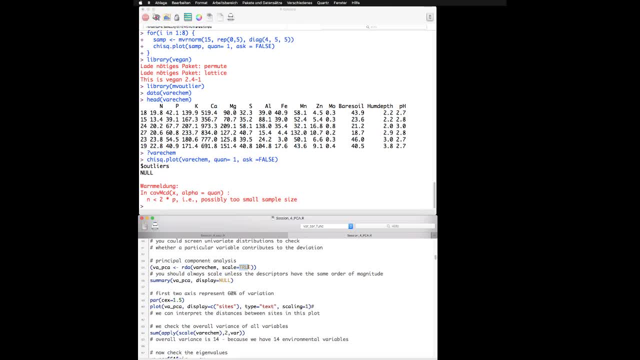 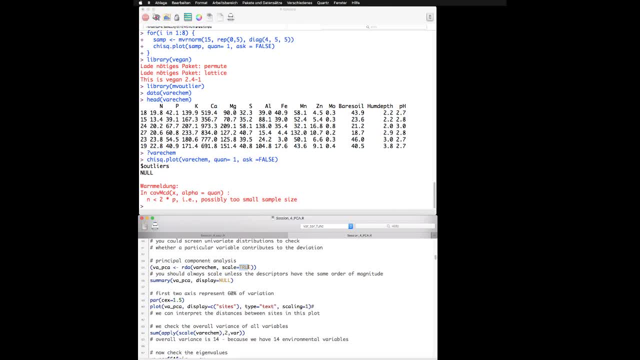 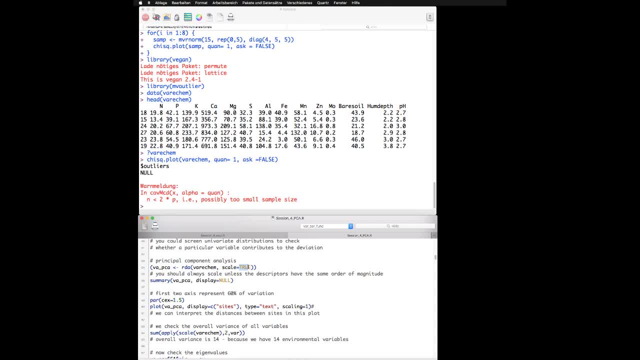 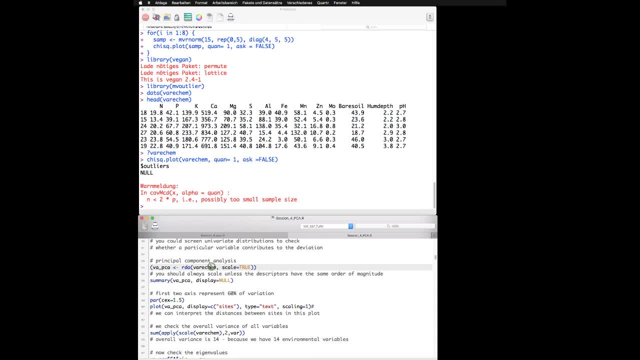 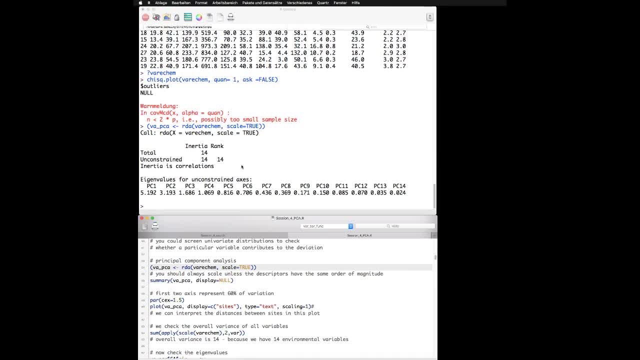 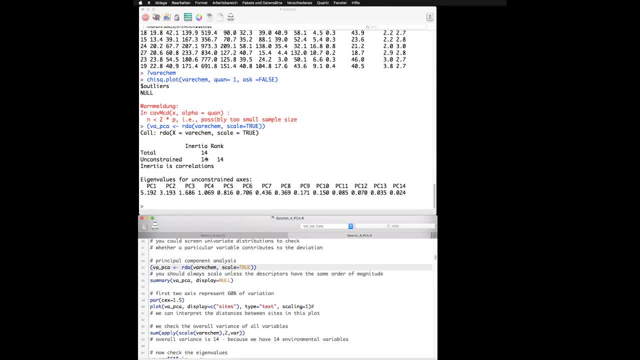 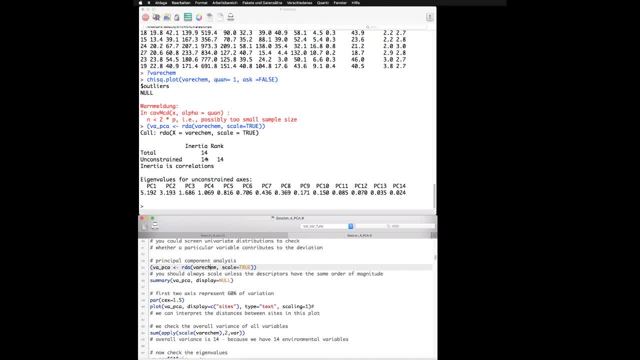 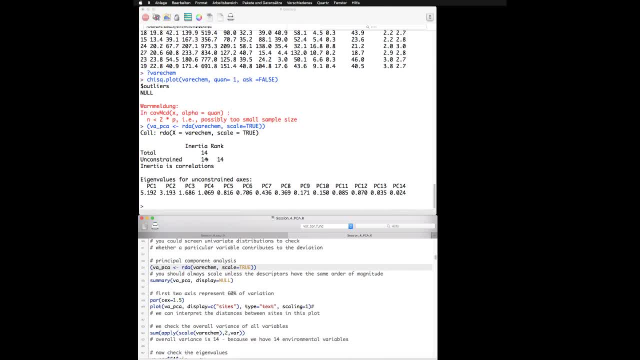 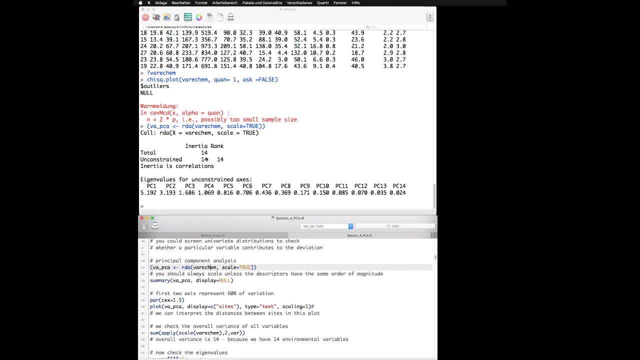 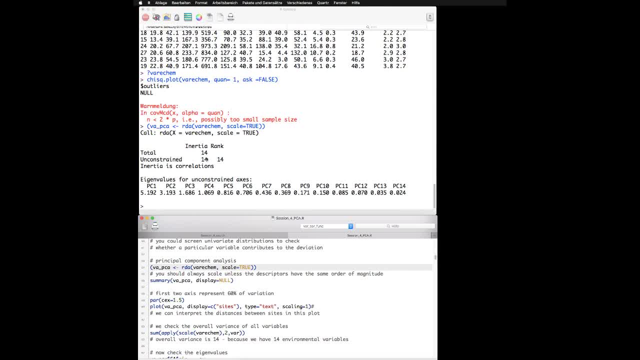 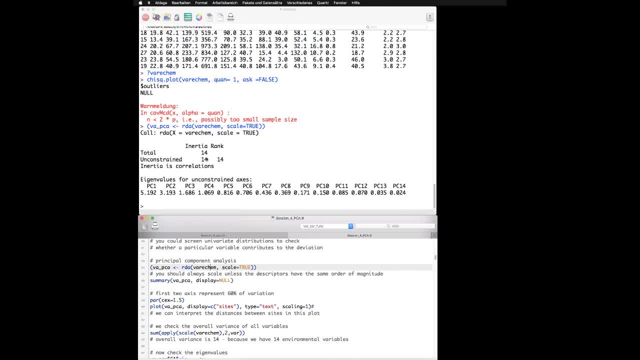 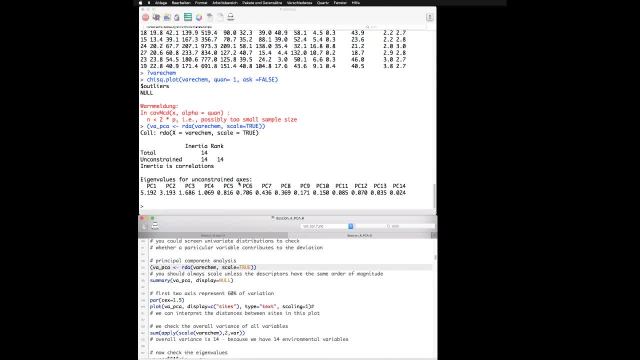 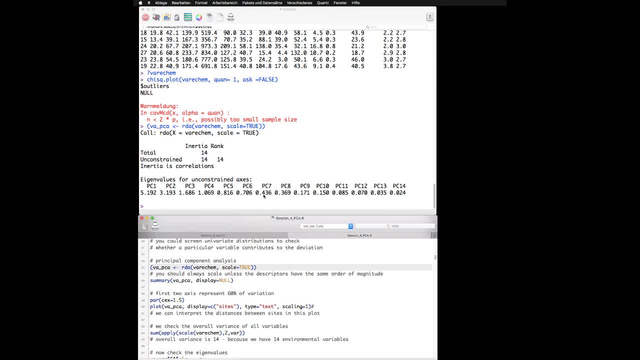 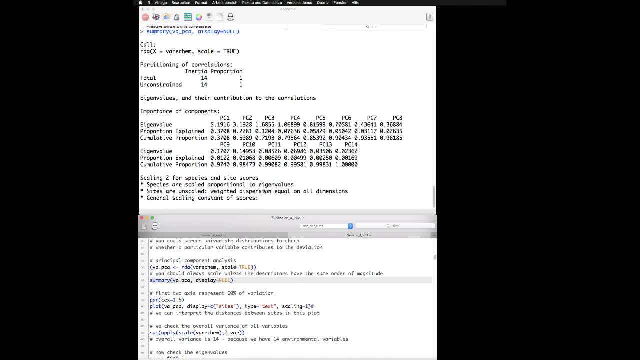 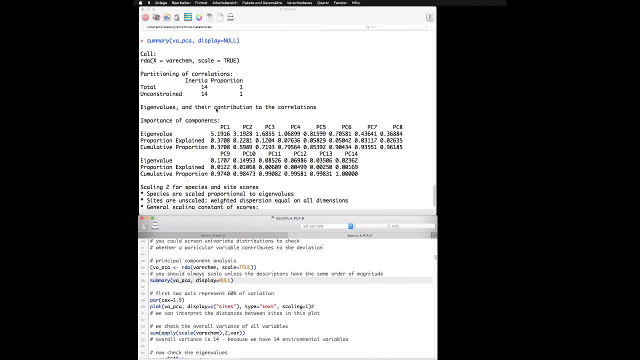 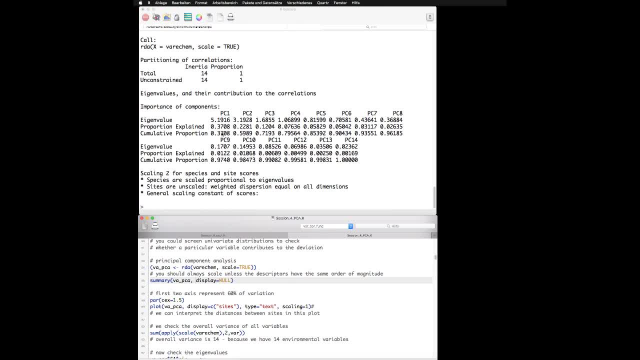 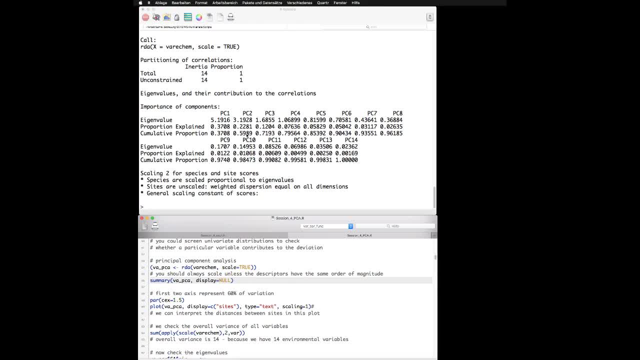 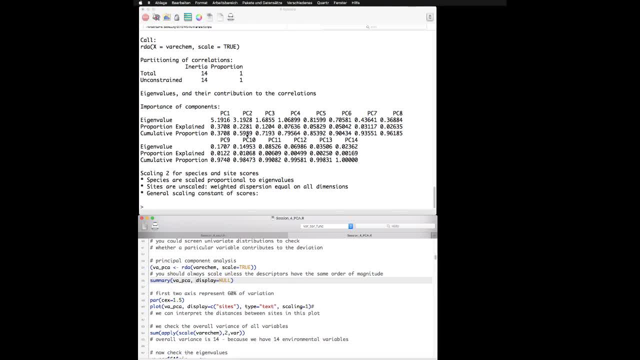 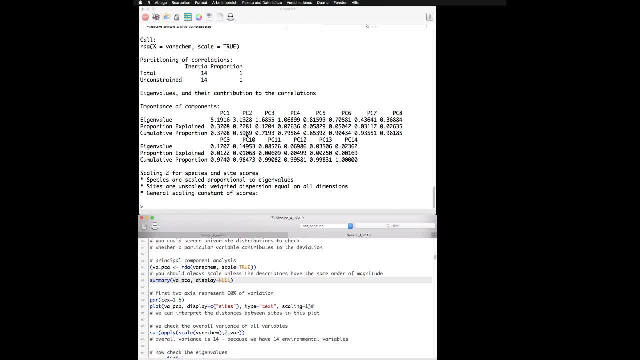 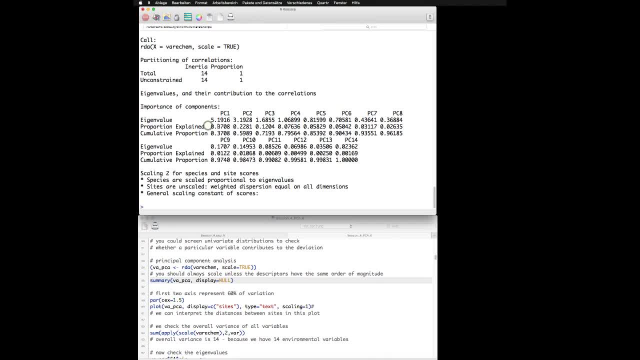 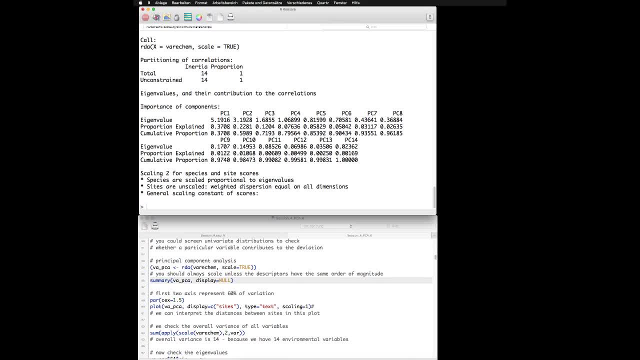 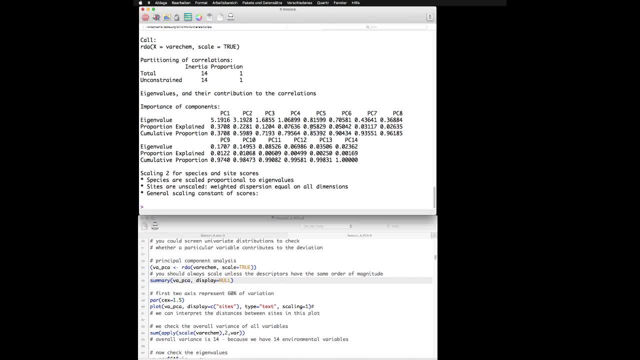 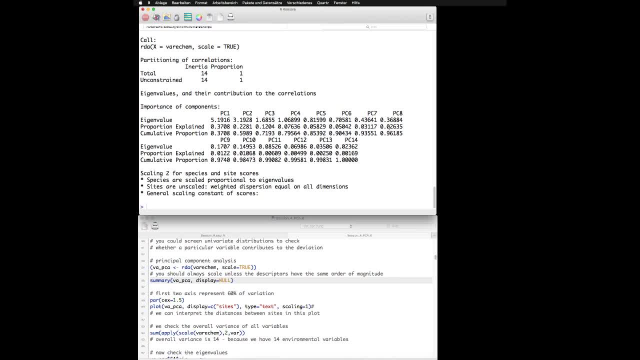 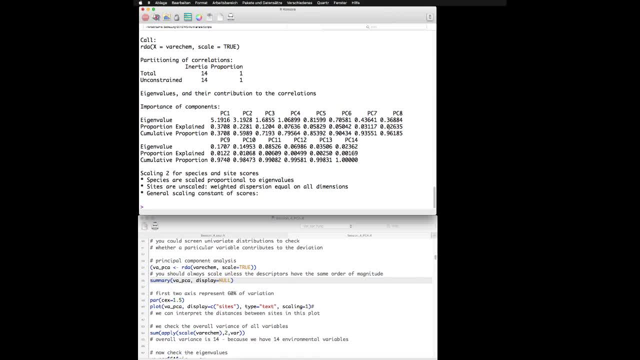 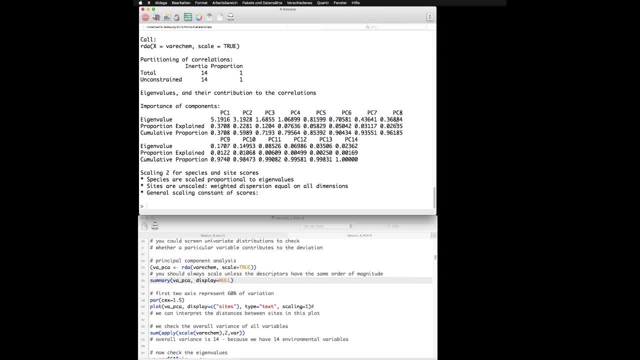 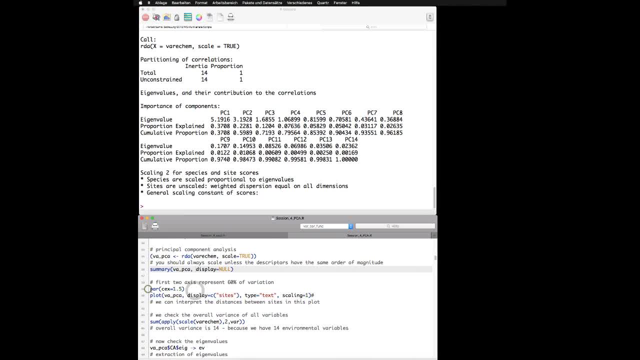 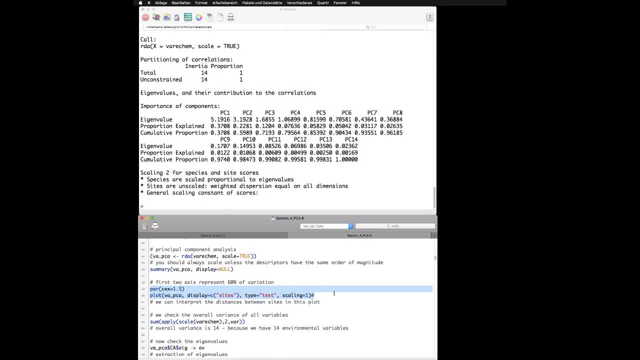 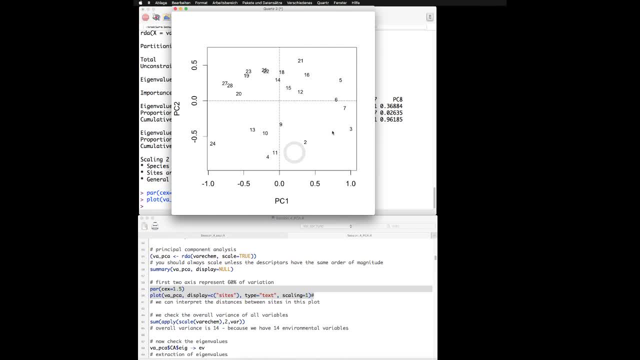 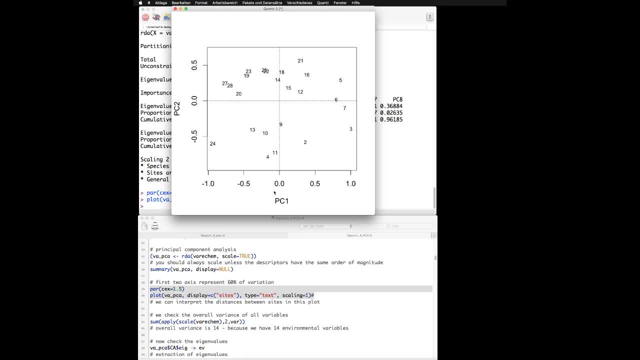 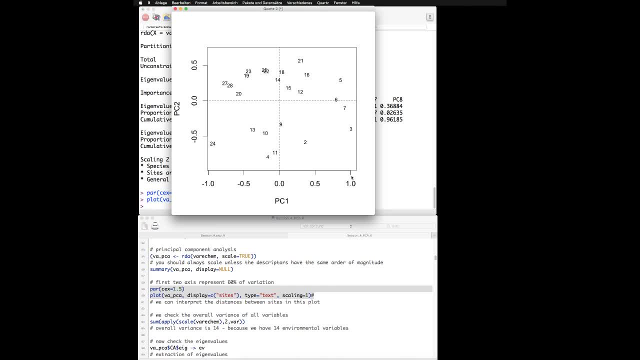 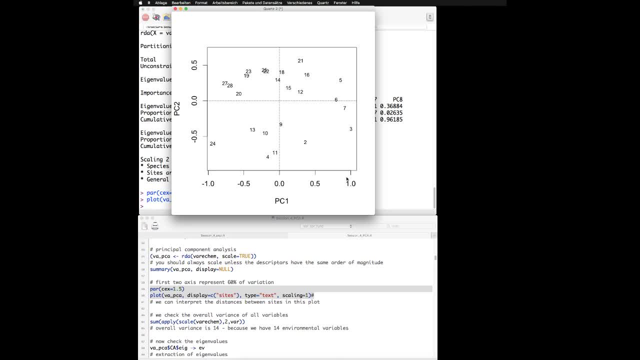 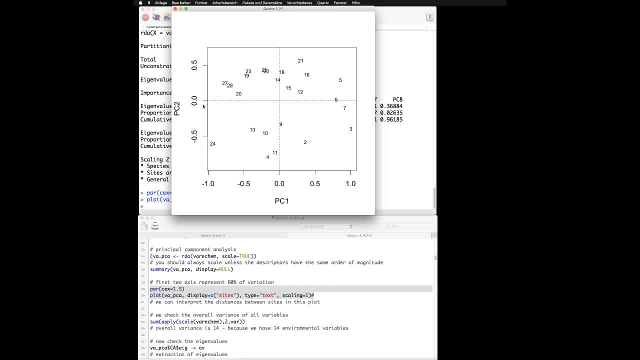 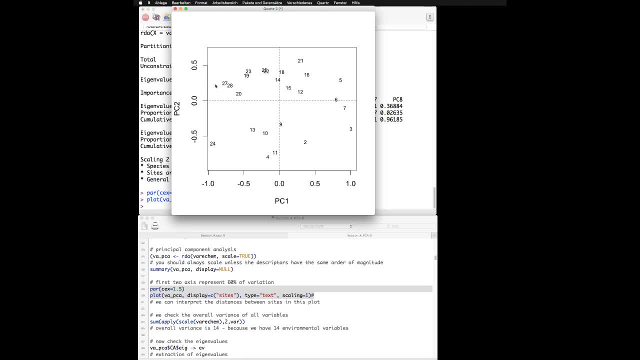 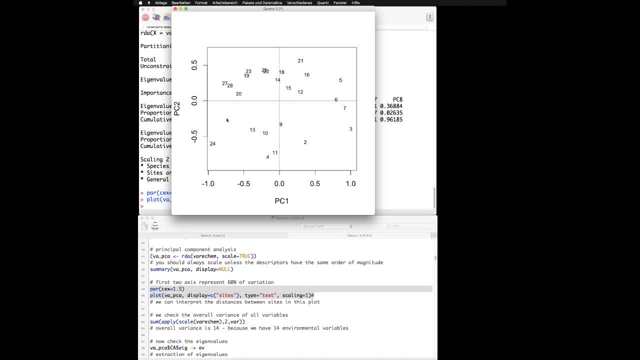 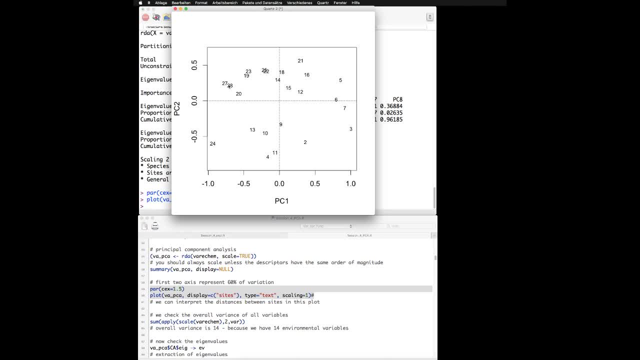 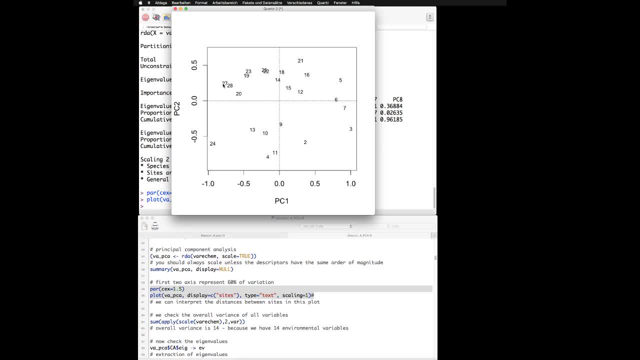 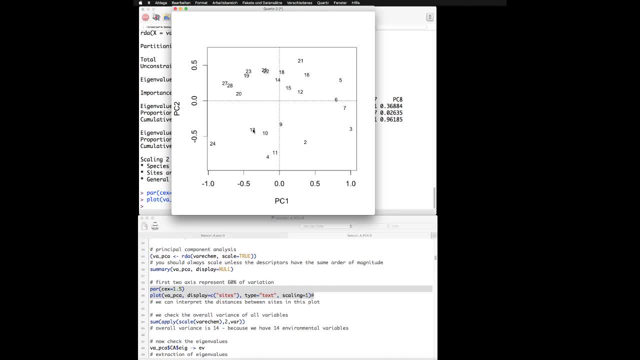 that the variables that are measured inside 10 and like 13 have relatively similar values and the values of variables that have been measured of this descriptor inside 24 and inside 5, more or less, have the maximum distance of all sides. so why is that? first of all, the distance. 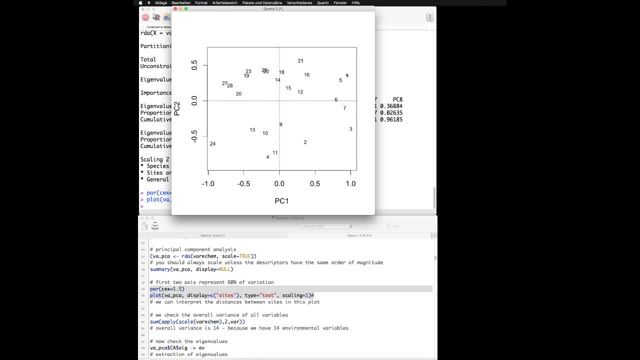 should be maximum. on the first principal component, that would be some now 24 and 3, 7, 6, 5 all have similar distances and if you also look, include the distance on the second principal component and we see that five has more or less the largest distance to 24.. 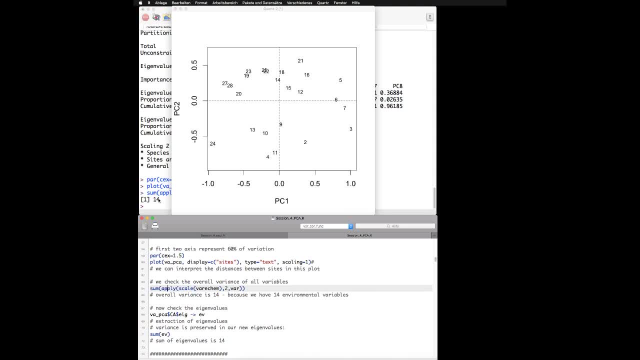 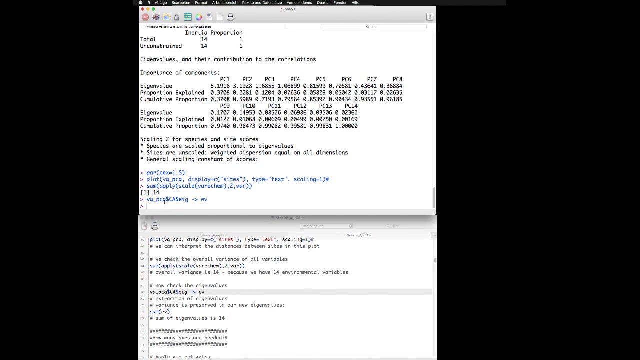 you can also check the total variance. as we discussed before, that is 14, because we have scaled our variables. we have 14 environmental variables, each with a variance of one, and if you wanted to extract eigenvalues, you can do it with this. with this, elements of our 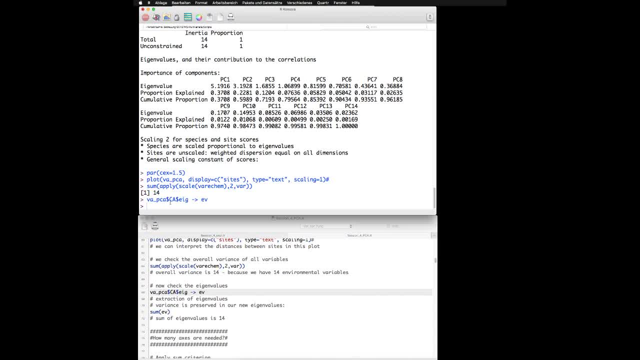 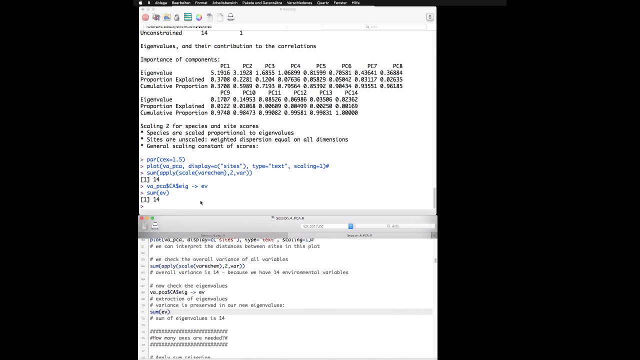 objects. this va underscore pca and the ca at that i um element of of this object. if we sum that up, not surprisingly, we see that the i total sum of eigenvalues is also 14.. so now we move to the next question: how many axes are needed in our principal? 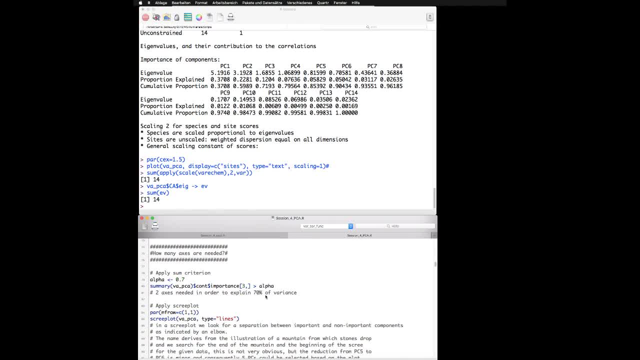 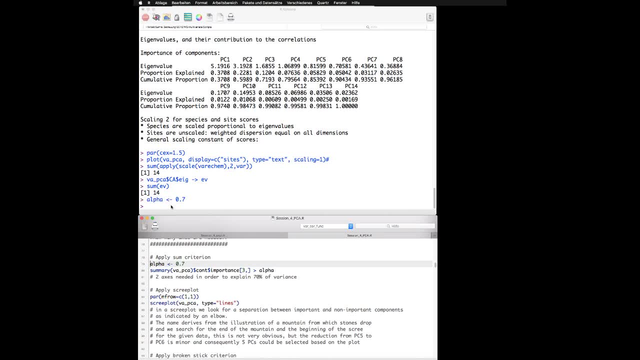 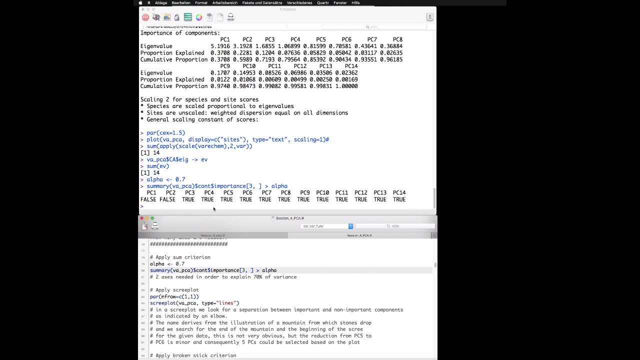 component, how many principal components are needed. so we have discussed the sum criterion. you set a sum here of 70 for the alpha and then we take the summary of the pca and and look at the difference and ask how many axes we need and whether the value is larger than 70 percent. and we see that if we have just 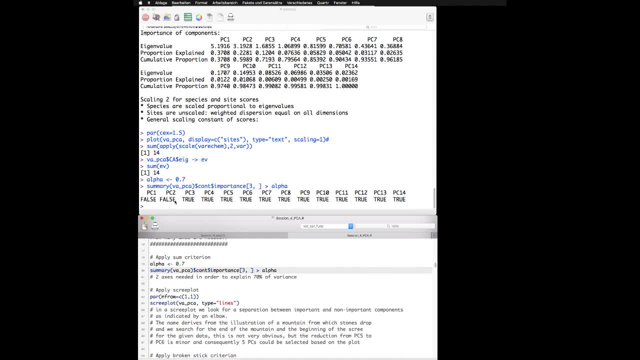 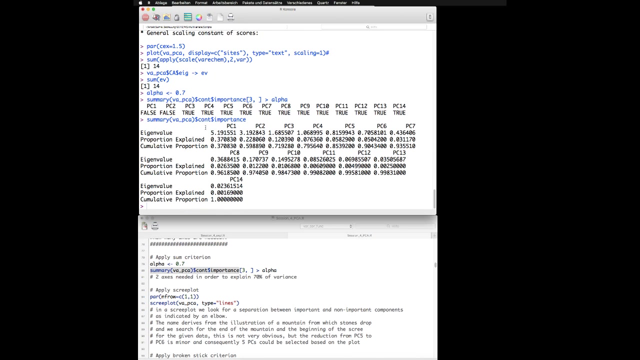 two axes we don't yield 70 percent of explained variance. but once we include the third, principal component, all data explains already 70 percent of the variance. so if you would just execute this part, you would see we have here the eigenvalue proportion of explained variance and cumulative. 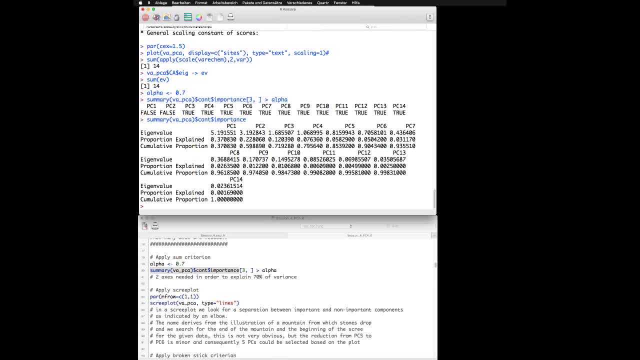 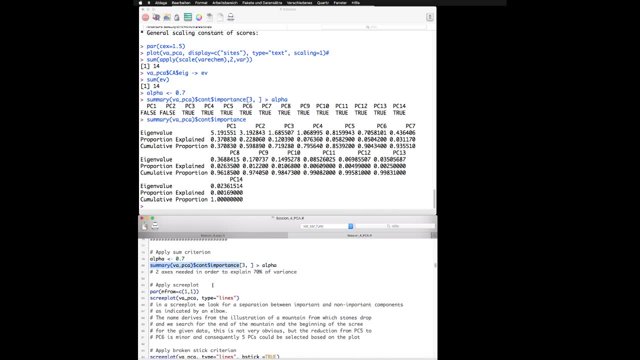 proportion. what we extract here is just the third row, so the cumulative proportion, and compare this to the 70 percent and we see with this third principal component we we exceed the 70 percent criteria you could also use in scree plot, the scree plot. in the scree plot we plot the different eigenvalues against the number of principal components. 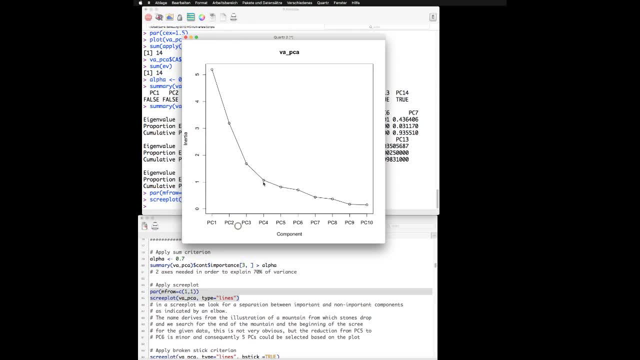 so we do this here and what we look for is something like a clear elbow where we see that there might be a point where we have only a minor degree. so we have very, very strong drops in the inertia, in the explained variance and at some stage that is leveling out this degree. so 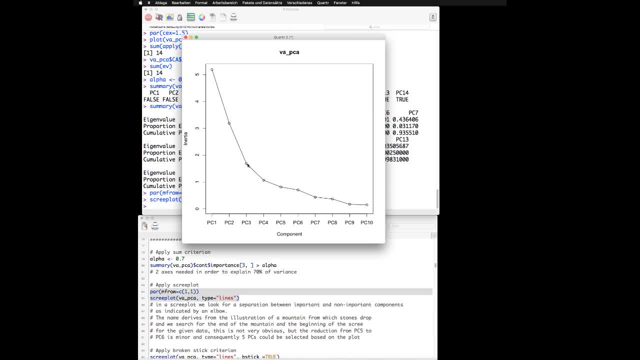 these are fairly similar and you would probably here choose also three or four or five components based on the scree plot. as we have discussed, this type of of plots are somehow more subjective form of choice. so, whether you define that at the scree, this creepy plot indicates three to five of the principal components. 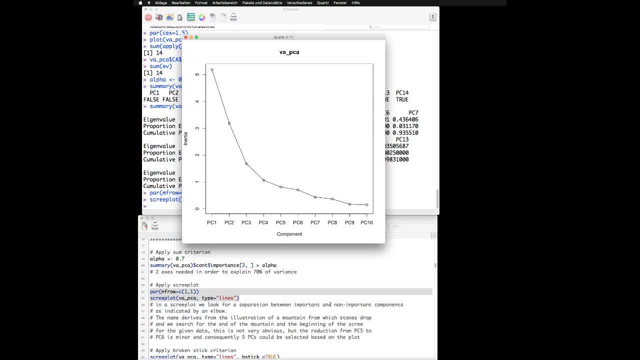 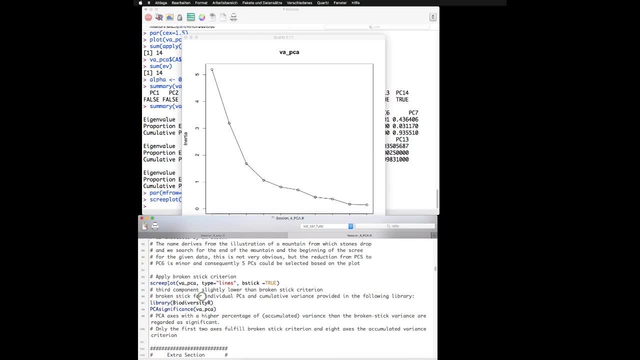 it's. it's rather subjective choice and depends also on your objective of the study. we can also apply the broken stick criterion. that's done here. so we plot above the ordination variance, we plot the variance that the broken stick. if you have this random broken stick model, if you would have that, then three: 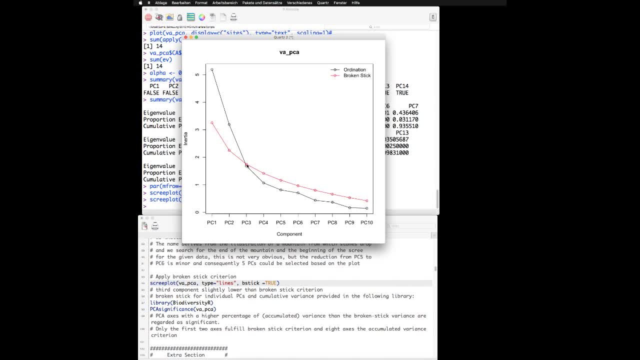 of the principal components would explain slightly more on the third principal component would explain slightly more than the third one from the ordination and you could, you could evaluate or assess, come to the conclusion here that if a random breaking of a stick would lead to more variance on the third axis, then in our data, then the amount of 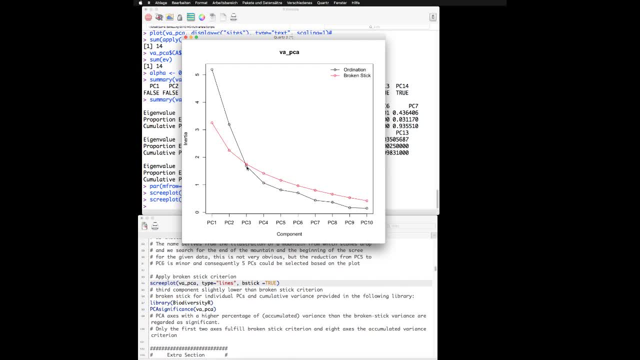 variance in the third axis is less than you would see from random data, then it's perhaps not that meaningful. but again, it depends very much you could evaluate or assess. come to the conclusion here that if a random breaking on the scope of your study and if you can include several variables, 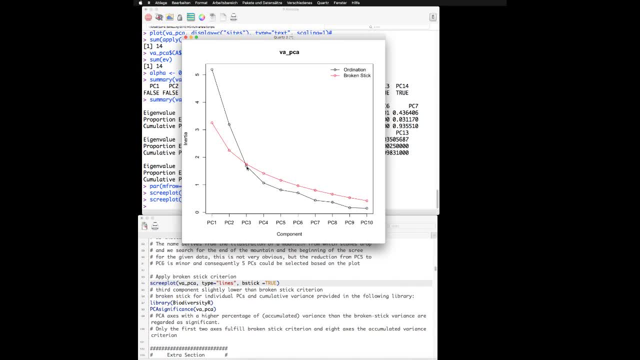 if your aim is not just to display, visualize the relationships between sides and descriptors, but you also want to conduct a follow-up analysis, for example, principle component regression, then you should include more principal components that may be needed and then maybe then those that may be needed under the broken stick criterion. 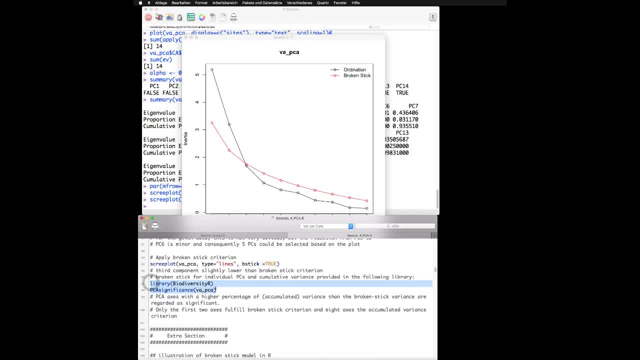 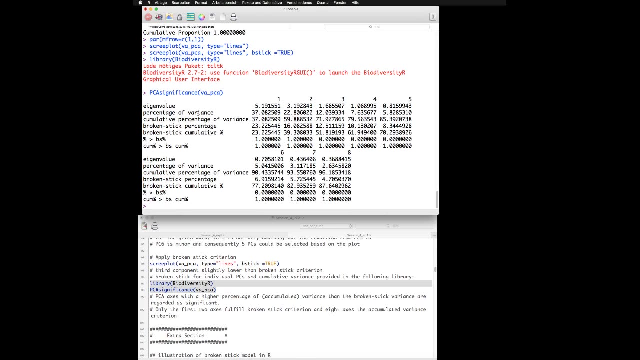 So different. Why of using the broken stick criterion is provided in the library biodiversity are. in this library that features a couple of Functions for biodiversity analysis. you have a more informative output of the numerics We see here: the broken stick, the cumulative broken stick and the individual broken stick provided. So we see that. 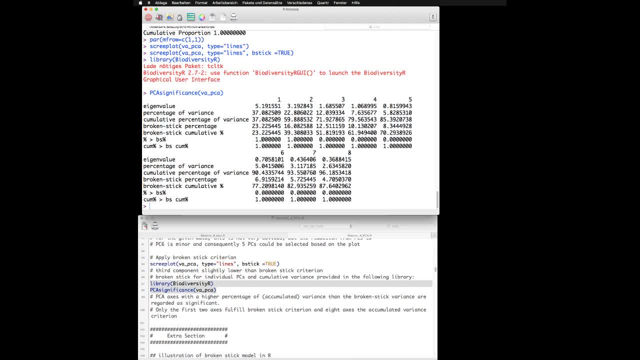 If we focus on the individual broken sticks, Then we have only two axes that taxes the two principal components that exceed the amount. that is explained by principal components derived just from Broken stick model. and if we look At the cumulative proportion of random stick, then we would actually include all first eight principal components. 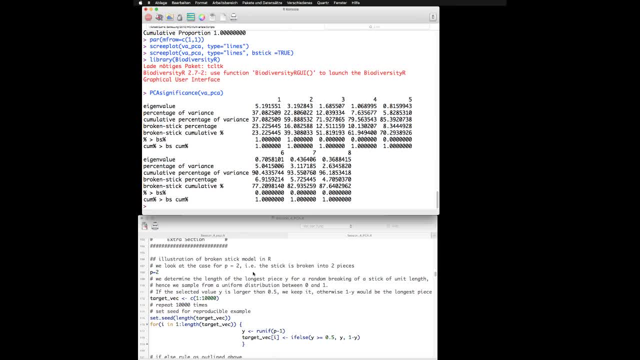 We have an extra. I provide you with an extra section section here that shows you how you run this principal and this Procrastiq model. I'm not going into details here. That's explained in the taxons, only for those that want to know how this. 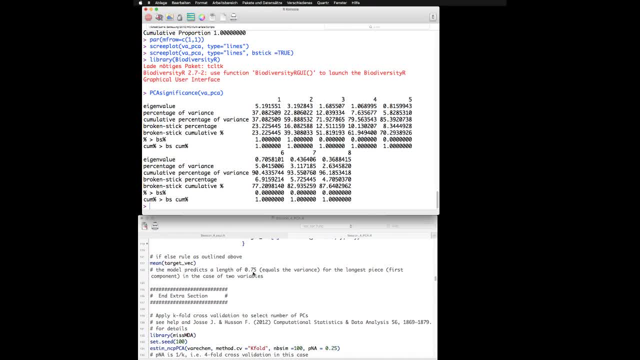 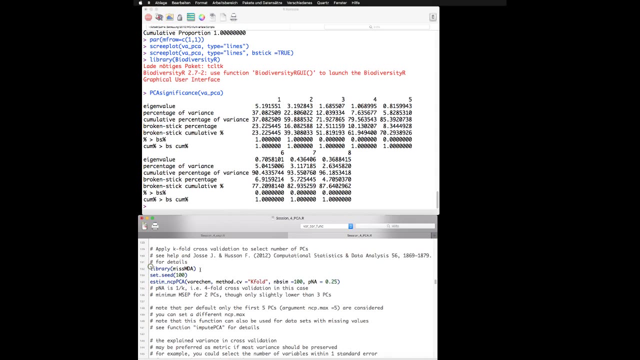 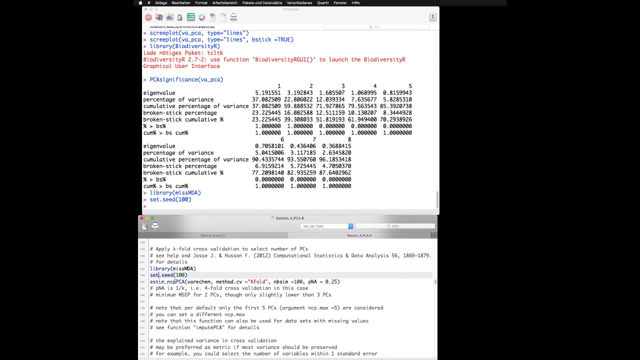 Broken stick model really works and how you can calculate this simply for yourself. The final technique that we have here is cross validation. We've encountered cross validation before in the course and we will use the function here to run k-fold cross validation. K-fold we will use here for fault cross validation. 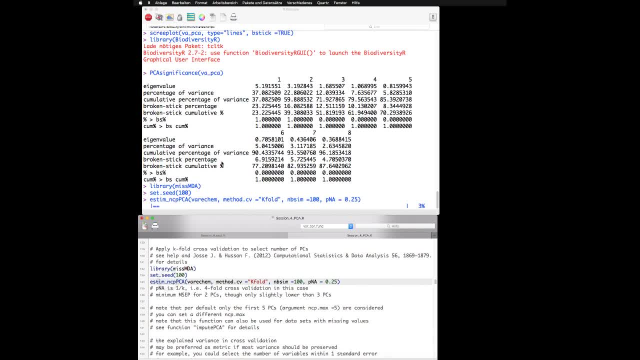 So we set the seed again so that we have a reproducible result, And you see that this takes actually a couple of seconds to run this function. So this is done as follow: the data are removed Using this function. so You provide here and then on how much data is removed, if here. 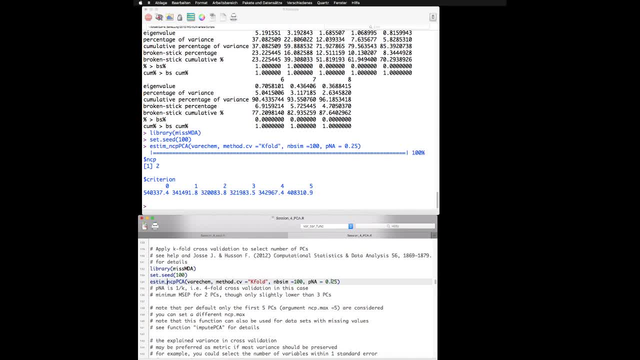 25% of the data are removed in one stage means you have for for cross validation, So You always use remaining 75% of the data to estimate These data. then you have the number of simulations. how often this is done. This is done here and this. 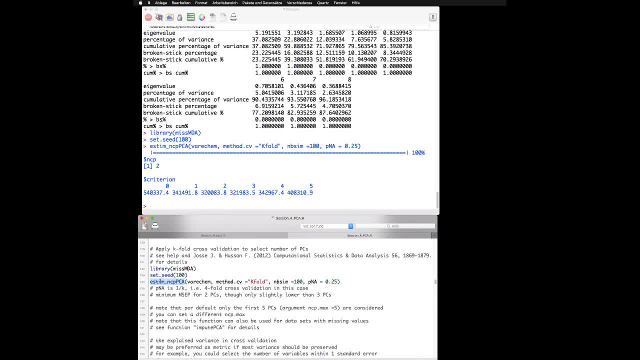 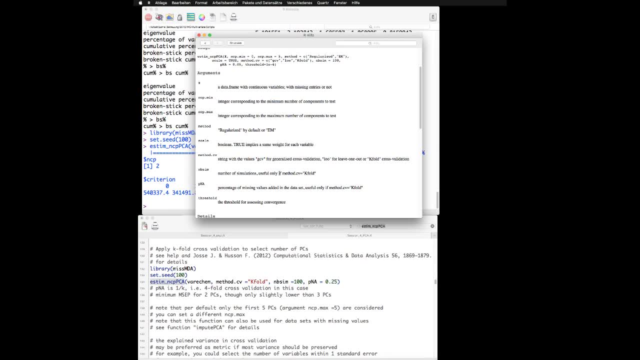 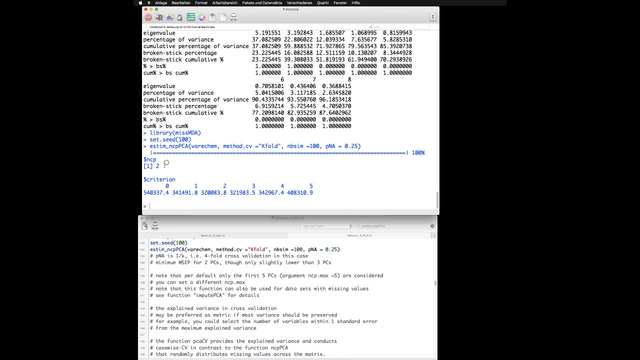 For this function. This is now the 100 times Wait so long and a couple of other arguments that are explained here. So if we look at the results, So if we look at the results, We see that the, based on this criterion, we choose, should use, should choose based on the. 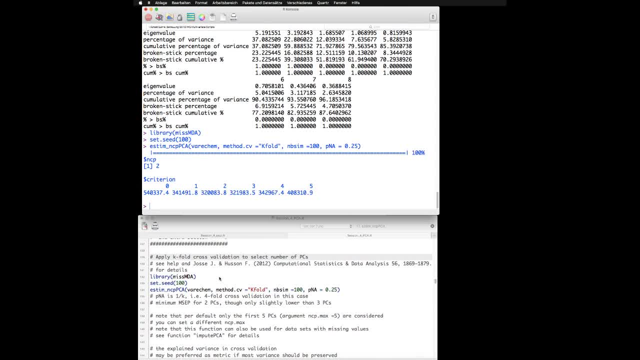 On the Mean sum of prediction error- Mean the mean squared error of prediction- Then we search for the minimum, So that's the minimum error per predictor in the model. And we see that if we have two predictors in the model, then based on the mean square per predictor and 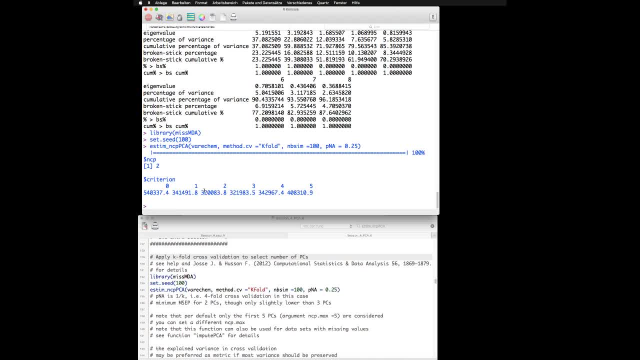 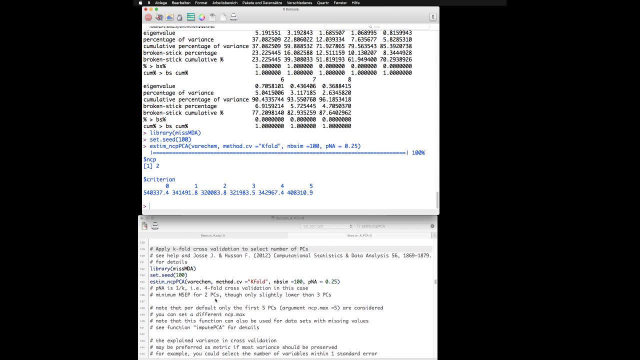 Mean square error per predictor. then having two of the predictors in the model and yields to the minimum, although even with three, that they did results of a Very close before two and three predictors in the model. So you could also use this function if you have missing values in your data set. that's explained in the function impute PCA. 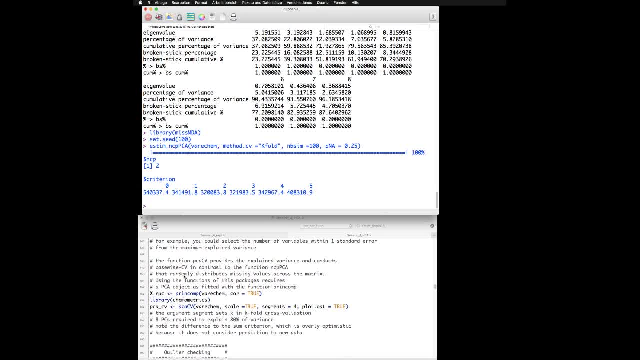 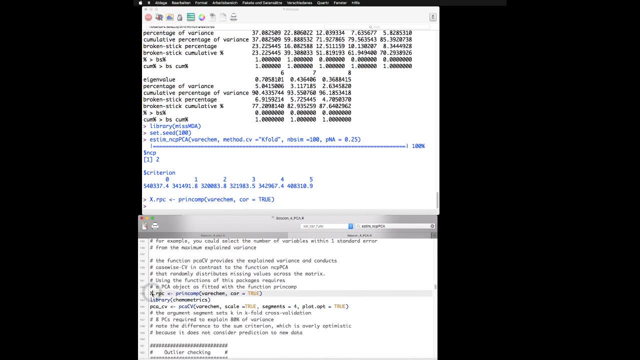 And There's another function which you can use for cross validation if you, for example, are Interested in the total amount of explained variance that it's conveniently provided in this functions For this. the function requires a fitted PCA object from the function print print comp, So it doesn't work with the vegan object. 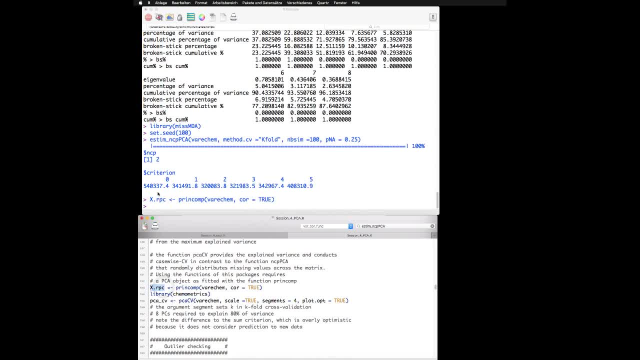 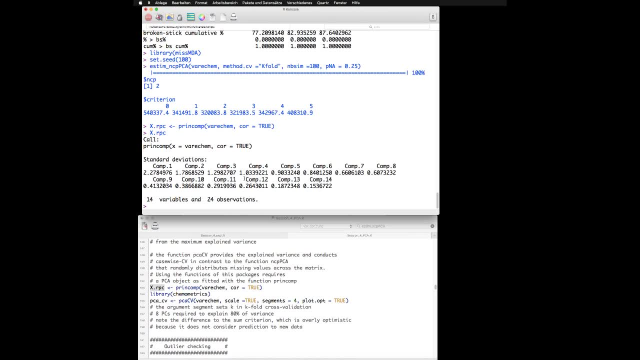 Although the result is exactly the same if we look into the X dot RPC. So if you compare this to the vegan, result is exactly the same. You see here also some design differences. in vegan You have the variance provided. here We have the standard deviation Provided per component. So these are the square roots of the eigenvalues. 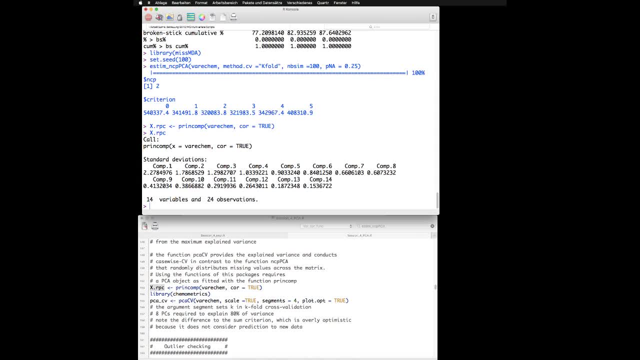 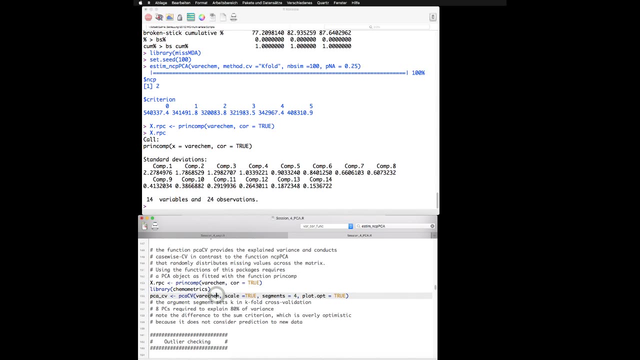 We could simply Use the square of this and then you would have the same results as for the RDA function And you have the Cobain partition And you have a specific center for the RDA function. Two variables, but each group. So how do you've got these two variables? 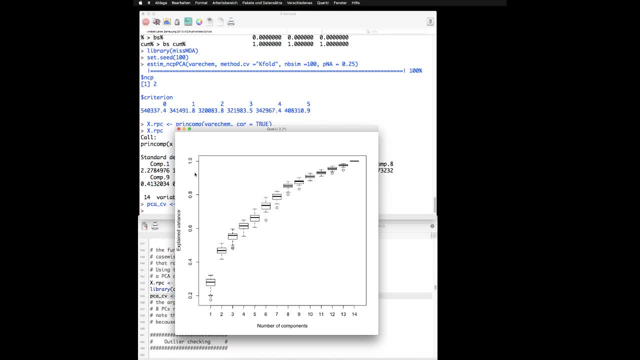 So we Calculate PCA here. What we obtain is this block. So you see the number of components included in the model against the total. then we have a total amount of variance. they ask where? and is obviously one. so you see here that we have a slight decrease and you could base your choice. 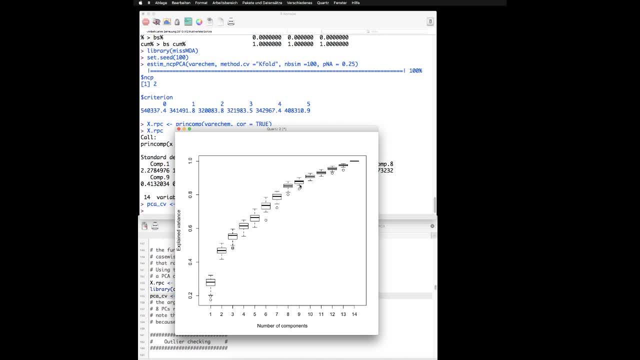 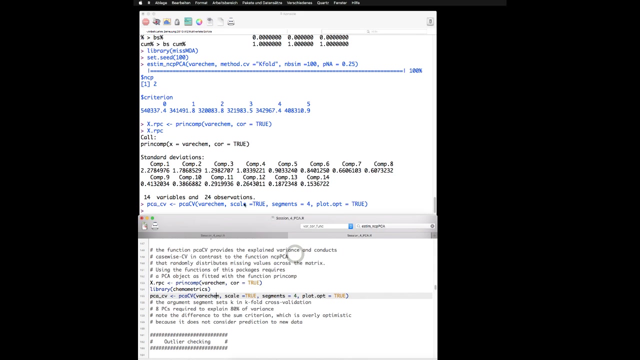 if you, if you're interested in prediction, you can base your choice on this graph as well and see how many variants we have explained. when we, when we said, when we decide on the chosen number of components, other elements of this function. scale equals truth. also same information as we discussed for 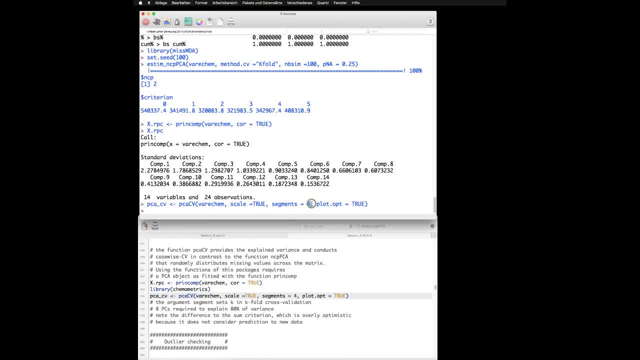 RDA. we have the segments function. segments means here number of number, of k-fold, so it's four-fold cross-validation, as in the previous function, and we have the argument plot dot opt equals true, which means that we plot the resulting, we plot the results. so when you use this function, know it that it. 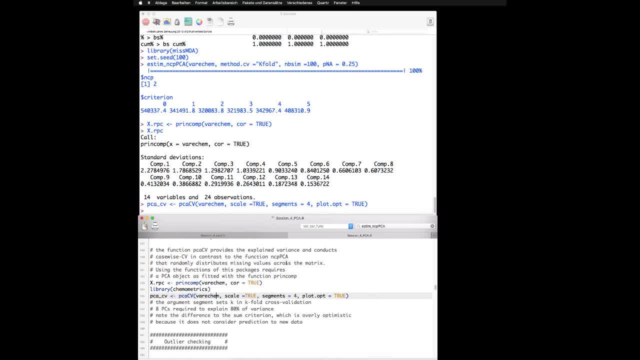 has a little bit different. why a strategy of conducting the cross validation? whereas in the previous function we randomly randomly nullified or set missing values and 25 percent of the matrix values, here we. this works much faster because we just take 25 percent of the rows and exclude them in the fitting of the PCA and then predict them all. 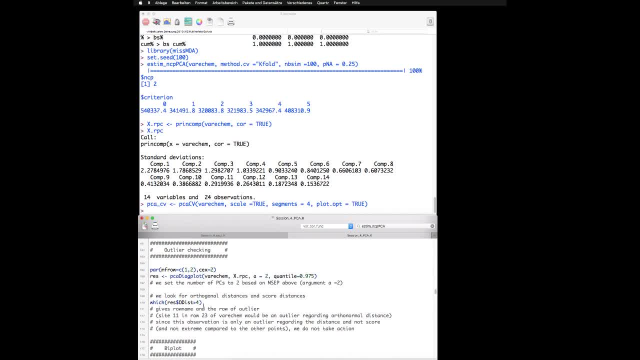 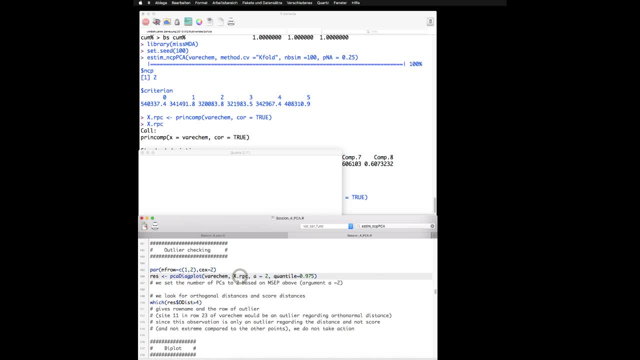 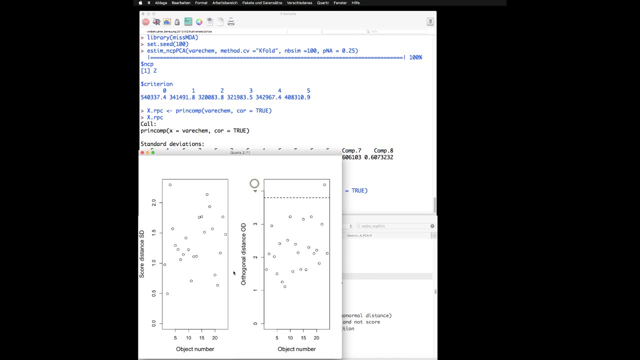 together. so we do the outlier. checking with the discussed this before. Select here a quantile of 79%. You see here the score distance and the orthogonal distance. We see, based on the orthogonal distance, we have one outlier. However, this outlier is not at the same time, does not have a large score distance, so we don't. 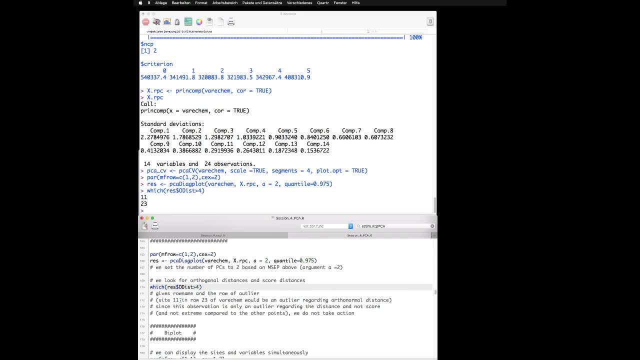 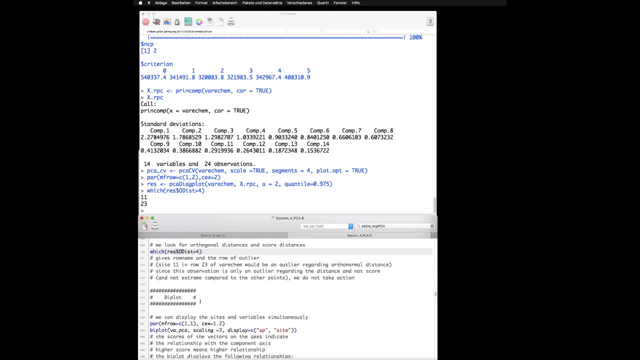 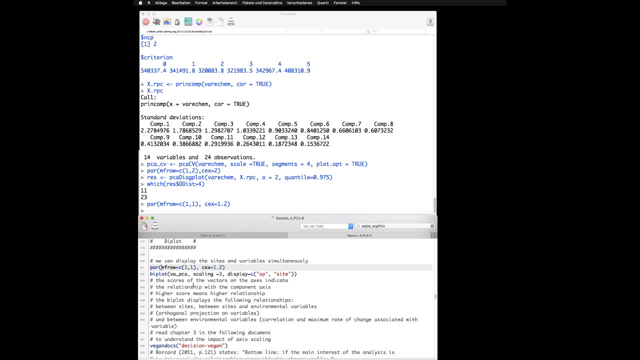 worry much more about this point. It's a side 11, row 23, and we have discussed outliers in the lecture. So we can now plot a B-plot, Set the variables back to the argument we set before, Set the plot window back to one plot per window, Then we plot the B-plot. I'm not going into. 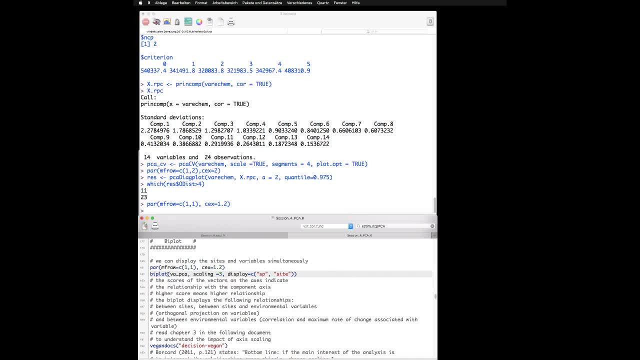 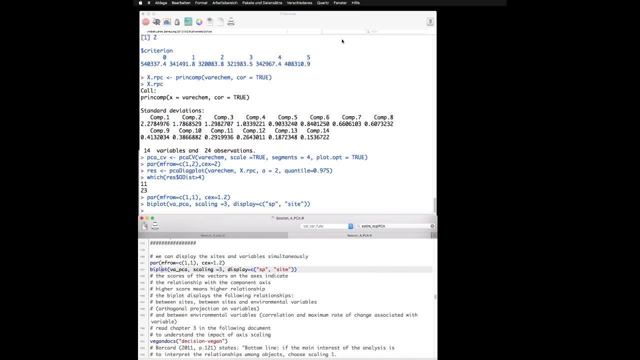 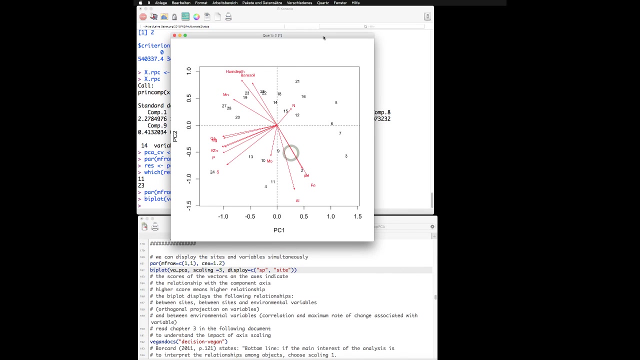 details here on the scaling in B-plots That is discussed below regarding the axis scaling the vegan documents, and you should execute this and load and read through The documentation for this package. So we plot the B-plot. So now we have a plot that shows you again relationships between the sides. We've already 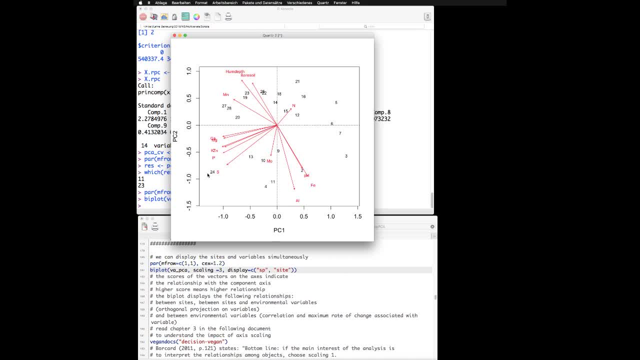 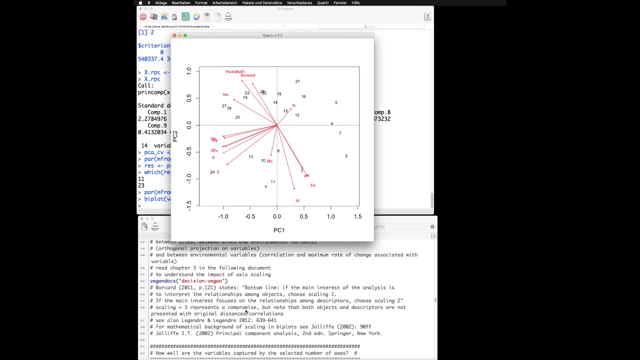 seen that before, And apart from looking at the relationship between sides, we can also look now at the correlation between correlations. So, for example, if we have a plot like this in B2, 32. To this side, and then we can assume that the value is correct here in B2, then we can 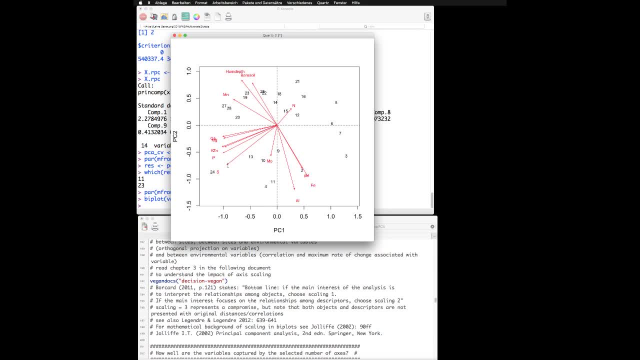 also assume that this is the same as in B3. Here we will interpret the plot like this, So you can see into this direction. And the same is the interpretation for the other arrows. If we look at the angle between arrows, then you can read the correlation. So if you 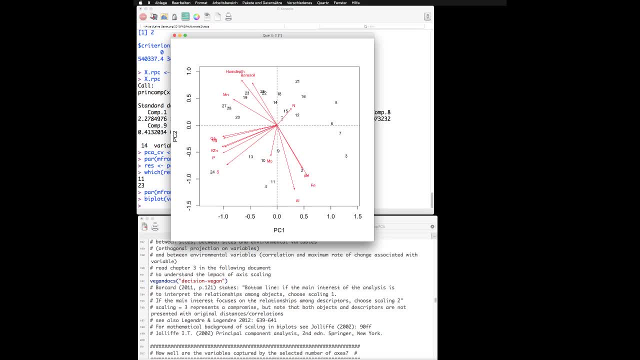 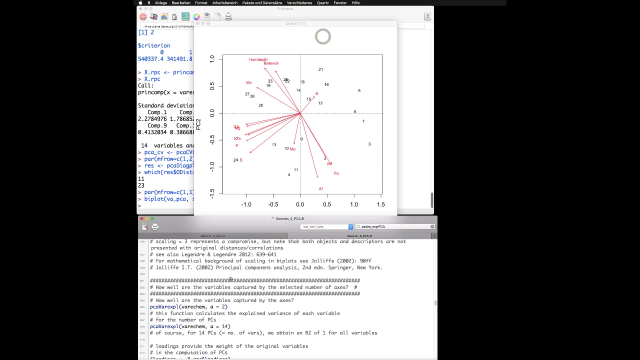 have a 90 degree angle, that is basically zero correlation. If you have completely opposite arrows, that means that your correlation is more or less minus one and all other results between that. Yes, after we have now inspected the plot, we will deal more formally with the questions, such as the choice of the. 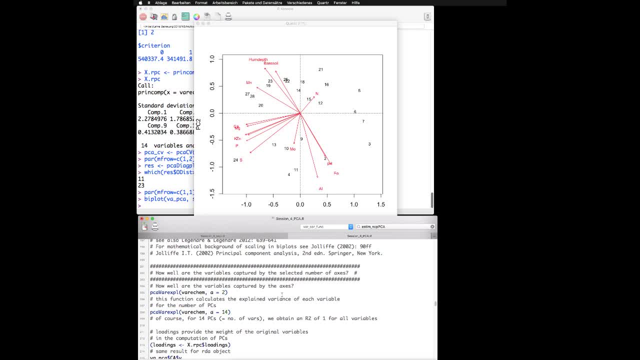 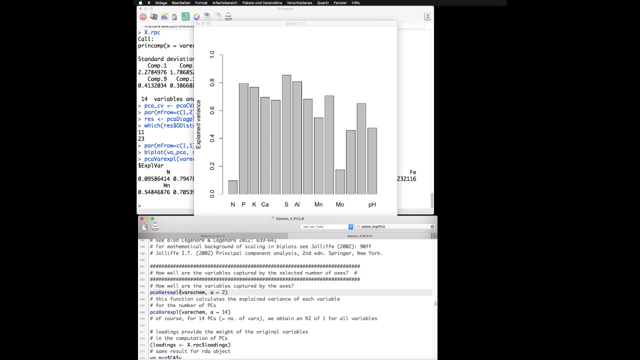 number of axes. Now we've done this already. we will have to deal with the question of the variables, how they load on the axis and you can calculate the explained variance for different variables with this PCA, var explain function and that shows you which the amount of explained variance of the different. 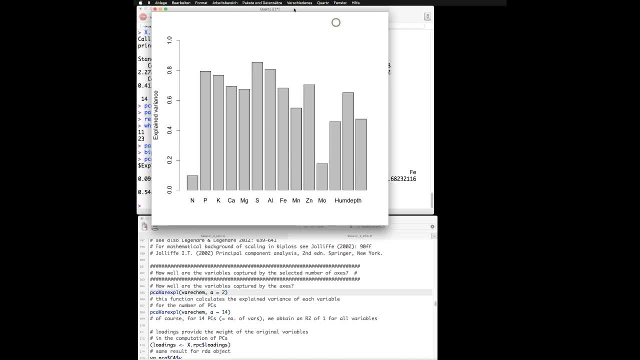 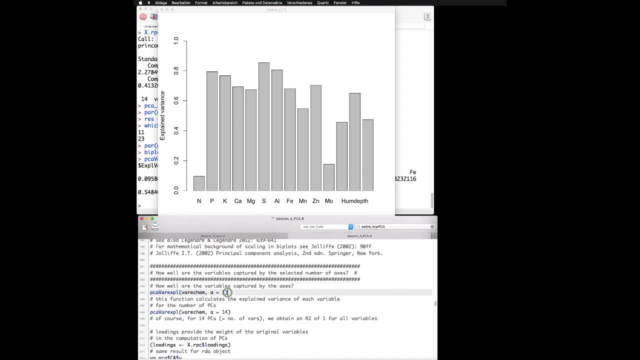 variables for two principal components. You could also do this. the a indicates the number of total principal components used, so you would see here which variables have the most variables. The highest contribution to the first principal component Can't do this…. The univitchable axis is always the cumulative r-square on all on. 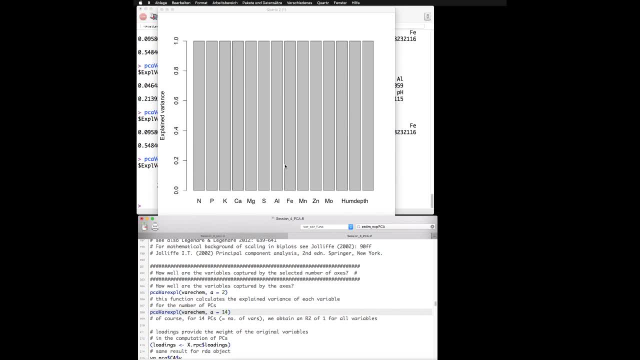 the axis. Obviously, if you choose 14 principal components, then you have an r-square of each for each of the variables, because, overall we explained, this is the total instrumental amount, total variance in the data set that is explained by the 14 variables that we had initially. 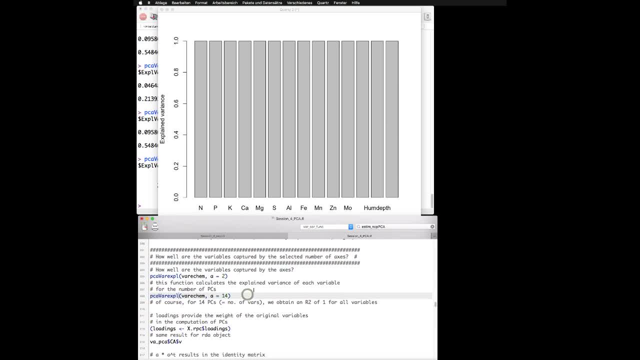 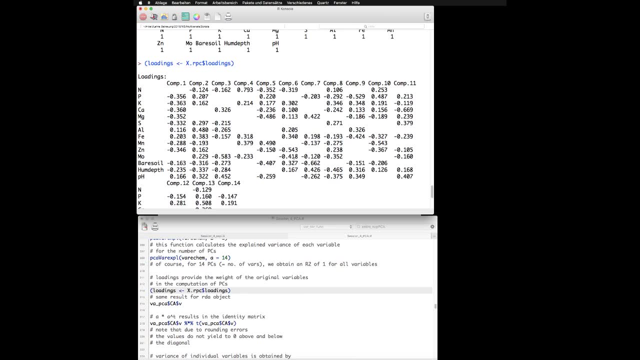 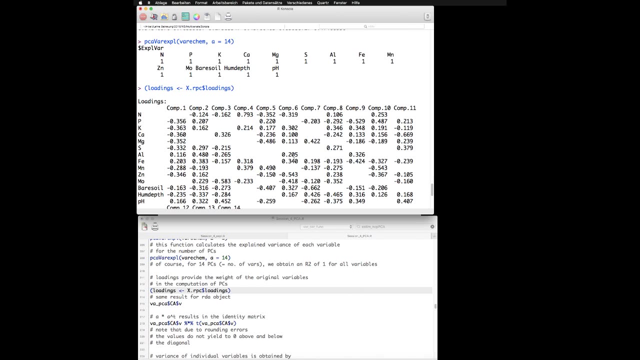 and now we have 14 principal components. If we want to look at the loadings- and just a note of caution, loadings are interpreted here in R loadings indicate the eigenvectors, whereas in different contexts they may indicate what we consider in R as correlation loadings, so the correlation of the original variables. 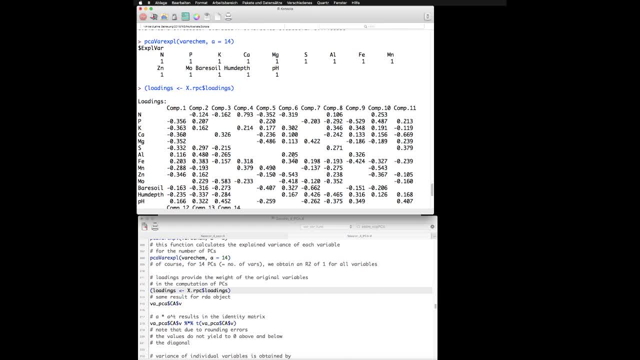 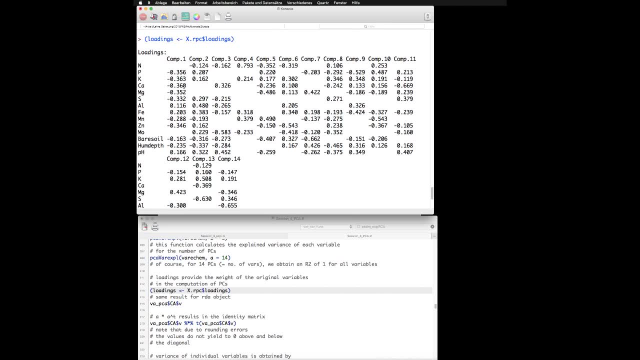 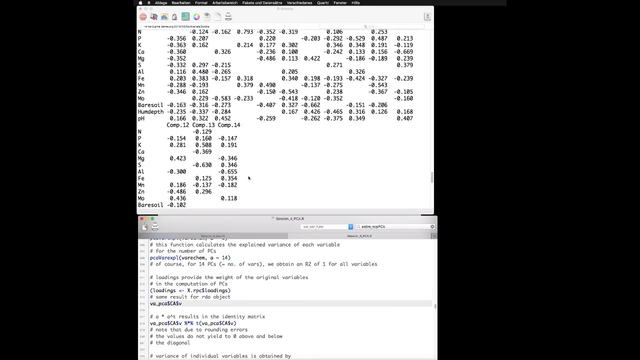 with the principal component axis. You see for this object loadings, only the loadings above a certain threshold- 0.1 I assume- are displayed. the other loadings are not shown. Same: You see the same for the object. this is the XRPC object that, remember, we needed. 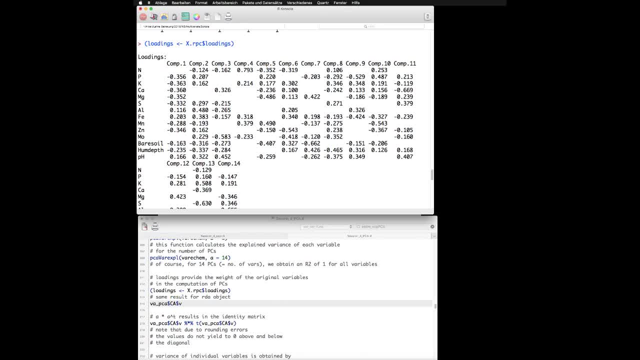 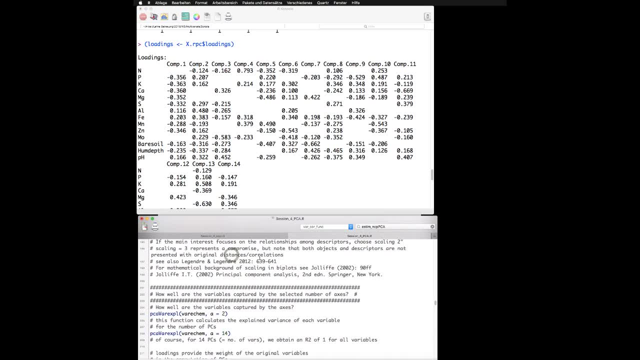 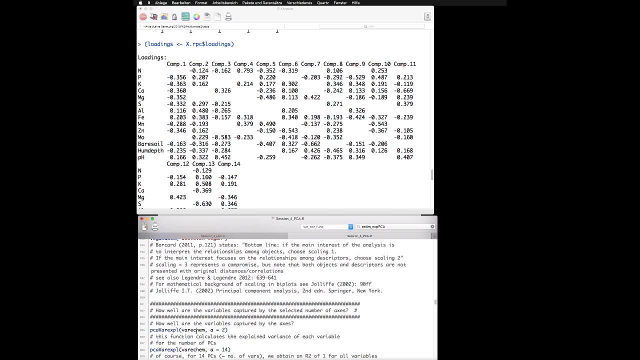 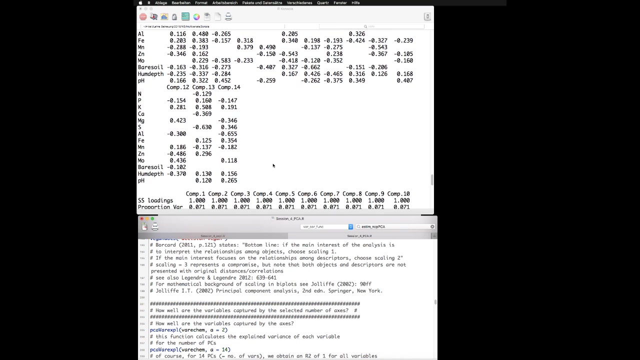 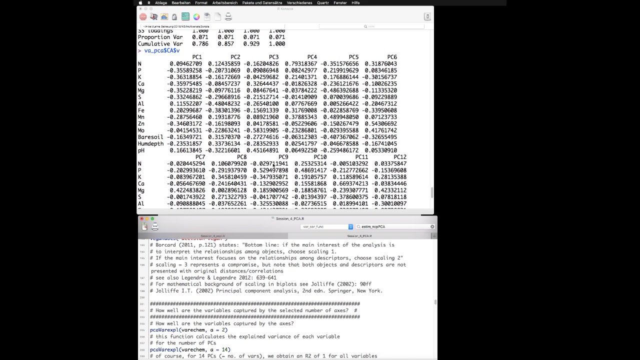 to run two different principal component analysis functions to enable the use of different analytical functions. So the analytical functions that we use for outlier checking, or PCA variance explain relies on objects. For example, we can use the RDA object for different purposes and we use this later on. 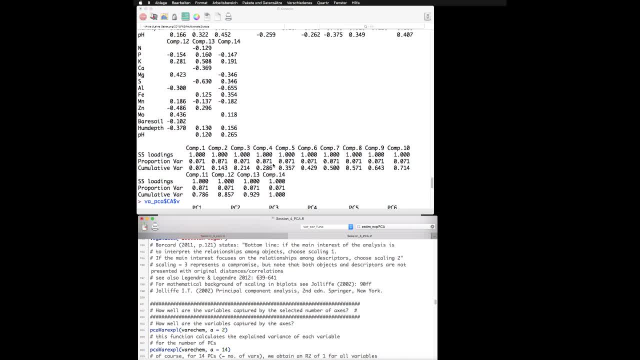 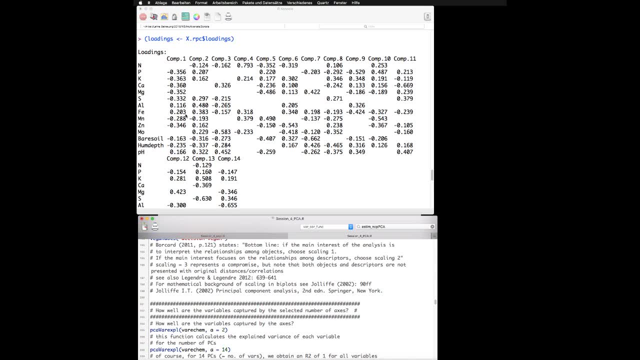 in the course, so that's why we use the RDA object here too. You see that the values, though, are the same. when you look here, the loading of phosphorus on component one is minus 35.6, and that's equivalent, or it's the same as here. 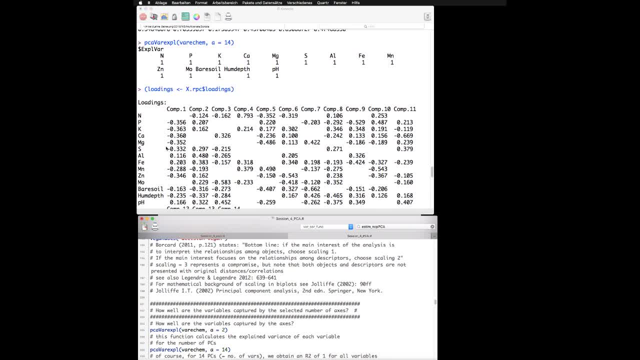 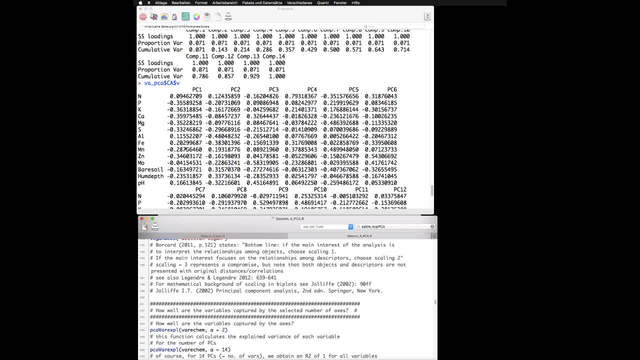 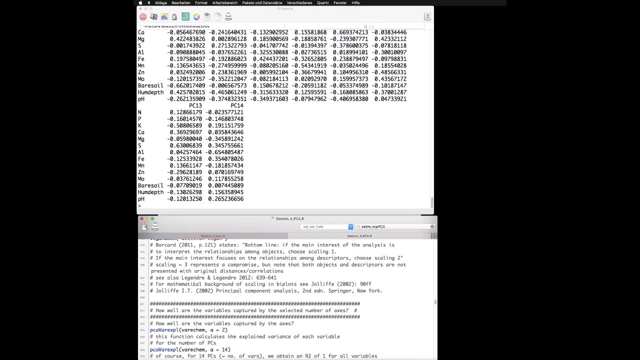 It's just rounded. these values are rounded values. we have another value, that's- let's check another- for aluminium, 0.116, so this is rounded. these are rounded values. You see that we obtain the same results for both functions. 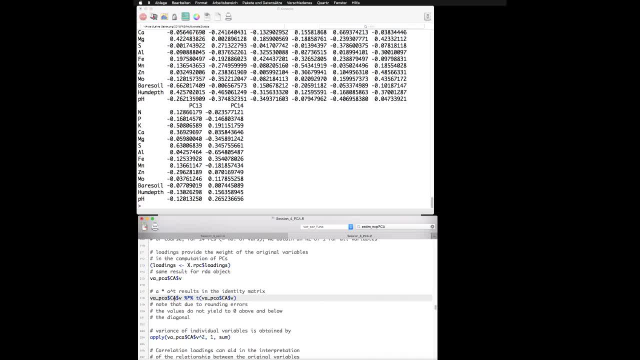 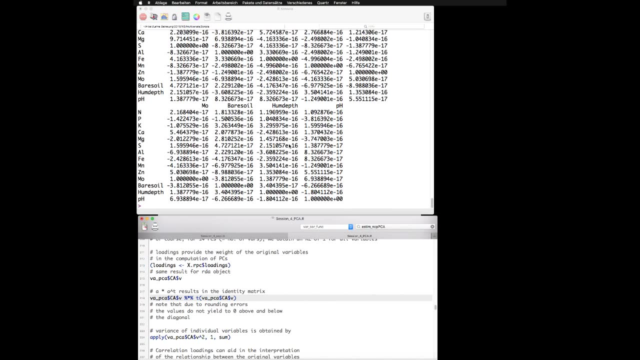 We can also check that. we know that one of the conditions in the principal component analysis is dead. So we can say if we use the RDA object here, we actually know that there is still a dead product. In the case of the RDA object I can say that now I can return the product and see. 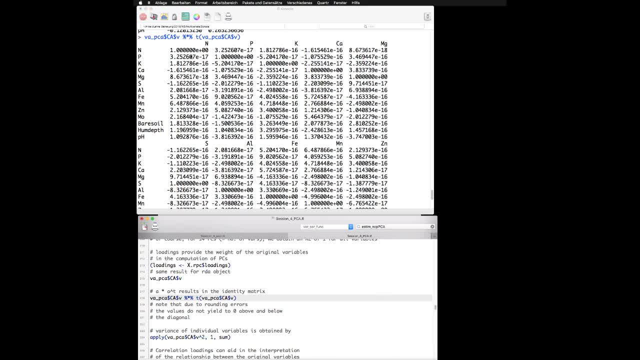 that I have to return the product. In the case of the RDA object the product. I can return the product. So basically, we get the same result. We can also see that the value of RDA is 0.. We can also see that the value of RDA is 1.. 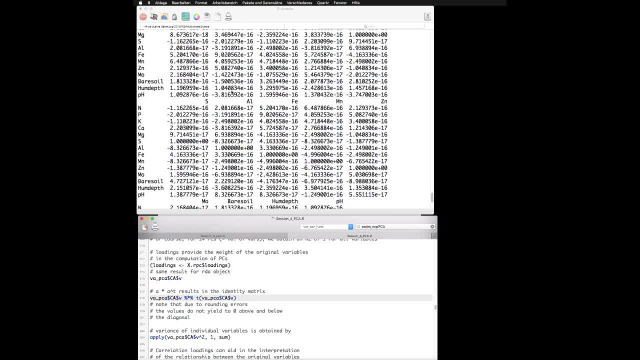 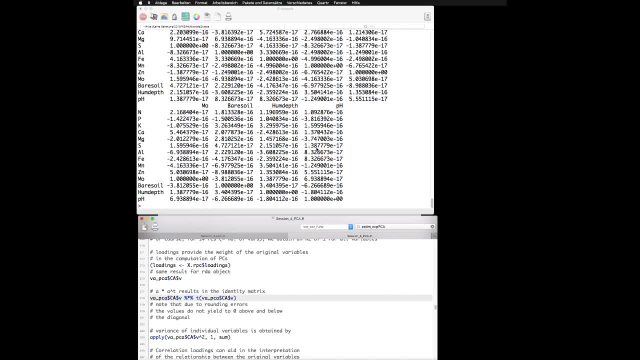 just rounding errors why it doesn't add up to zero. but basically we have zeros along the remaining cells, in the upper and lower triangles, above and below the diagonal, and, yes, because of rounding errors, that we have extremely tiny values, that these values are not exactly zero in these, in these cells, we can't compute the variance of individual variables again. 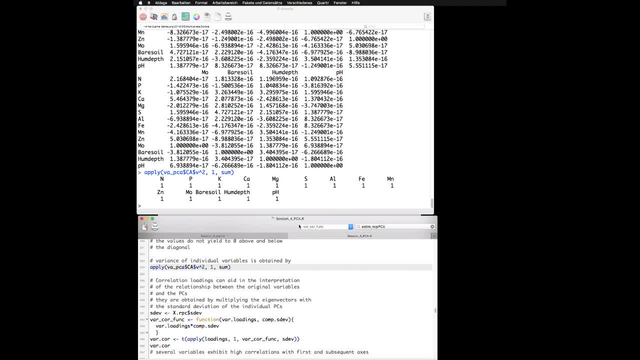 that's not surprising that we have here all variances. of all the virtual variances is one. and then we, I provide you with a function. I just took this function from the internet and I'm going to show you how to do that in just a moment. and then I'm going to show you how to. 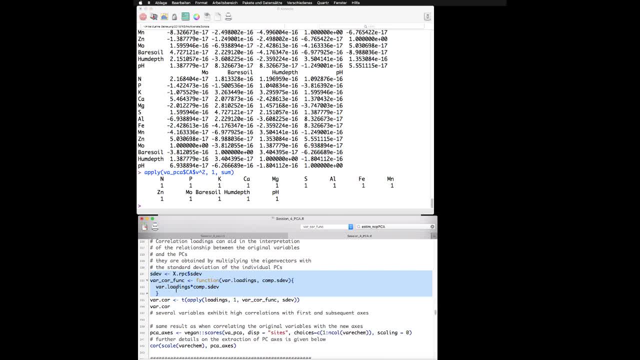 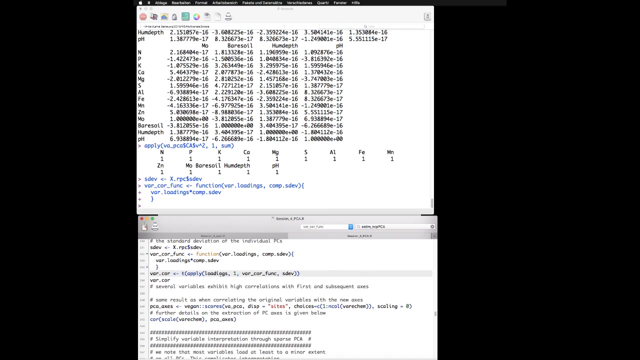 do that in just a moment, and then I'm going to show you how to do that in just a moment from a website. that's a convenient wrapper to calculate the variable loading. so this function just multiplies the loadings with with the standard deviation of the eigenvalues. so we apply to the loadings we, and one just means that we do this column. 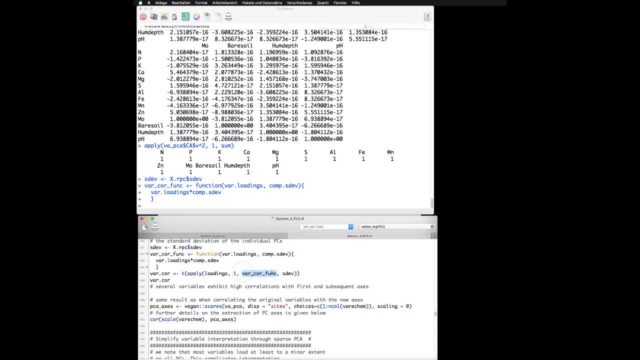 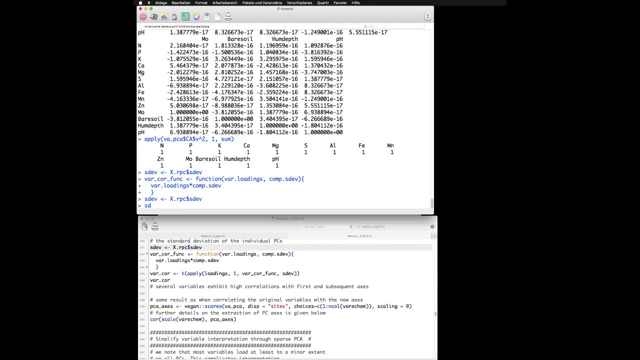 likewise, we apply the function that we have just defined here and use as input the standard deviation from the object. just another deviation we assign here as a standard deviation. just have a quick look. these are the standard deviation of the eigenvalues for each of the principal components. 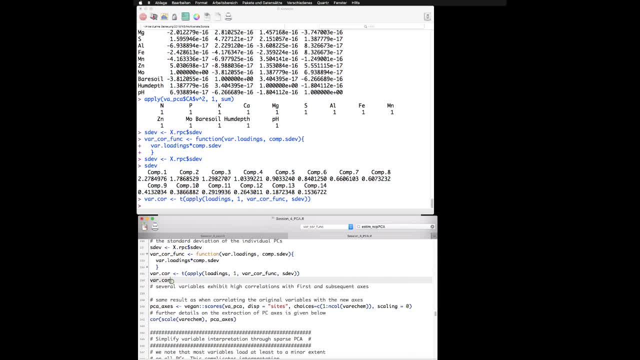 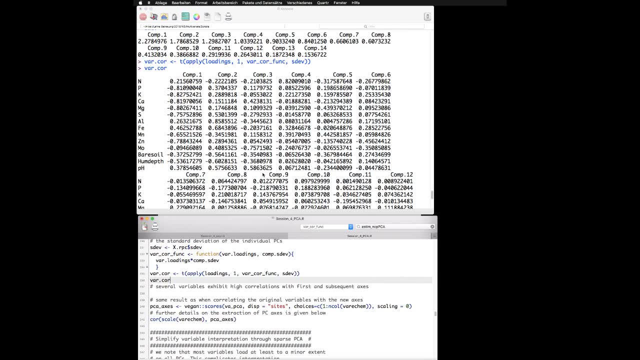 so we run the function and now we have three DEVIATIONCOM For each the principal components. so we run the function and now we have more easily interpretable results. We see that the component 1, we have different variables that have a high correlation with this component. for 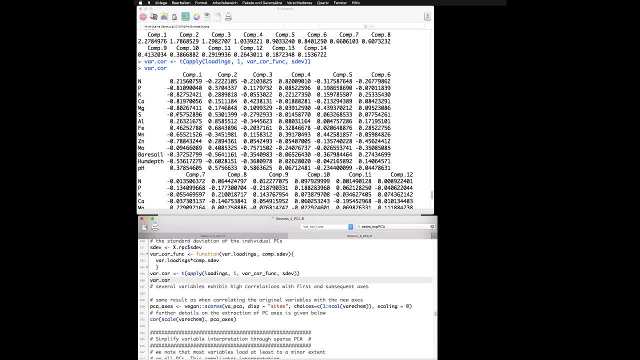 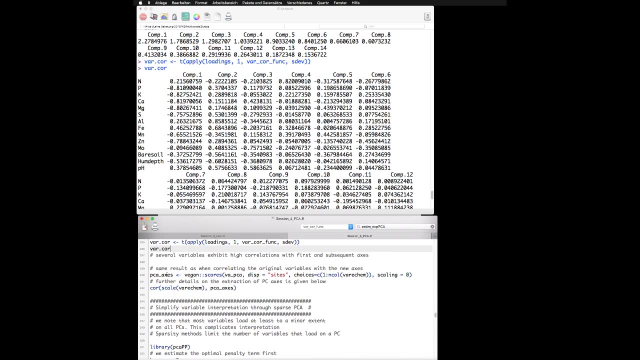 example pKa- calcium, magnesium, sulfur, zinc- They have all correlation coefficients above 0.75, so they have a definitely high correlation. We can check that this is true by extracting scores from the pKa. So the side scores, the principal component scores we've discussed in the 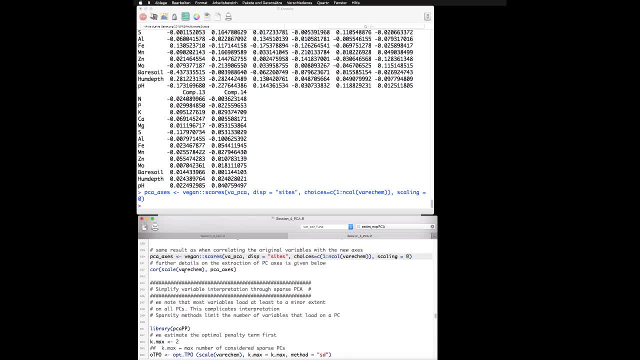 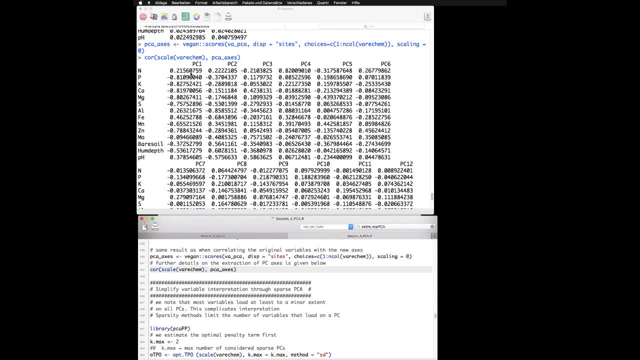 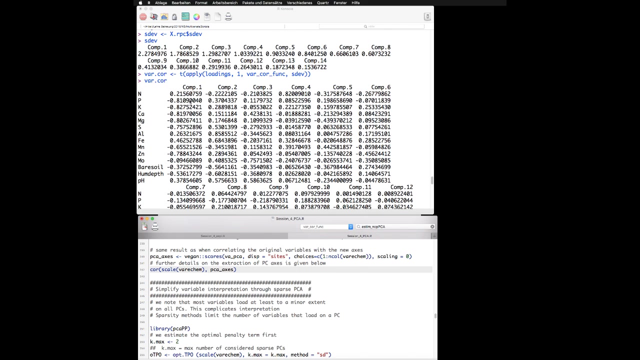 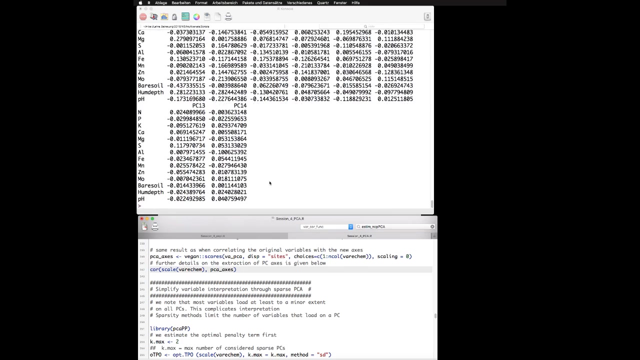 lecture. See here how you extract them in R and when we correlate now the scaled variables And actually we'll look at the scores Just to show a bit how we get power. So we have the double Santiago And in this slide face this square group with the table八. 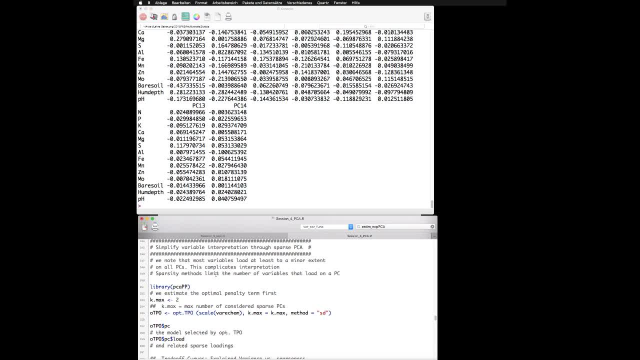 And now we get some vêie representing the data In the first two slides where we got more points. This is what we have came to demand for the original elements. We are now looking at be cutting up the meals and the data In the context. we began discussing in the context of multiple regression analysis and we discussed also for PCA. 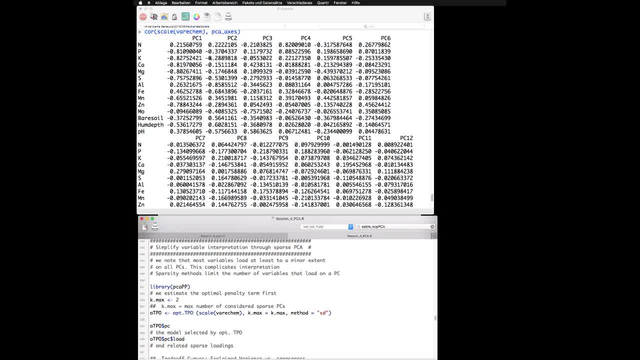 As you can see here. if we look now at the correlation coefficients, we see that we have many variables that are associated and have a correlation with the first principal component, And that doesn't make interpretation very simple. So ideally we would limit the influence of variables with low correlation on the individual principal components and just have a few variables that have a higher correlation. 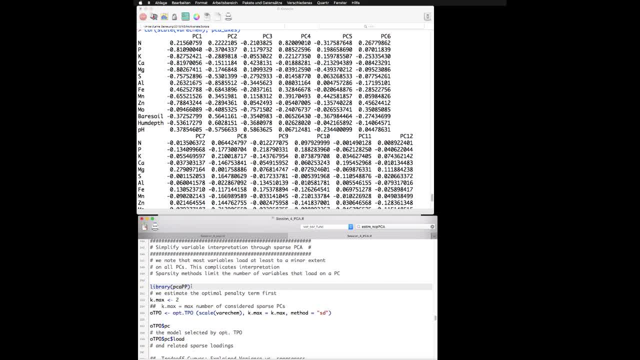 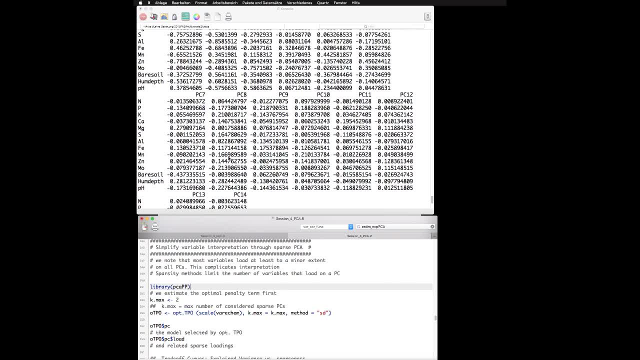 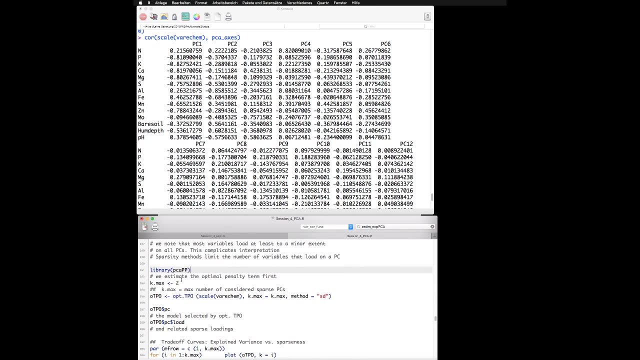 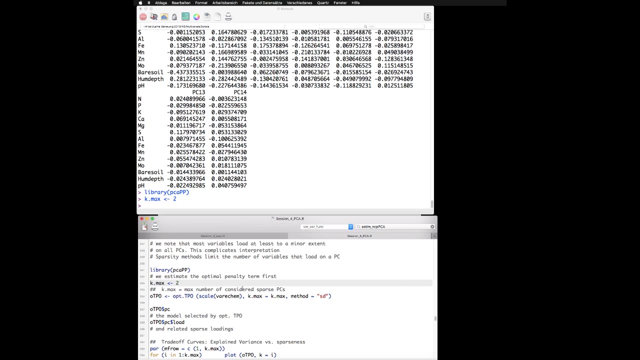 And we can run so-called sparse PCA where we put a penalty term on these variables, On the eigenvector values, on the loadings, on the axis. this has been shown in the lecture. First, as you know from the lasso, we need to find the optimal penalty term. 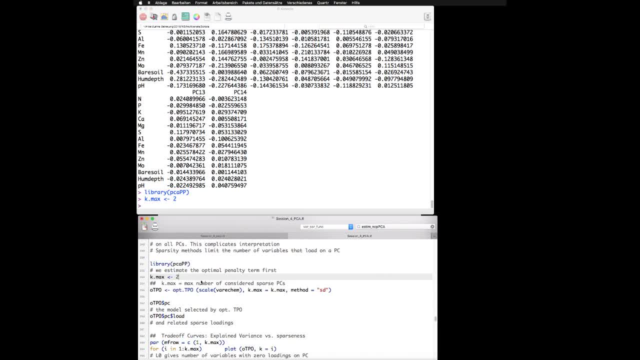 This is done here with an objective function. I'm not going into technical details here. What we provide to this function is: on the one hand, we scale our data. Let me just go ahead. We discussed this before. We need to have the same variance in the different variables. 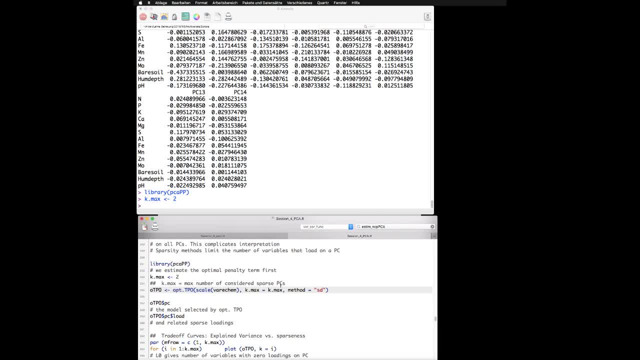 Kmax means it's the maximum number of considered sparse PCs. We have identified two principal components as being ideal before, so we provide kmax equals true, And then we provide here a method that is used to estimate the variance. That's here the standard deviation. 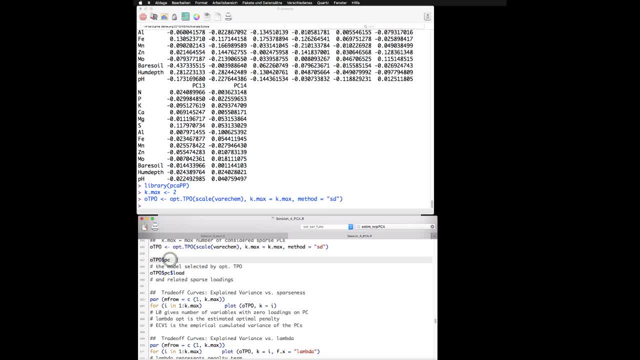 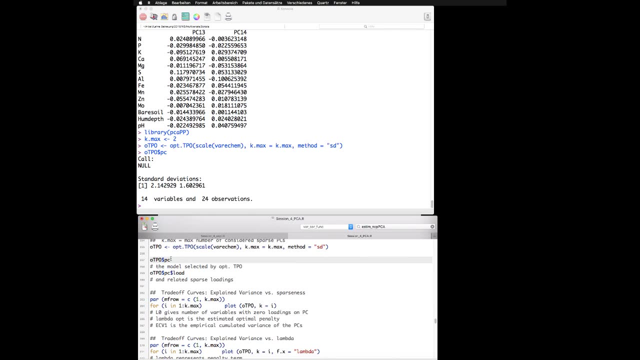 Yeah, have a look in the function for other options, for example for the methods that you could use, like the median, the multivariate median or other values. We first obtain the output. that is the same as for the principal component function. 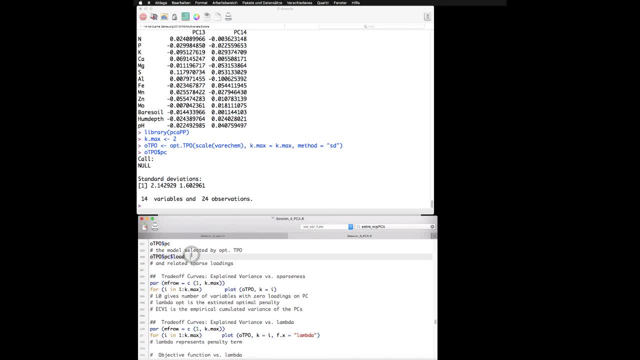 We see here that we have the eigenvector, The eigenvalues for the two axes, And then we obtain here for the optimal selected variable, we obtain the loadings on component one and component two, And we see that now the loadings for seven of the variables have been. 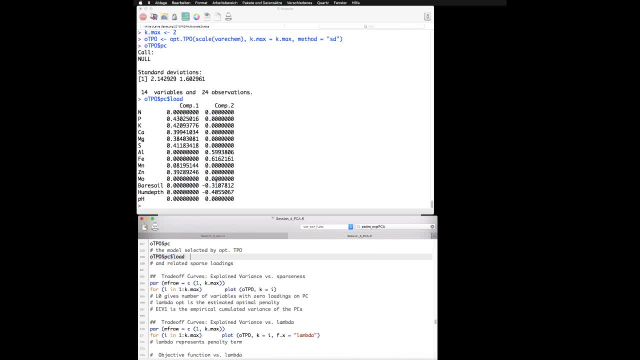 reduced to zero And the loadings on component two- actually most of them- have been reduced to zero, So it's much easier now to compare component two, which is mainly a gradient and axis of aluminium and iron and has a negative correlation with bare-soled and humous-steel. 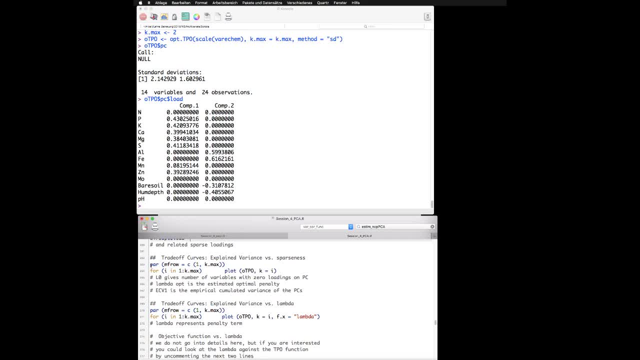 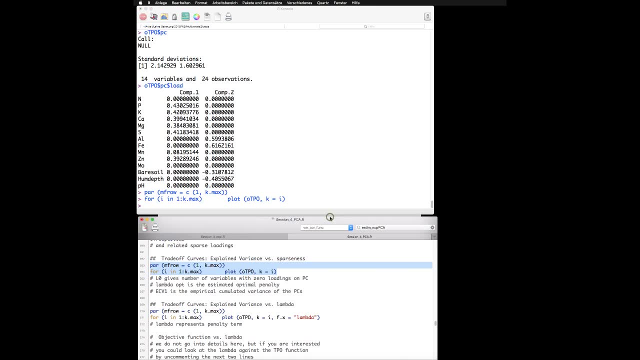 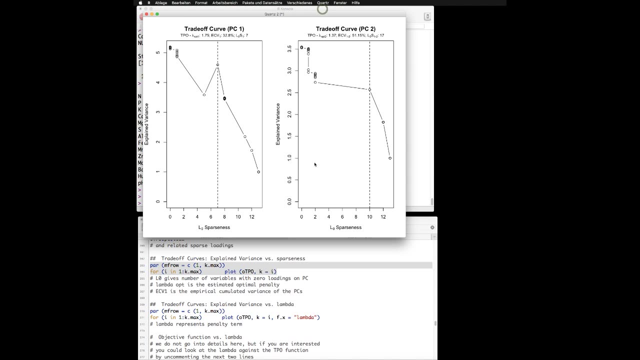 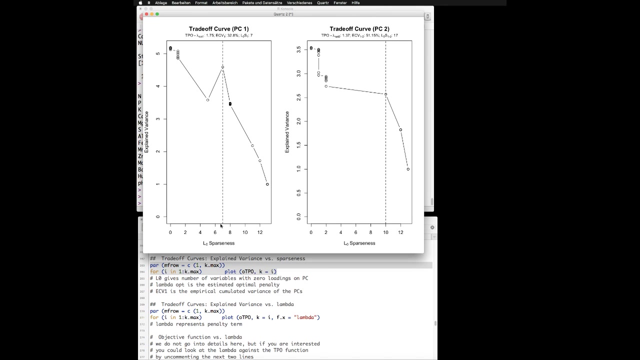 So the choice for the selection of this optimal value we can have in the one- riches function we can have. we could look at different plots. so first plot here is for each of the principal components. we see the explained variance against the sparseness. 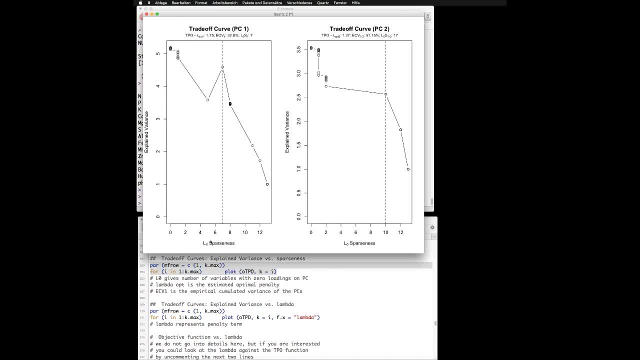 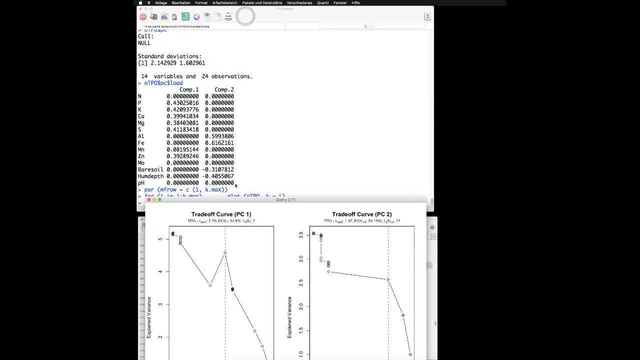 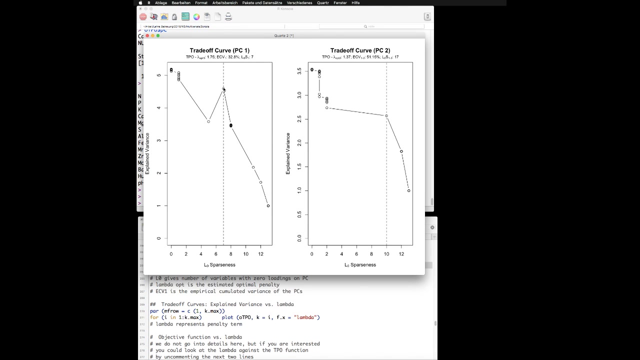 that means the number of components that have that have a value of zero. where the, where the loadings are zero, we see way and we have- and that's actually the selection that we, which we see- we have seven of the loadings for the descriptors that are zero, then we reach an optimal value and we obtain the value. 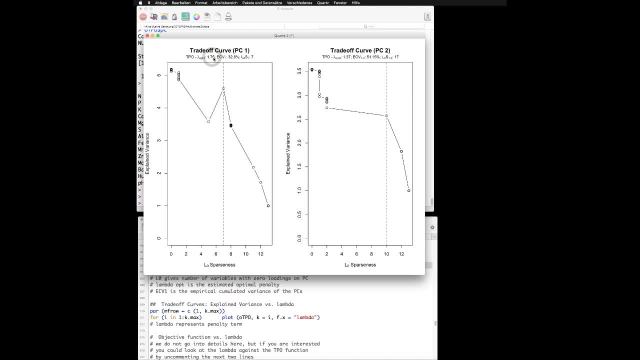 for lambda, that's the penalty term. here we obtain a value of 1.75. we see here the estimated cross-validation error. we see as well the number again here, the number of component of descriptors that are contained or that are zero, and this is here given for. this is given here for the optimal value of lambda, for the. 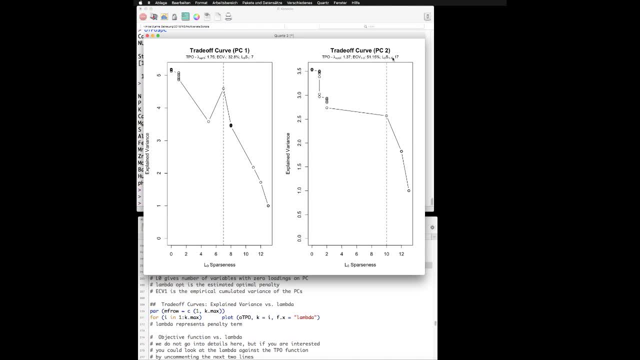 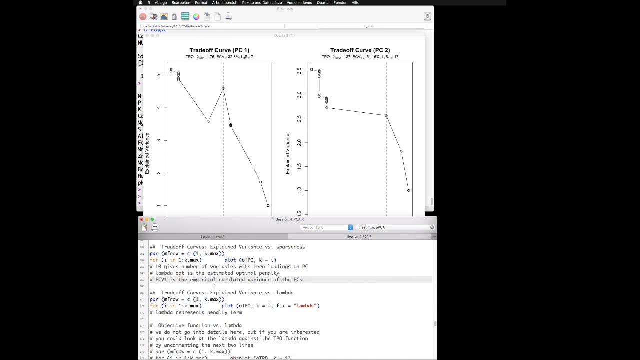 second axis and we have here the both. this is for both axis together, for the both, for the two first two principal components. now, excuse me, and it's not the cross-validation error is of course the accumulated variance of the PCs. it's here 20, 32 percent. for the. 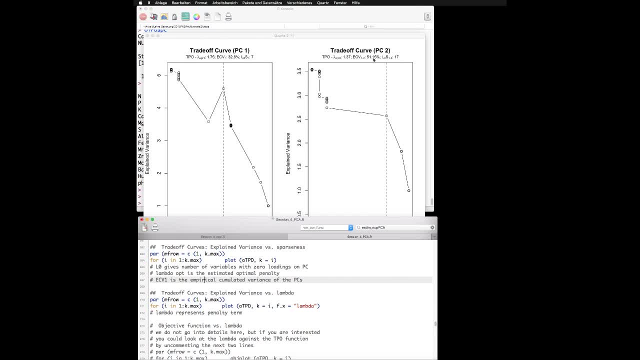 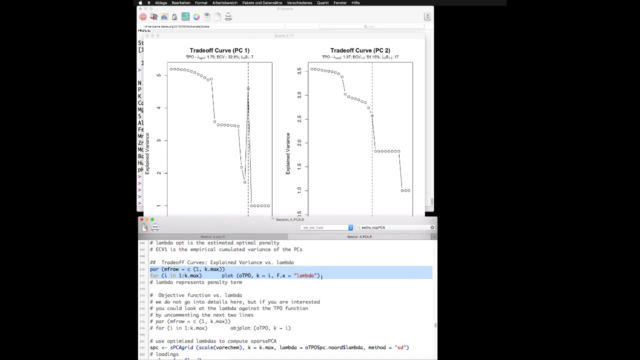 first axis for the first principal component, and here 52 percent or 51 percent is explained. if you check the both, the first two axes, we can also plot lambda directly. so we see here for choices of different lambda, we see the development of the explained variance of. 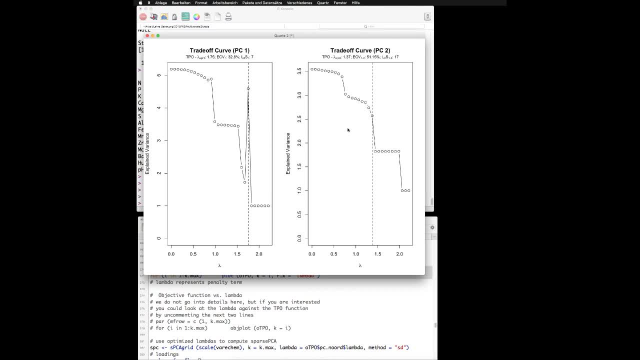 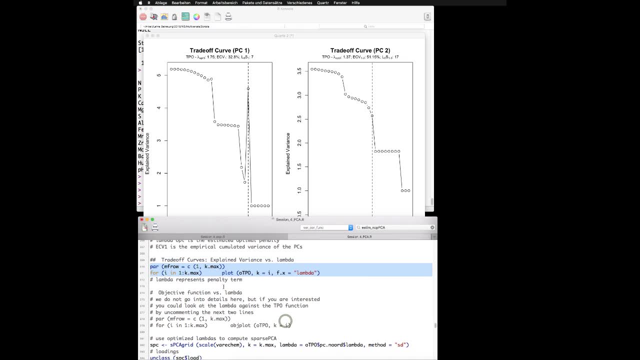 the in the first axis and we see the same for the second axis, and the optimal choice based on the objective function, and you could look at different details. now we use these optimized lambda in the SPCA grid function to compute the sparse PCA, an object which we can use. then we have some more. 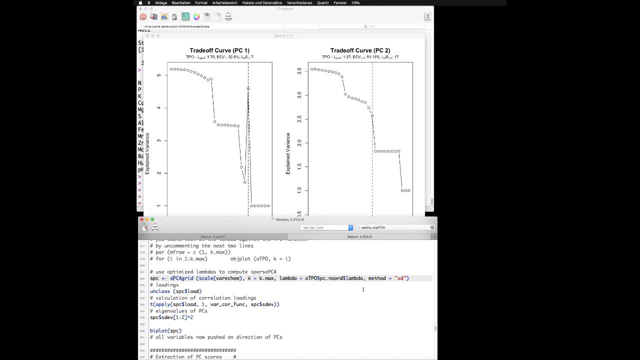 information contained in this object. you see that compared to the, to the optimizing optimization function, we provide here the lambda as well and we extract from this object the lambdas. we abstract the lambdas from this object that we defined before, save this in the object spca. 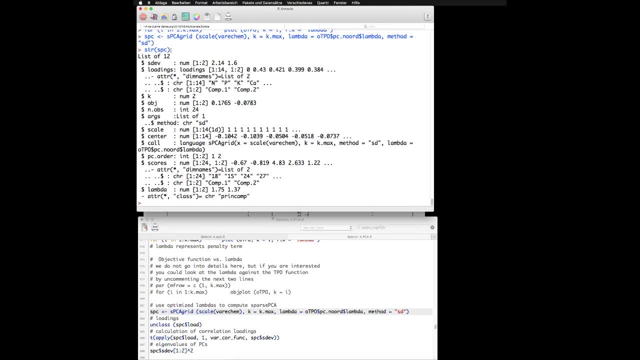 if we have a look into this object, we see it's a object that has 12 different attributes. you see standard deviation for the two axes we have defined, two axes are fitted and we have several other information given and we have, for example, the scores given here and the class of this object is principal component object. 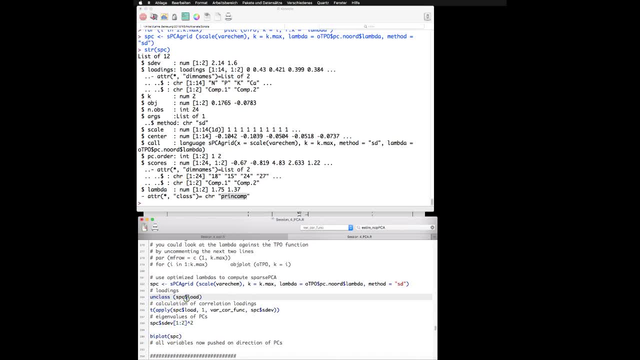 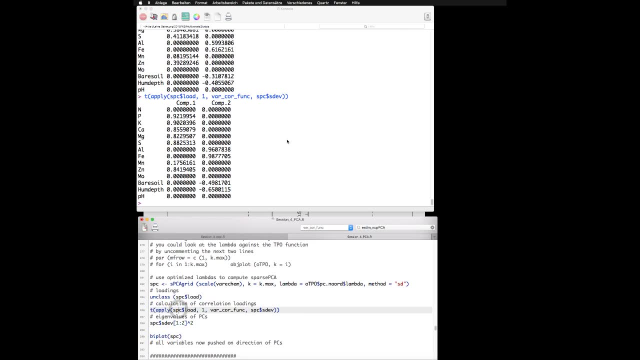 that's similar to an object from principal component, from the class principal component. we have a look at the loadings, we can again compute the correlation and we see that through the sparsity function we have actually an increase in the correlation with some of the variables. so before we had 0.8, now we have 0.92 for the variables phosphorus, calium, calcium. 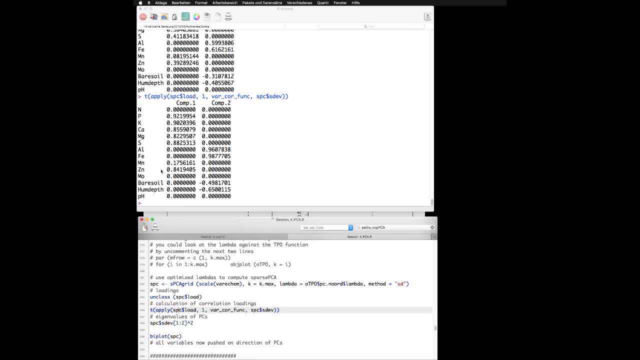 magnesium and sulfur and manganese and zinc. manganese has a low value, so if we would choose a low, a higher lambda than manganese, this would be a very high correlation with the component one and it would not load any more on this component. and we see by contrast again that now component two is really a very strong. 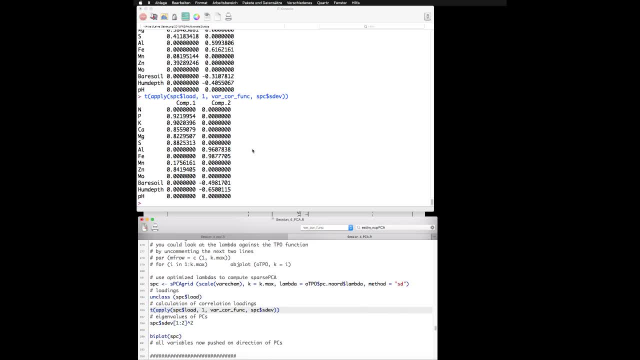 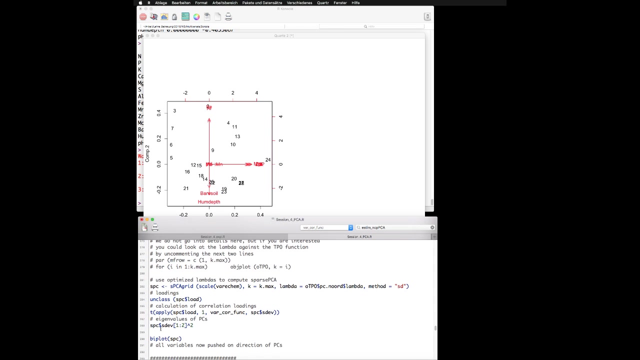 aluminium and iron has a really high correlation with aluminium and iron. you also see, uh, when we use this this, that none of the variables that has a high correlation with component one or two has component, and that means they are more or less orthogonal. This can be seen when we calculate a bplot. in fact, we should put back the graphic window. 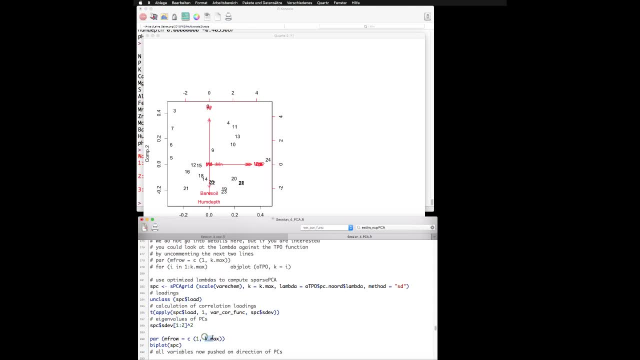 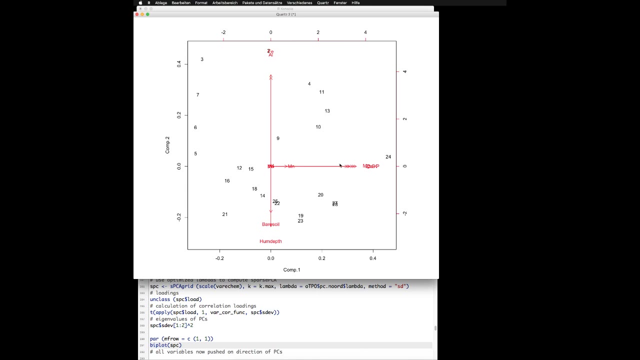 to default with just one plot for a graphic window. that's done with this function If we plot this so first this looks a little bit strange. now you have all variables plotted really in the same direction as the principal components, but it's somehow clear because 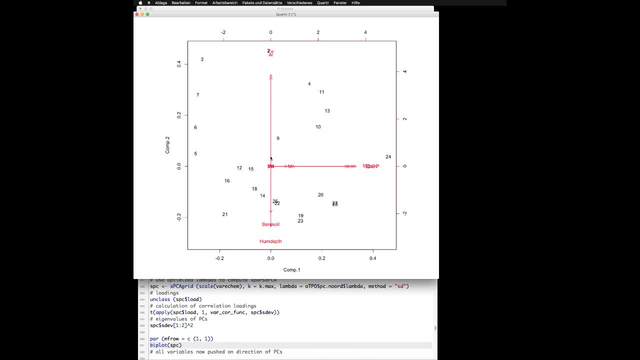 we have now only correlations with. if you had the error like that, it would also slightly correlate with the other principal component, and since we see that the correlations are now zero For the four variables with the component one, then of course it is just parallel to. 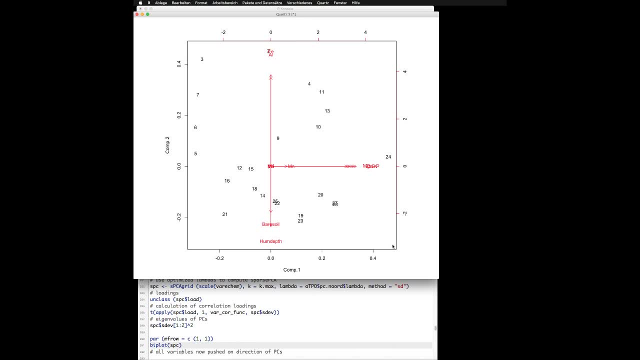 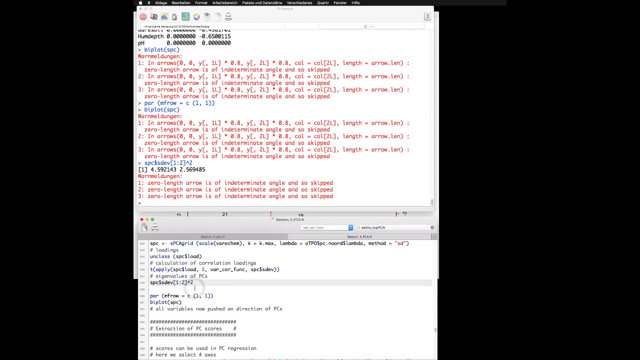 the first or second component. It's not really easy to read in the bplot now because all the variables that have relatively high correlation with the principal component are plotted on top of each other. And finally you could check the eigenvalues again, and it's done like that. 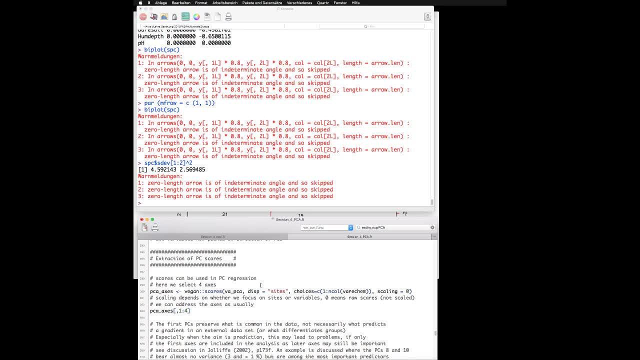 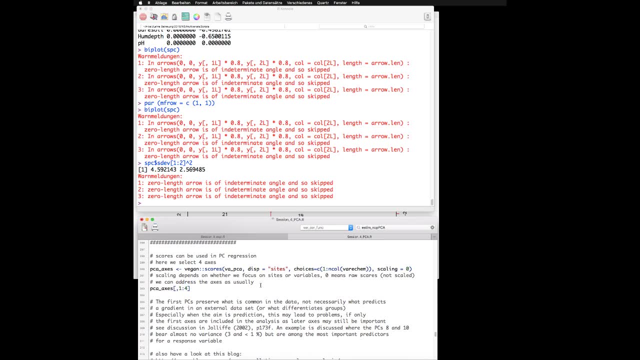 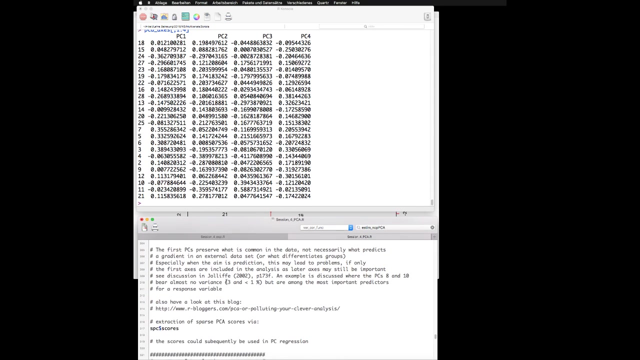 The final issue is we could extract the principal component scores if we wanted to run a principal component recursion. that's shown in this part of the script. just quickly, you can extract the scores from the vegan package from the object using the bplot, This function. so we obtain here the scores from the first four axes and for the other. 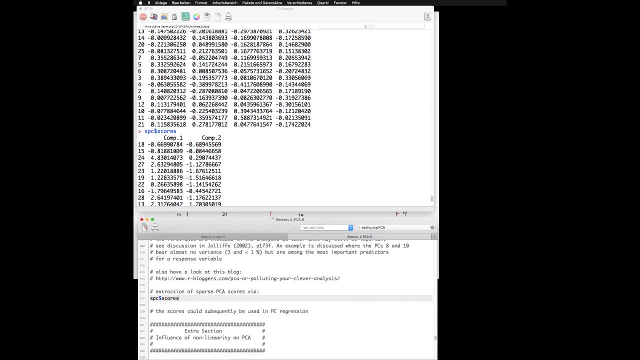 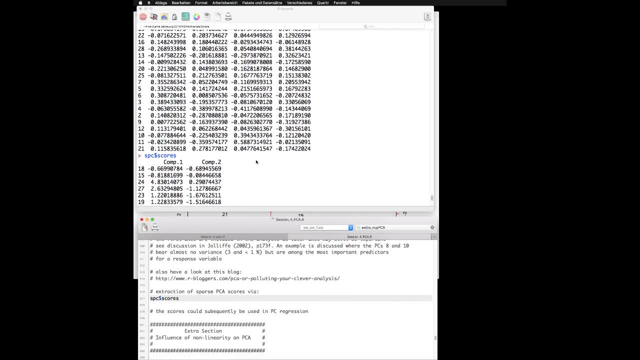 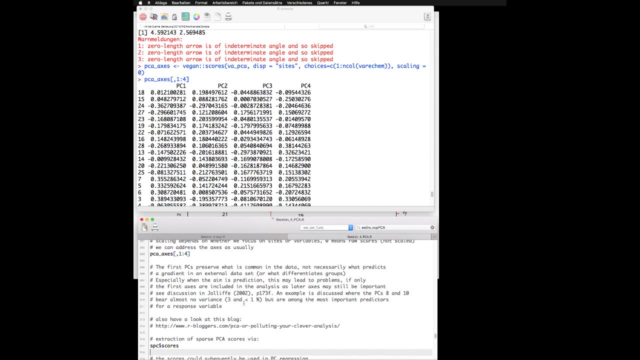 object from the sparse PCA. this could be done here with the scores in the scores attribute of this object, fairly simple. You see here a little bit more text. a core note of caution on principal component regression and on the choice on the number of variables and axes to use in the principal component. 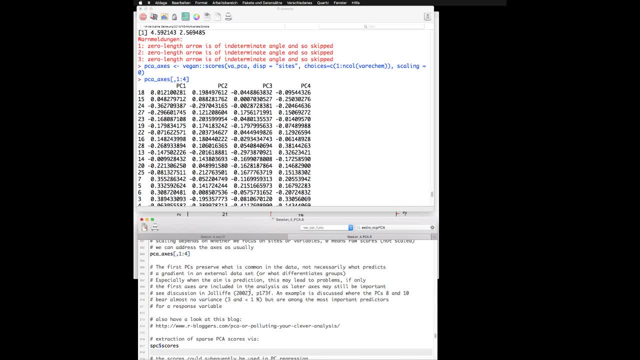 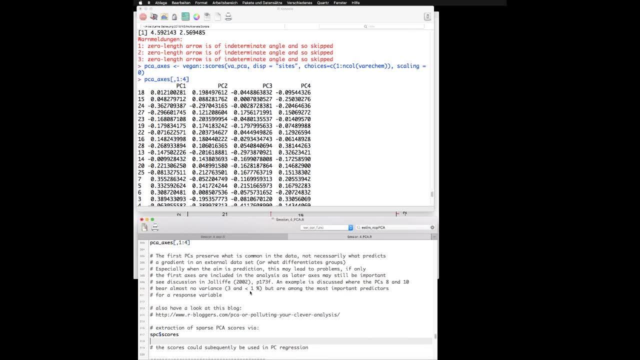 regression and so on, But it's discussed more theoretically in the lecture as well, so I don't go into details here. you can just read this yourself, And I have an extra section for those that want to look a little more into it, where 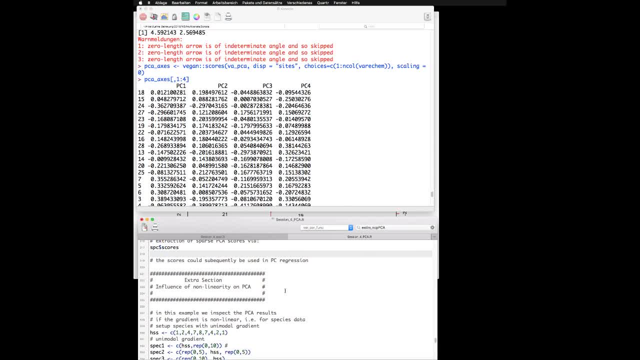 I'll show you how, How non-linearity influences the principal component analysis and why different ordination methods are used. And then you have the exercise, below this extra section, for those that want a little to look into more, more into depth, then you have the exercise. 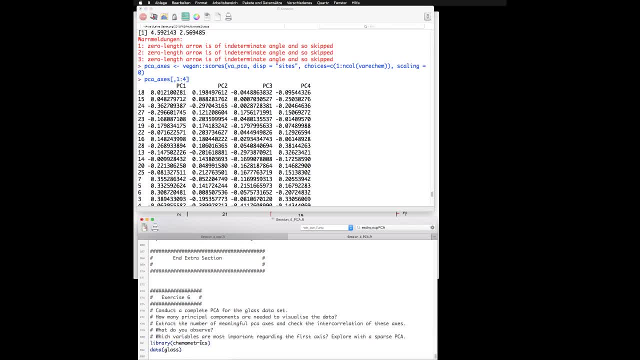 So use the class data set in the library chemometrics. conduct a PCA, decide how you want to use it. how many principal components are needed to visualize the data, extract the number of meaningful PCA axes and check the inter-correlation of the principal component? principal components. 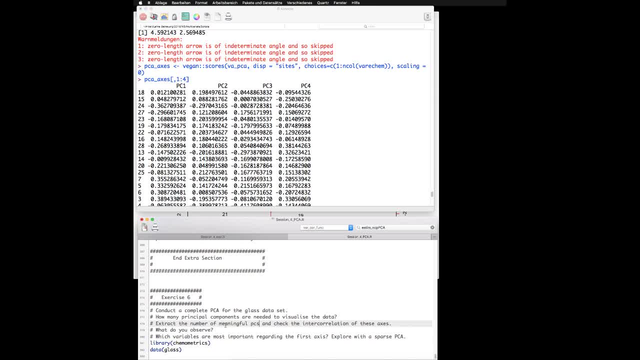 Check the inter-correlation of these axes, what you think, what you could also already formulate an assumption of the correlation between these axes, Um, And then have a look Which variables are most important for the first axis and explore and redo the analysis. 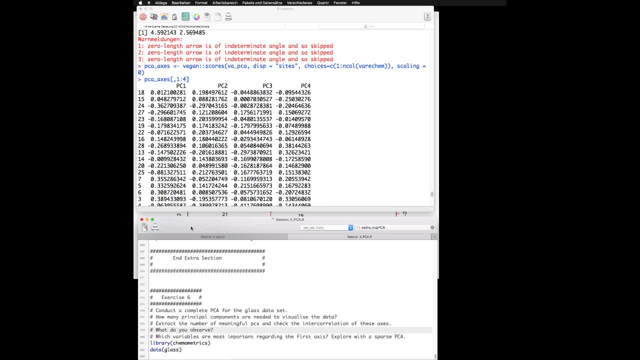 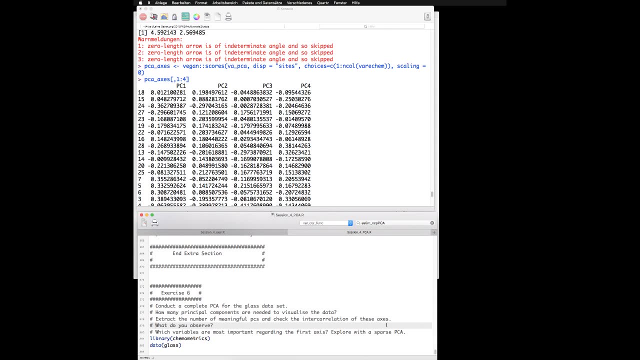 as sparse PCA. That's it. I hope you learned a little bit about PCA and sparse PCA and about the different implementations in R functions, how you could use them, and hope to see you in another session.